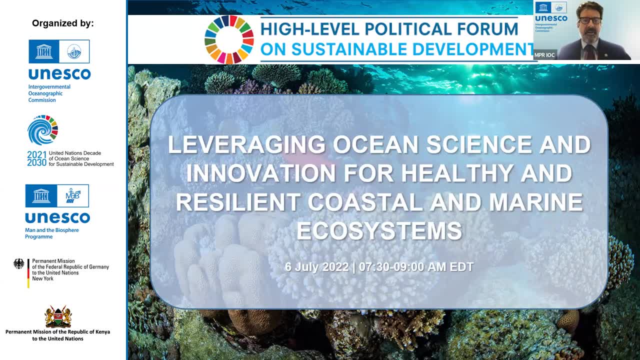 Good morning, good afternoon, good evening, wherever you are. Welcome to the side event organized by UNESCO together with the support of the Permanent Mission of Germany and Kenya, entitled Leveraging Ocean Science and Innovation for Healthy and Resilient Coastal and Marine Ecosystems. It's probably quite early in New York, 7.30, so thank you for our audience joining us. 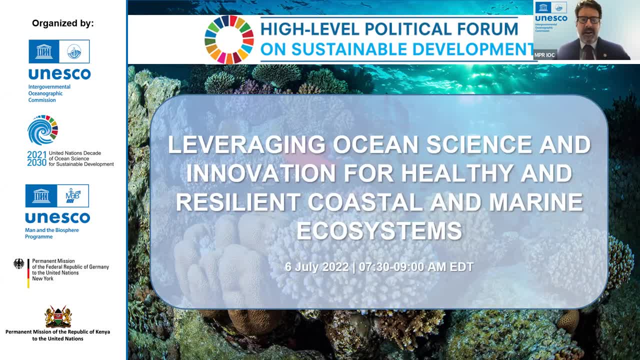 who is attending the high-level policy forum, and this event is a contribution to this high-level policy forum. My name is Julien Barbier. I'm the head of marine policy and regional coordination at the Integral Oceanographic Commission of UNESCO and also coordinator of the Ocean Decade, and I 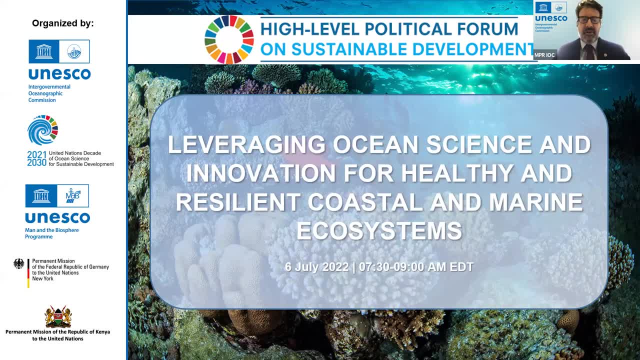 will have a pleasure to moderate this session today. So, as I'm sure some of you must know, this high-level policy forum is a part of the UNESCO Ocean Decade and it is a part of the high-level policy forum is a very important gathering of UN member states and it really 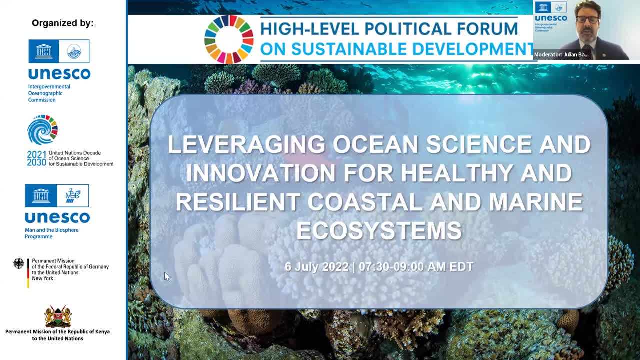 provides the formal review process for the implementation of SDG 14 this year in particular, but also it is addressing other SDGs, like SDG 15 on terrestrial biodiversity, or number four on quality education, as well as gender equity- number five- and partnerships- number 17.. 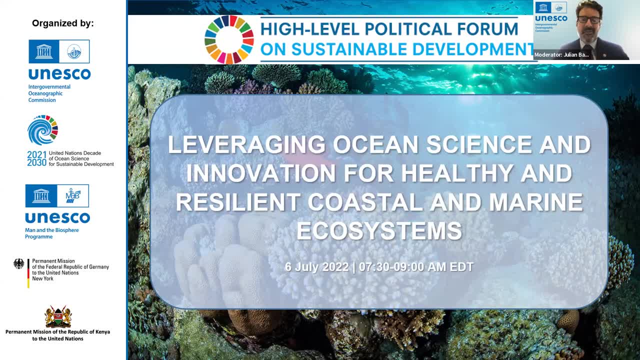 And I think, as we will hear across during our side event today, the ocean really cuts across all these dimensions and we will, I'm sure, go into more in depth. The purpose of our event today is really to highlight why ocean science is so important to the 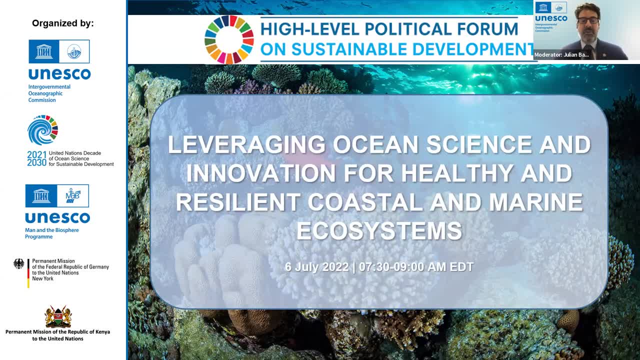 achievement of SDGs and SDG 14 in particular, but also to showcase what investments and partnerships in research are being done around the world and generating ocean observations, but also looking at different ways of engaging local communities to support sustainable development and to conserve and restore ocean ecosystems. So a couple of house rules, maybe, before we go into the 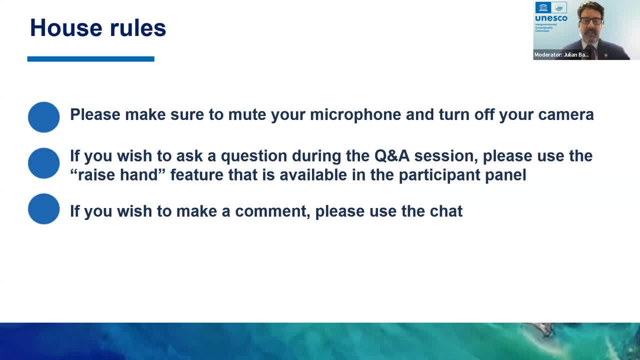 structure of our meeting. I just want to highlight that we will have, if you could, kindly turn off your microphones and cameras during the presentations. If you wish to make a questions- and I certainly hope we will have a little bit of time for Qs- and, As with our panelists, You will then. 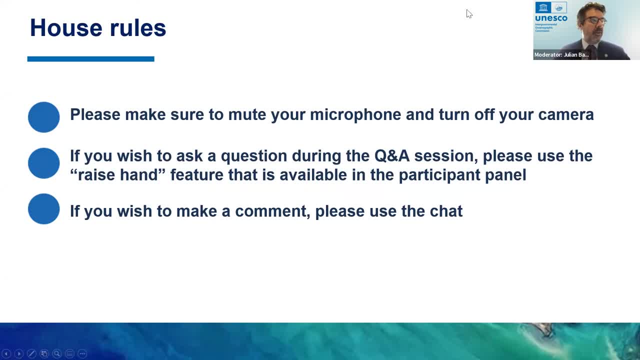 please raise your hand, which is basically one of the button at the bottom of your screen in the Zoom application. I'm sure by now you are all aware of how to do that. If you want to make any comments, please use the chat and also, if you have any technical issues, please also use the chat. In terms of the structure of our 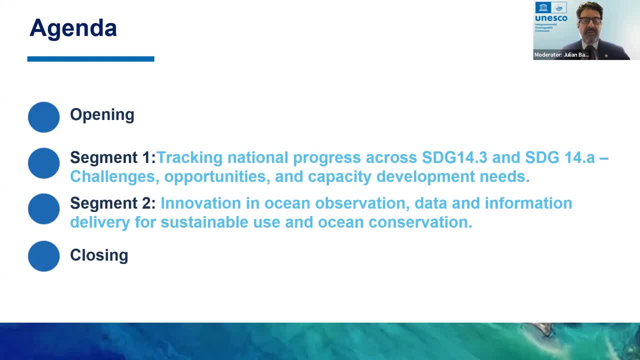 one hour and a half event today. we will have a first segment Now. first of all, we will have the opening and we will hear from our two sponsoring member states, Kenya and Germany, and then we will also have a pleasure to have our Assistant Director General of UNESCO, Vladimir. 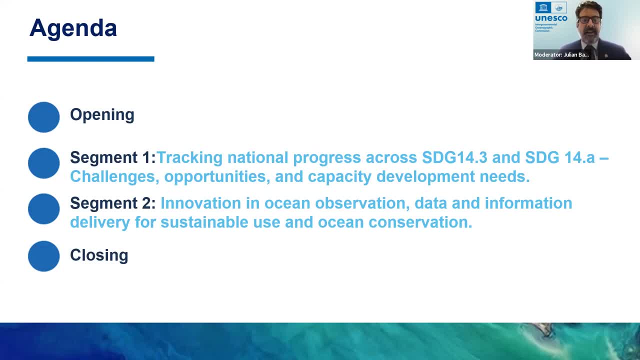 Yabinin with us for some opening words And then we will go straight into our two rounds, two panels. First one is really focused on the progress and challenges and opportunities in implementing SDG14, with a focus on two areas where UNESCO and its IOC are particularly engaged, And then the second one, too, will focus on innovation. 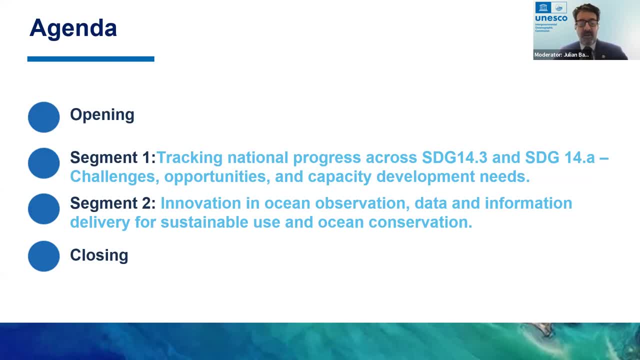 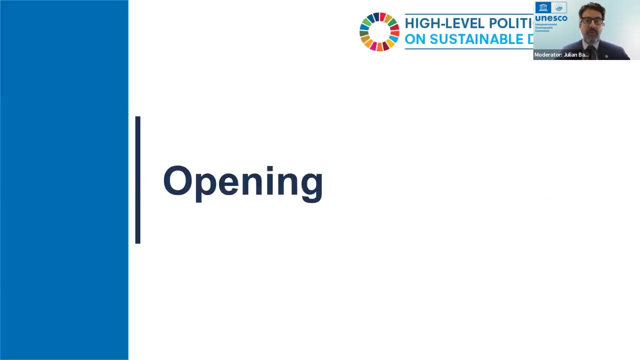 in ocean observation technologies and information delivery, but also talking about socio-ecological innovation in terms of empowering local communities to build resilience and protect biodiversity. So, without further ado, I would like to go straight to the opening segment, and we will have a welcoming word from: 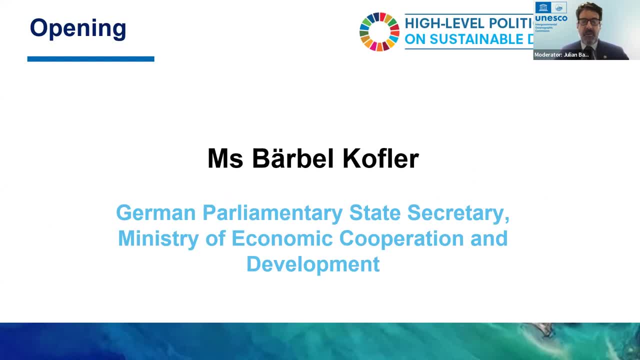 Mrs Birbel Koffler, German Parliamentary State Secretary from the Ministry of Economic Cooperation and Development, And we have, I believe, a video message from the State Secretary. If we could play this, thanks, TRANSLATED PERFORMANCE YABININ: 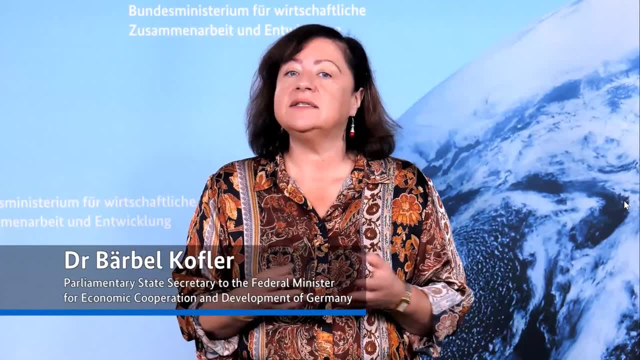 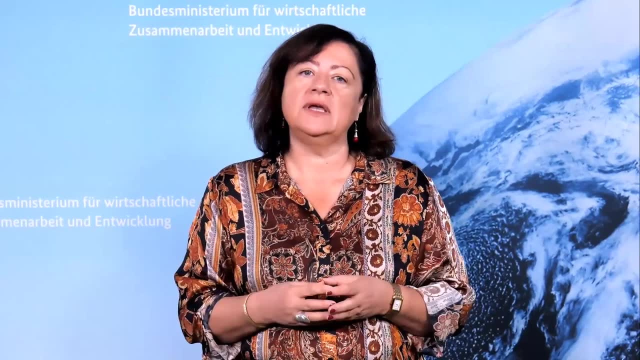 Dr Yabinin, Excellencies, Ladies and Gentlemen, Oceans are the source of all life. They cover 70% of the Earth's surface, are home to a wealth of biodiversity, provide food and income for millions of people across the world. 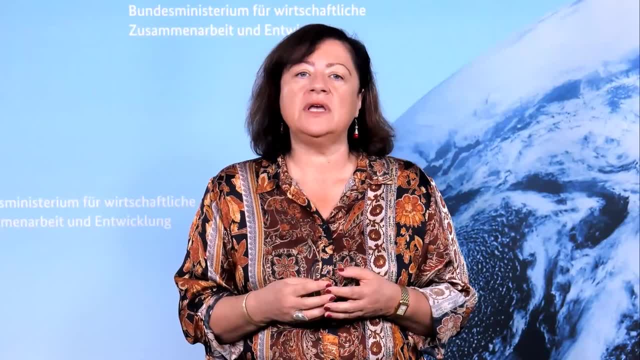 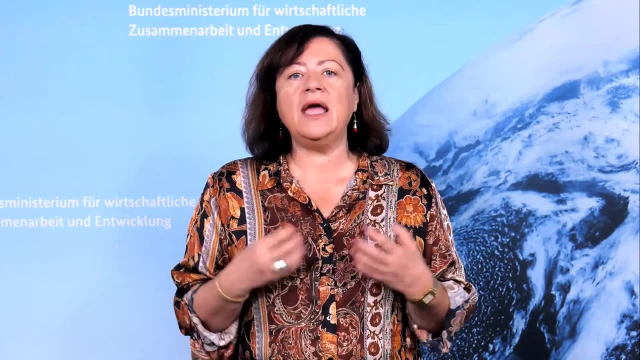 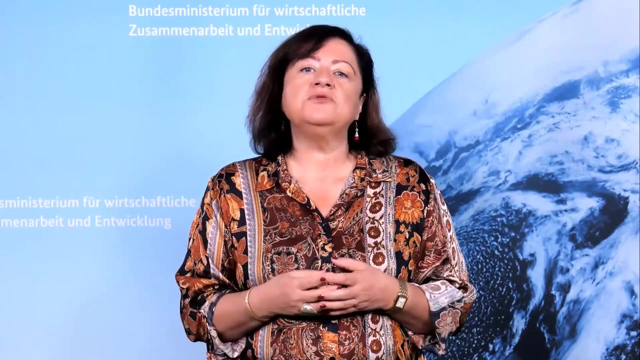 and regulate our climate by absorbing heat. So we can only conserve biodiversity, mitigate climate change, reduce poverty and achieve sustainable development if we also protect the oceans. Yet oceans are in increasing distress as a result of advancing climate change, increased population acidification and overfishing. 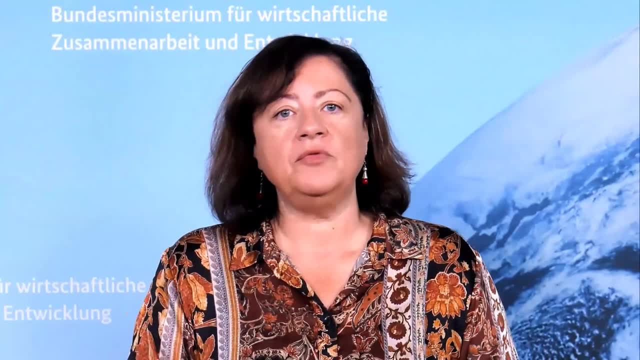 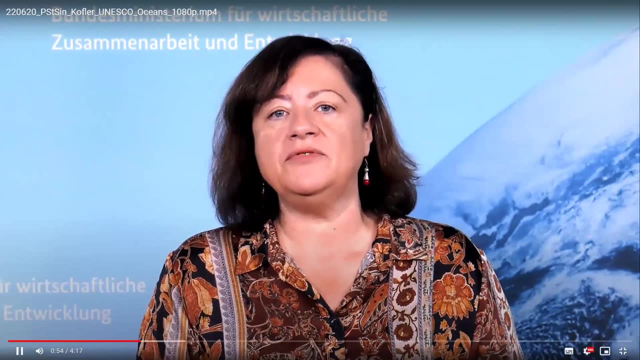 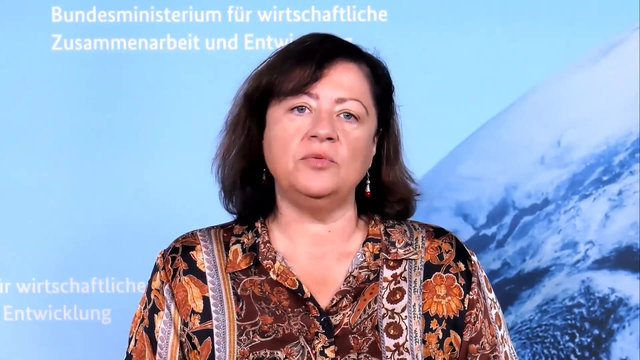 We must act now, before it's too late. We need to make sure that today and in future generations, all people are able to enjoy the benefits of healthy marine and coastal ecosystems. That means the international community stepping up its efforts and halting the loss of ocean biodiversity. 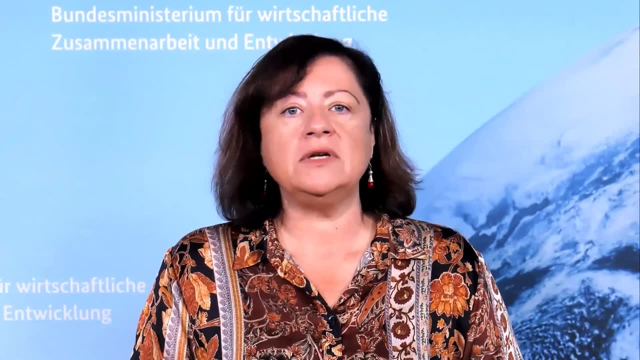 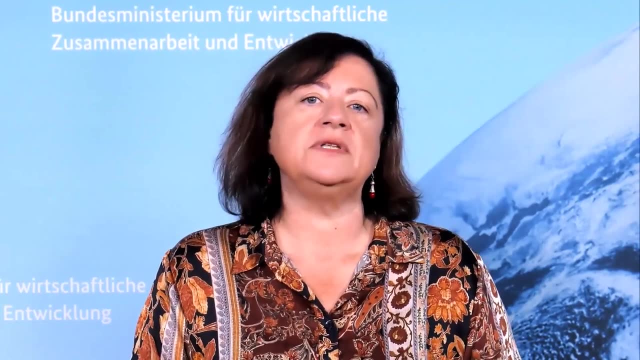 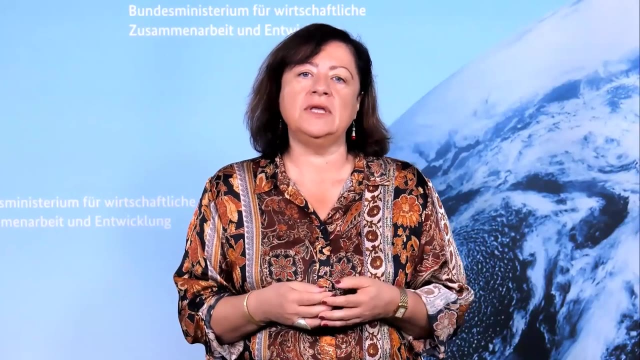 Yet, with a financial gap of 150 billion euros- 150 billion euros, 150 billion dollars a year, SDG 14 is currently one of the most seriously underfinanced goals of the 2030 Agenda. Ocean research is still suffering from a lack of funding, staff and institutional support systems. 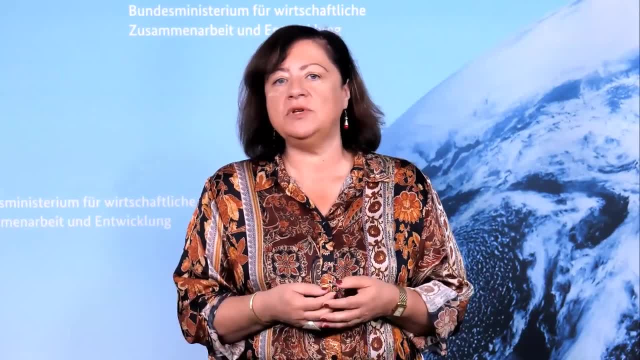 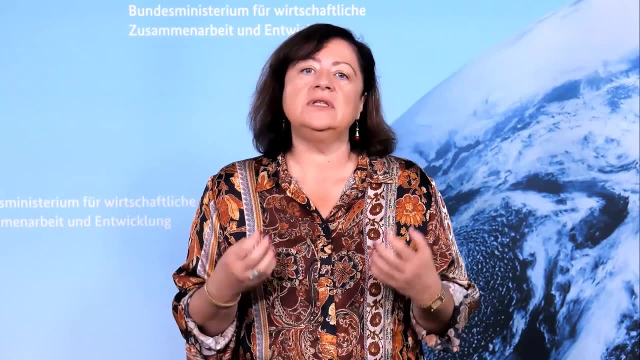 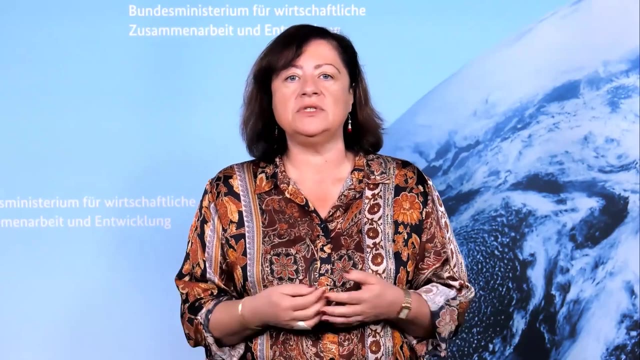 As a result, the international community lacks the fundamental knowledge and information it needs to effectively protect the oceans. We urgently need more research to tell us how we can most effectively restore, strengthen and protect maritime ecosystems. The German government therefore welcomes the United Nations Decade of Ocean Science for Sustainable Development. 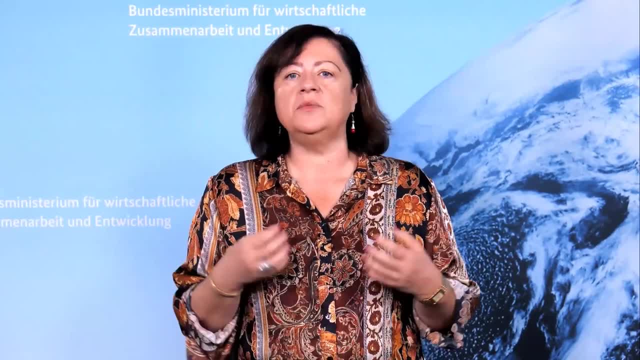 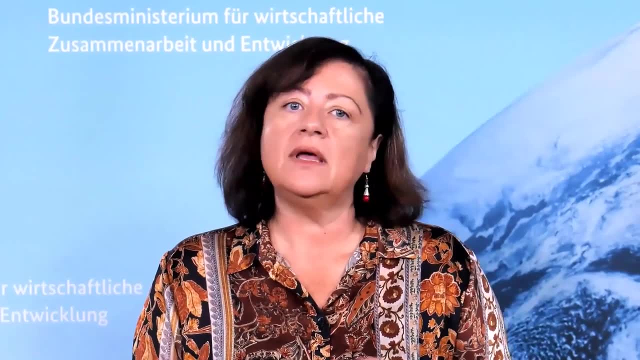 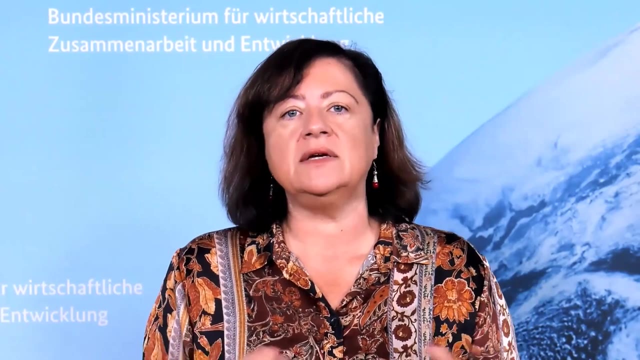 which aims to increase the focus on the important topic and generate new momentum. The German Development Ministry launched the initiative MIR Wissen- African-German Partners for Ocean Knowledge back in 2018, with the aim of uniting policymakers and scientists in the search for workable solutions to maritime protection. 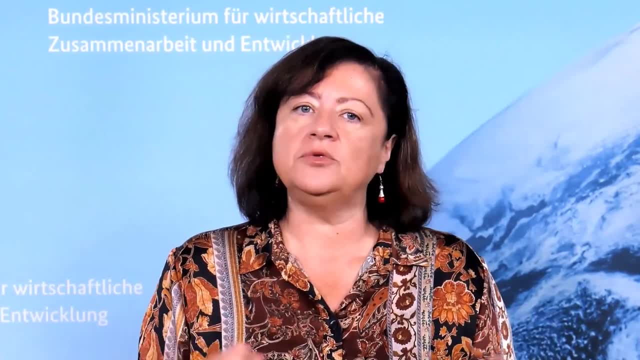 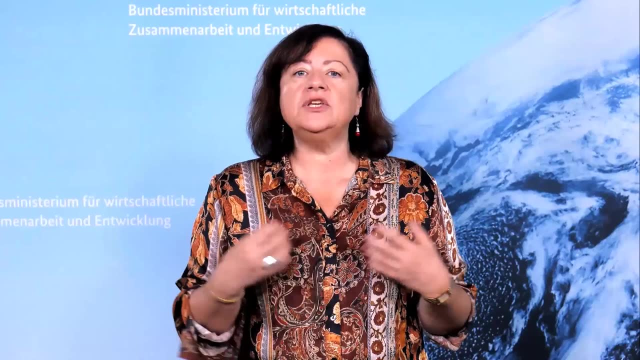 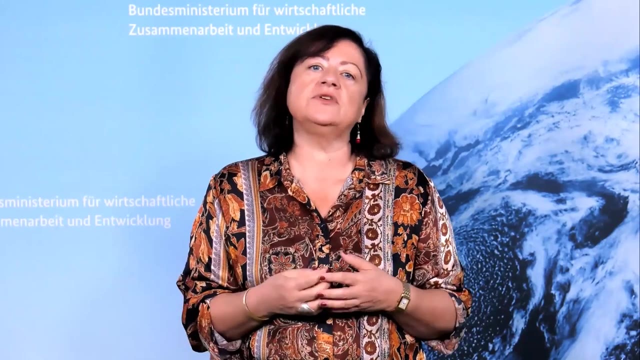 The initiative is supporting German-African research partnerships in 12 projects in seven African countries. The recent third call for proposals, issued together with UNESCO-IOC, is likely to result in a further four projects which will focus on nature-based solutions. I am pleased that today's event will also be looking at that approach in more detail. 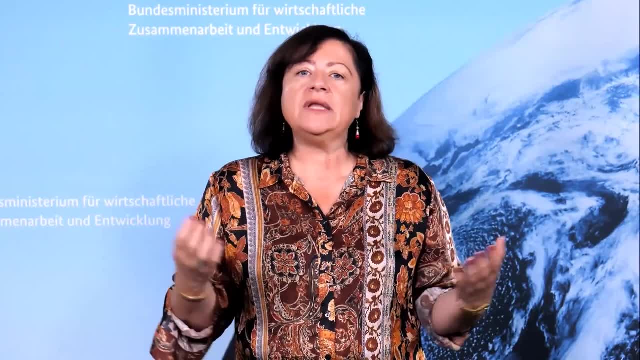 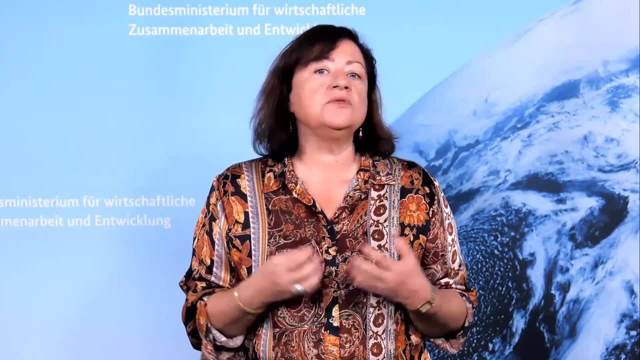 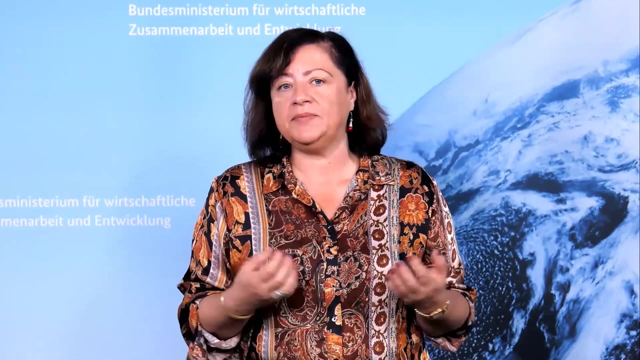 The aim of the MIR Wissen initiative is to better lay the groundwork for the future of science and policy makers. Its goal is to produce research findings that will help policy makers reach decisions. To that end, it has developed an innovative approach called co-design. 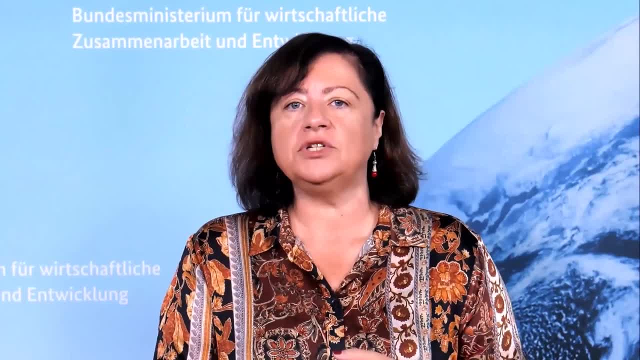 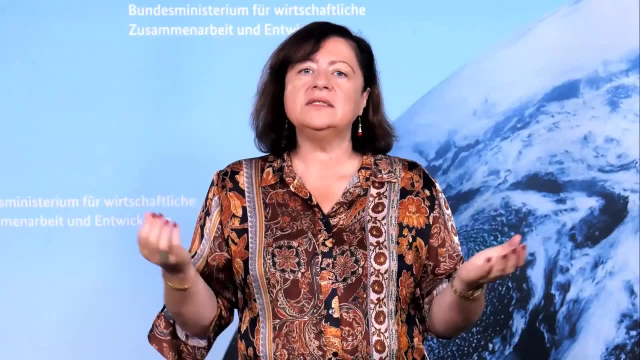 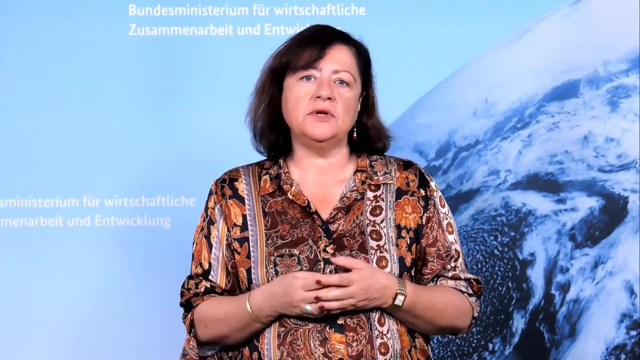 It ensures that all stakeholders are involved in research projects right from the outset and have a say in everything from the design to the decision-making process. This means that new findings are not just generated, but still actually applied within the context of a holistic, science-based marine conservation. 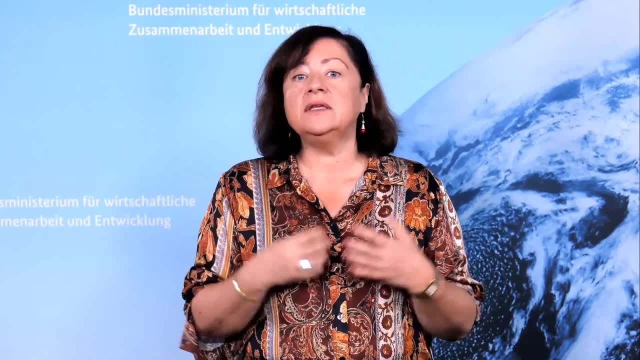 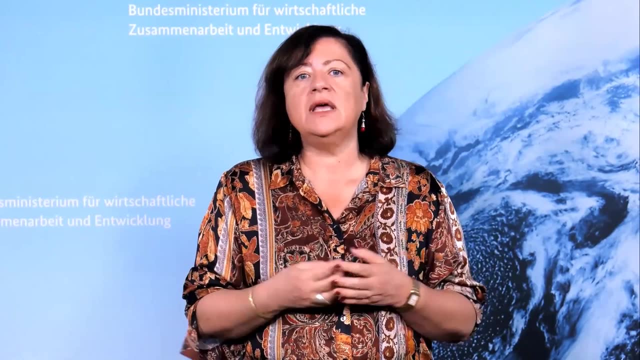 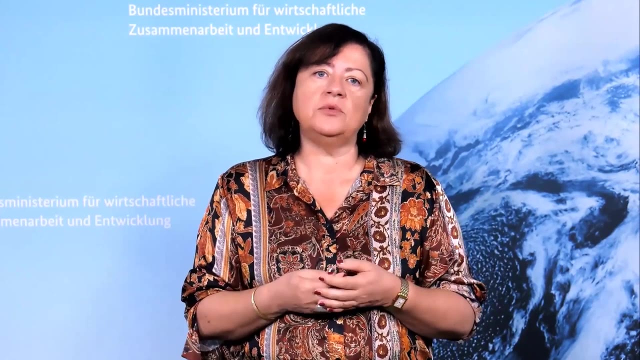 We at the German Development Ministry are delighted that the MIR Wissen initiative can make such an important contribution to the United Nations Oceans Decade as an official endorsed action. I would like to thank UNESCO-IOC for our close and productive collaboration on this. 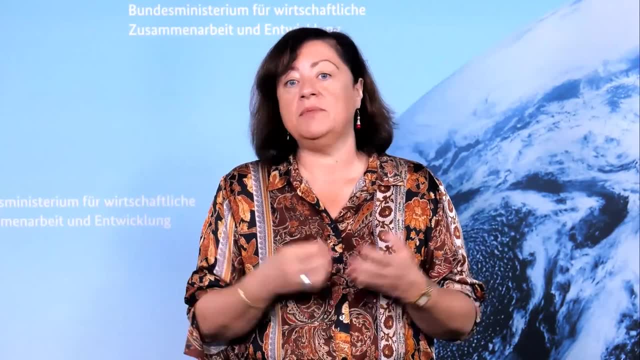 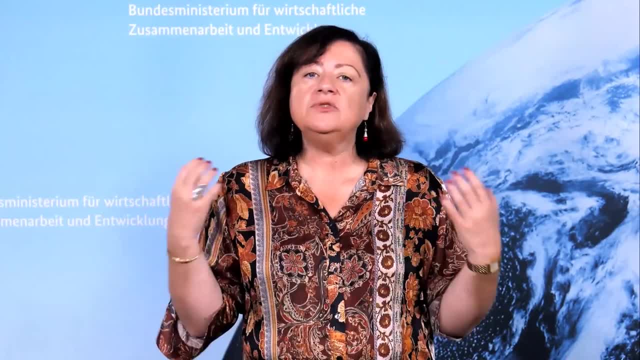 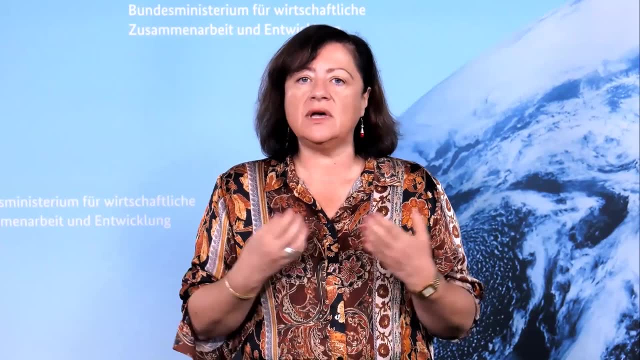 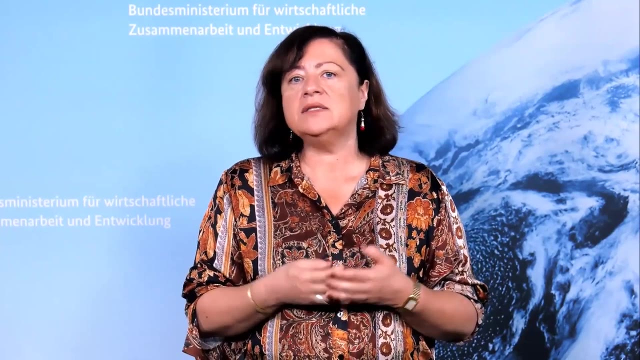 part of the UN Ocean Decade. Please do join us in supporting this initiative because, looking to the future, we need to unite civil society, governments and other stakeholders in defining the questions science should address. This is a way to ensure the solutions developed. 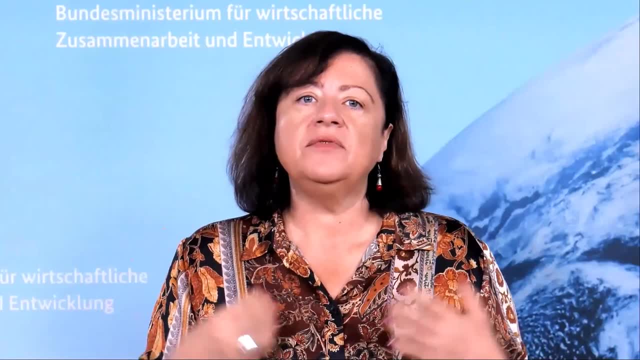 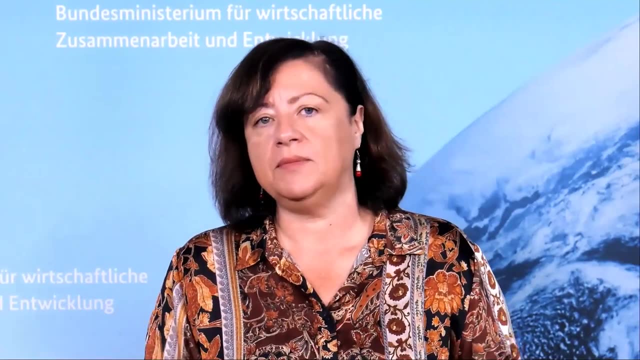 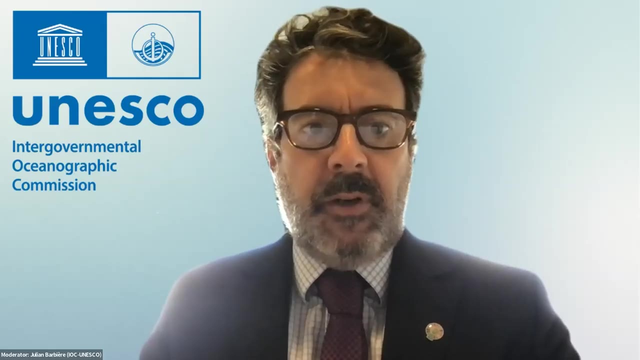 are actually workable in practice. That is the only way we will have a transformation impact and succeed in protecting both humans and oceans over the long term. Thank you, Thank you very much, State Secretary Koffler, And, of course, we are very grateful for the 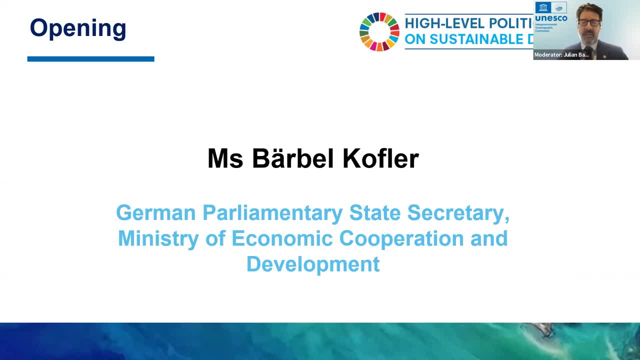 support of Germany in the work of the Ocean Decade. As it's been mentioned, Germany also supported the launch of a decade with the first international conference, Which you know was a very intensive but very productive process for the Decade Laboratories. that generated a lot of enthusiasm and great ideas for the Decade. 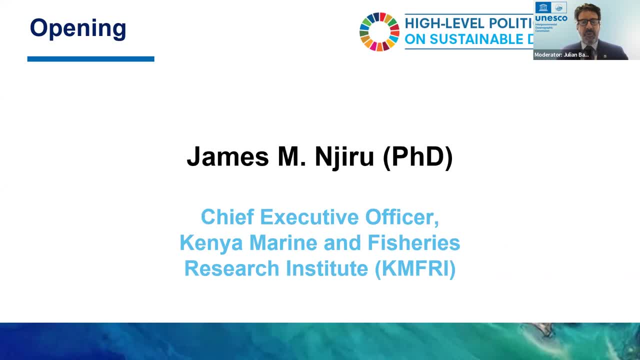 My next speaker is representing a country which is also very much involved in the world, to introduce James Njuru, the chief officer from the Kenya Marine and Fisheries Research Institute, Over to you, Professor Njuru. Thank you, Julian. The camera says that you have stopped. You cannot view me, So I will proceed. 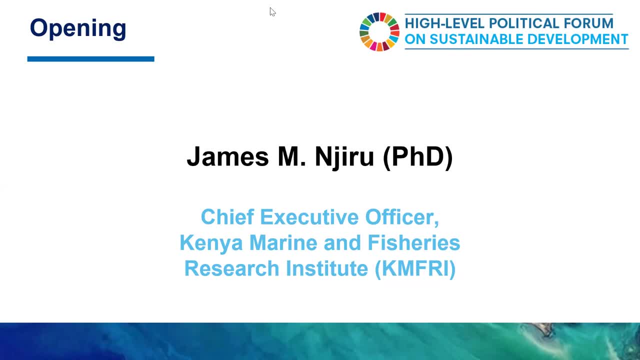 even without the camera. Is that okay? It says you cannot start your video because the host has stopped it. Yes, Okay. as you move on, let me take this opportunity also to thank you and the organizers. May I start by saying that science tells us most of the ocean remained quite unexplored and 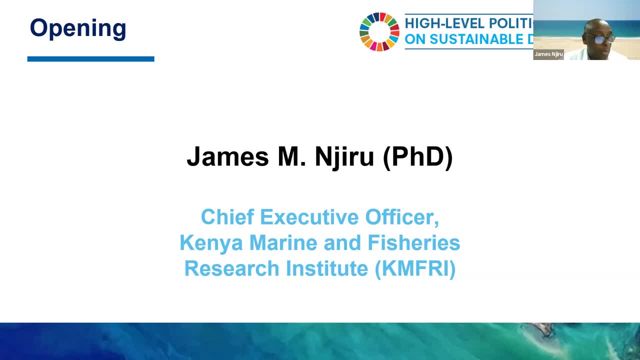 as the saying goes, that only probably 5% of the ocean has been explored and chartered by human beings. Additionally, as the saying goes, you cannot manage what you do not know. That is why, in my opinion, the UN assembly was put on to task- IOC, UNESCO to go and finish. 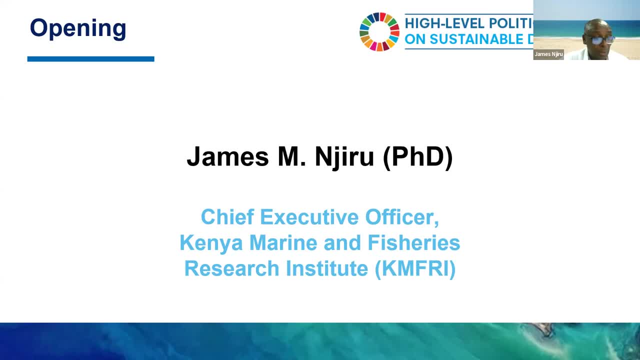 the proposal. Let me get into what happened at the UN General Assembly meeting At the UNESCO to coordinate the decade of ocean science, what we now call the decade, the 10 years which are now dedicated at ocean science and literacy and management. Ladies and gentlemen, the decade resonates very well with the current scenario in our 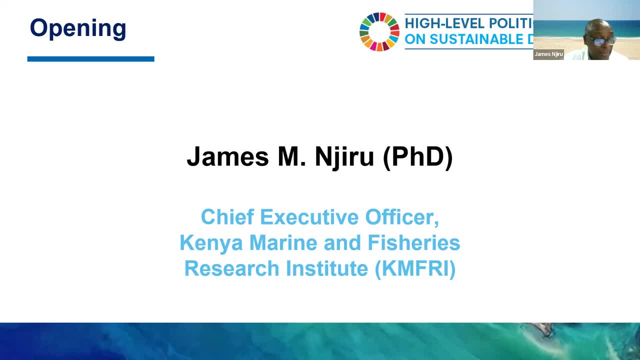 ocean, of course, inadequate data or lack of data, And that's why the theme of our decade is a science we need for the oceans, for the ocean we want, And it could not have come at a better time. The aim of the decade is to leverage on ocean science innovation that will be very key. 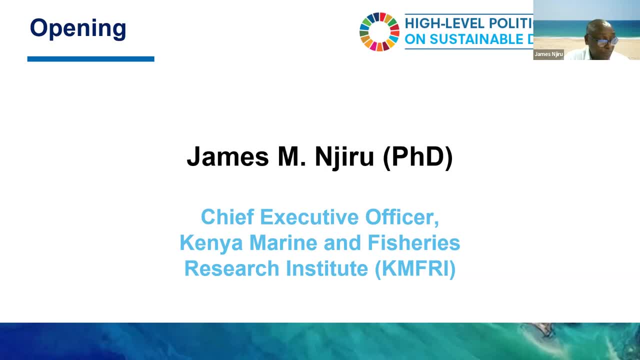 in managing and the exploitation of our marine resources. As we move on into the decade, we cannot fail to recognize the SDGs, the interlinked blueprint to achieve a better and a more sustainable future for all, especially in the ocean issues, For example, there is a very clear nexus. 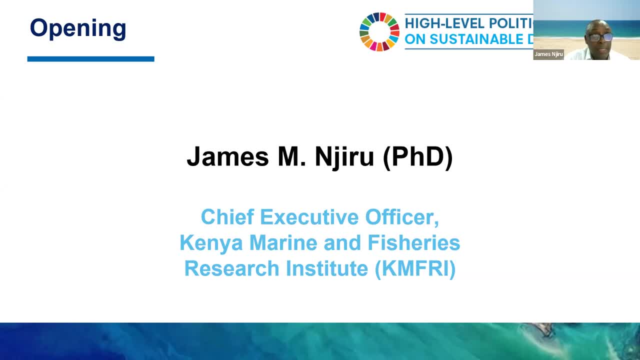 Among SDG 13,, that is, climate action. SDG 14,- life below water and, of course, SDG 15,- life on earth. The decade calls for action towards the nation. However, despite several challenges affecting the ocean, like pollution, acidification, 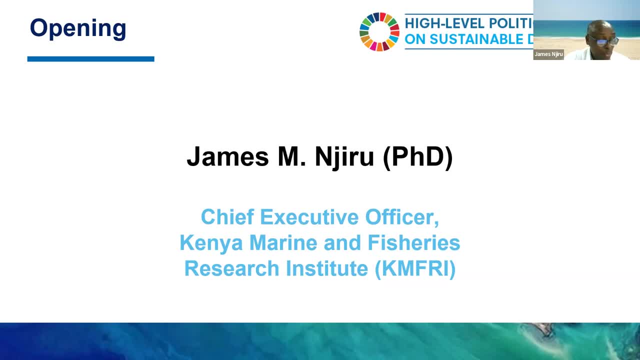 inadequate data, COVID and all the others. I would want to say that we are very happy as Kenya, Under the cognition of the IOC And the coordination of VAT bill. it is my opinion, it's an opinion that the one is progressing. 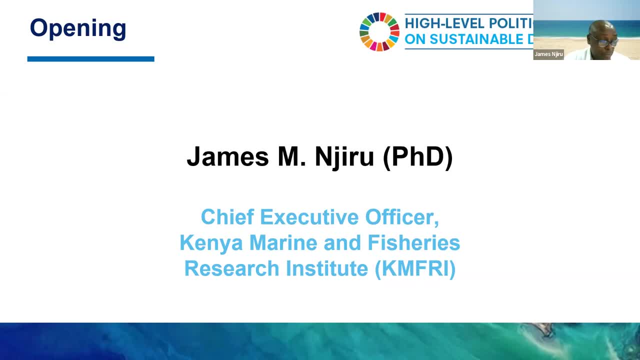 very well and in the right direction on the issues of matters of the ocean. They just concluded UN Ocean Conference in Portugal, in Lisbon, is a case in point. And you cannot forget, of course, other conferences, like the first Sustainable Blue Economy, which 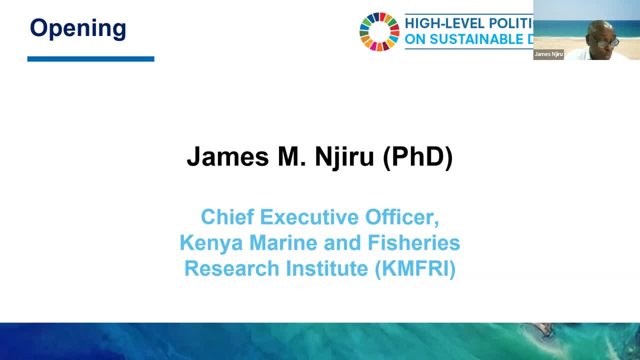 was held in Kenya in 2018, UNEA 2022, Stockholm Plus 2022,, among others, We are taking a notch higher in terms of commitment in issues of the ocean. There are several events which have been lined up in issues touching the ocean. 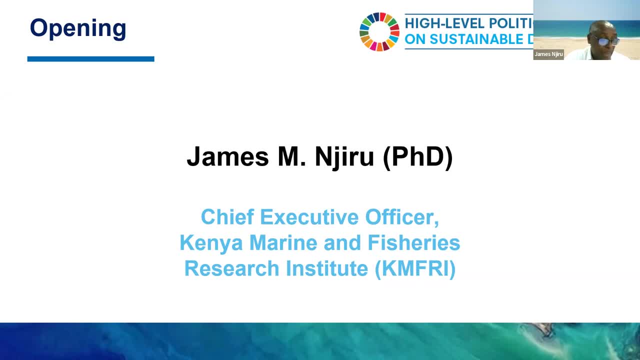 Some of them include ocean and environment meetings which are coming up, conference or parties which are coming up, and many more. We are now seeing a buy-in in key stakeholders concerned with ocean management and exploitation. Partnership is being cemented to us ocean issues. 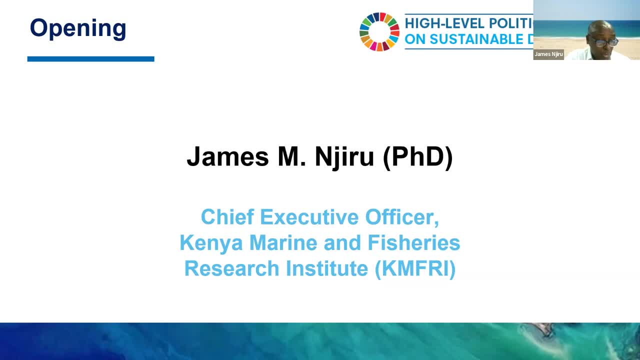 One cannot fail to mention the political goodwill currently being exhibited, And again I'll point to the second UN conference, which has just ended in Portugal, which was championed by two presidents: the president of Kenya and that of Portugal. And again we cannot fail also to recognize that the president of France, who also came, 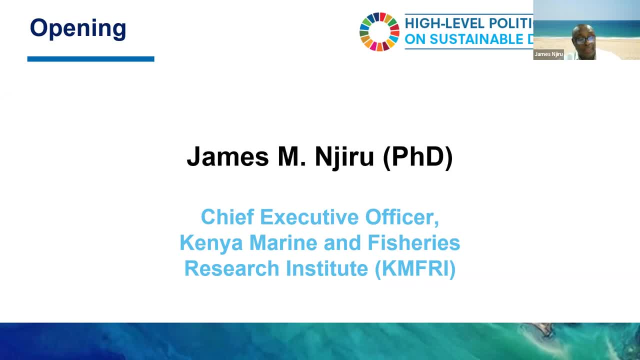 up there and Costa Rica have agreed again to co-host the next Ocean Decade in 2025.. We also have the Ocean Alliance and the high level panel, which are populated by hands of states. It's a good thing as we move on. 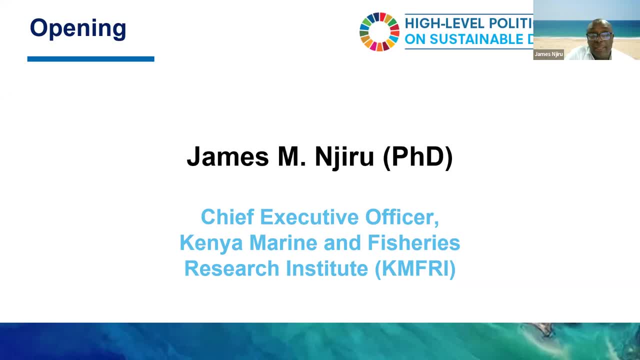 And because we know that SDG 14 is one of the least funded SDGs and probably the least understood. as we move on, However, these seem to be changing, with this political goodwill. As I conclude, I come from a marine science institution known as Kenya Marine and Fisheries Research Institute. 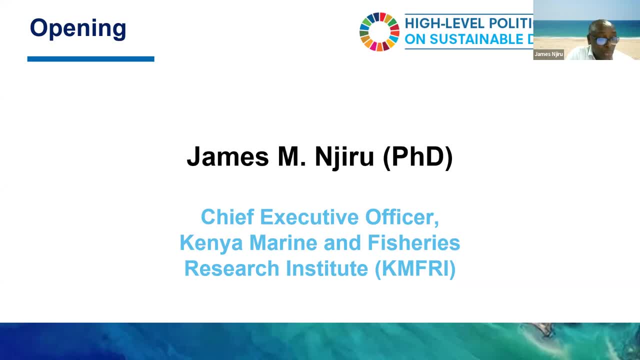 And we two are partners. We work together, embraced the ocean decade mission of transformative ocean science solutions for sustainable development, connecting people and our ocean. ladies and gentlemen, we acknowledge the need to create ocean science with partners for multiple skills. we need to match the the social science discipline. 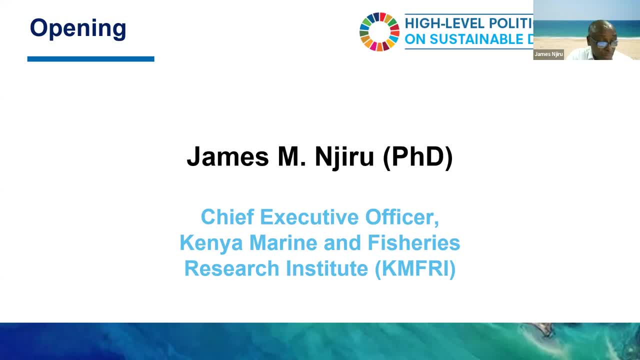 and scientific standards, among others. we need to support the application of ocean science for societal benefit as we as we integrate the sense to policy dialogues in the journey. finally, as as ocean stakeholders, we should seize this golden opportunity in furtherance of sustainable and the ocean. finally, let me take this opportunity to thank the organizers of the side event. 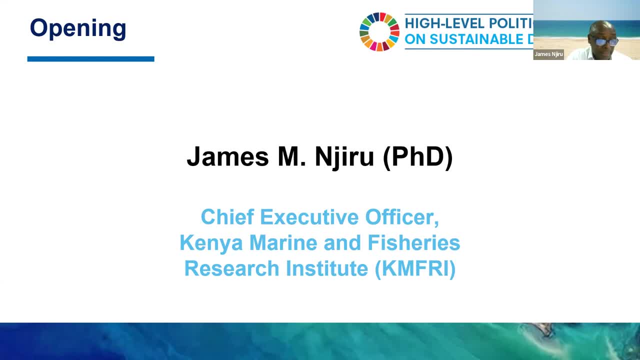 that is continuing to build momentum on the ocean science in the decade. we should not tire in this endeavor, and the more the better. we should not. we shouldn't forget to leave a better ocean for our next generation. I thank you all. Thank you very much, Professor Njuru, and thank you for the great leadership that Kenya 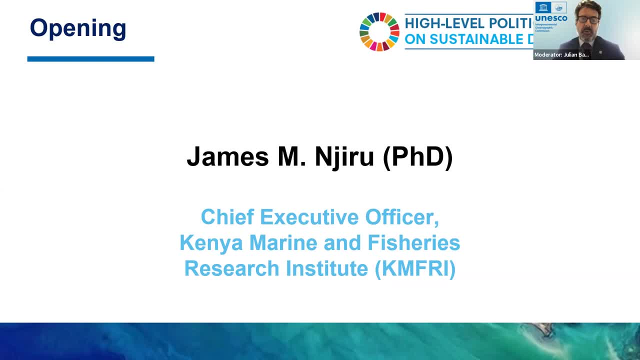 has demonstrated And, as you mentioned, it was also a real pleasure to hear President Kenyatta at the Ocean Decade Alliance event last Monday in Lisbon to commit to the work of a decade, but also calling his peers to also invest more in ocean science. So thank. 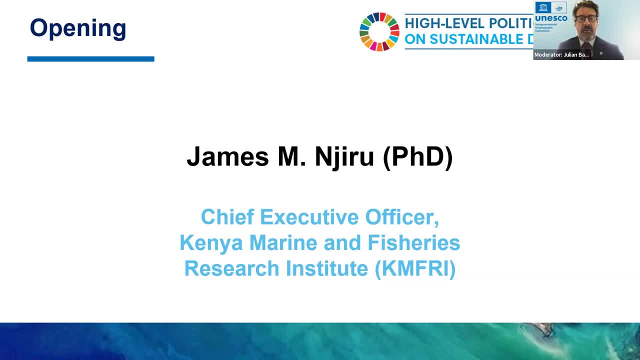 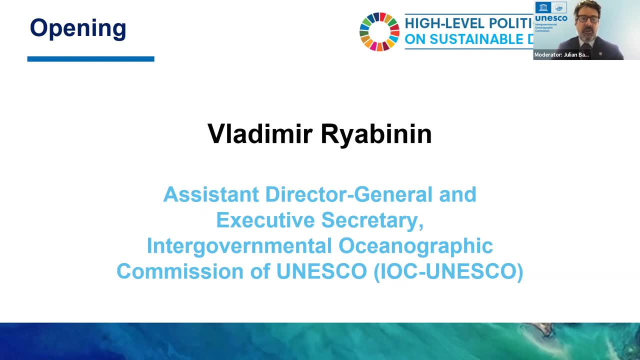 you for that. With this, our last speaker for the opening segment is Dr Vladimir Ryabinin, Assistant Director General of UNESCO and Executive Secretary of the IOC. Over to you, Vladimir. Thank you very much, Julian. Let me greet all the participants. I see 92 participants. 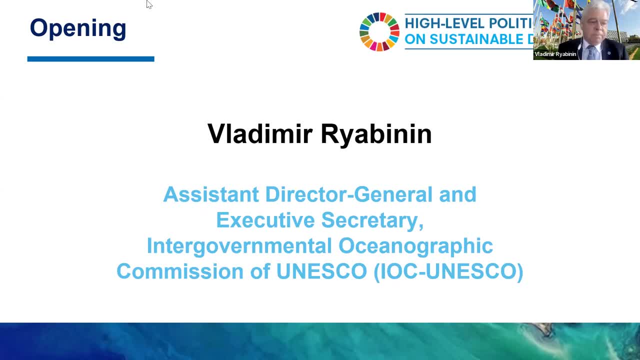 in the call: Hello, Hello, if you can hear me, that's great, We can hear you, I believe. Thank you very much for the invitation. Thank you very much. Thank you very much, Dr Ryabinin, for your introduction. 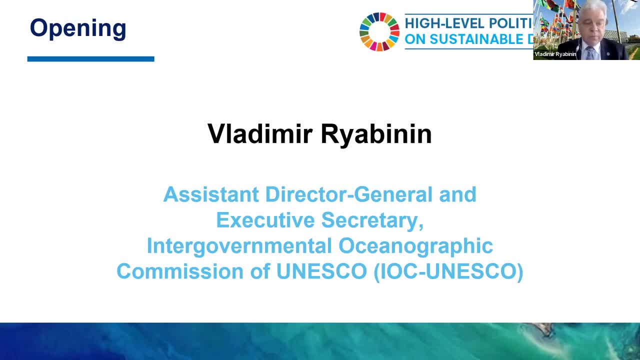 I am a researcher for ENS, the Institute ofapplied and scientific research on ocean science, which is a science and data science center in Kenya, And I am very happy to be the host of this session. I am very happy to be the host of this session. 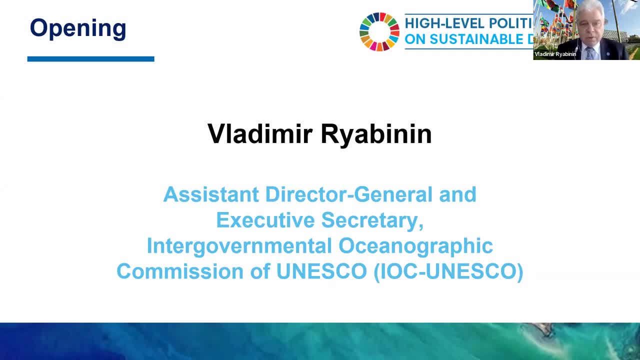 Thank you, Thank you very much. research institute that does very important work in all aspects of ocean sciences. you know many people refer to the conference that took place last week and at the start of the conference united nations secretary general antonio guterres recalled that sustainable development goal 14. 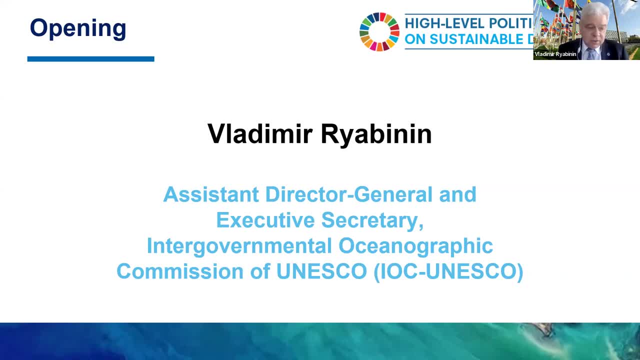 is actually the least funded among all sdgs, but it is definitely central for achieving all the goals of the sustainability agenda. indeed, ocean is the center point of many issues and because of that it suffers from multi-dimensional threats caused by combined pressures of climate change, overfishing. 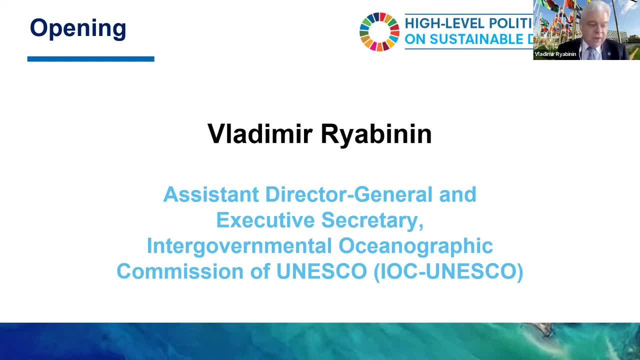 biodiversity loss, pollution and many other activities that result from us humans, and indeed the solution to this is is based on science, and that is also confirmed very, very visibly by the conference in lisbon last week that identified science and innovations as key enablers for implementation of sustainable development, goal 14, but also many, many 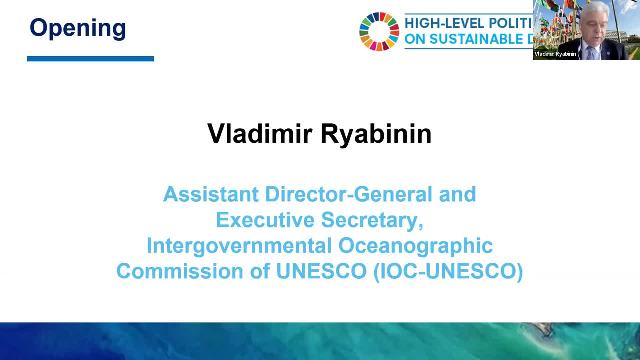 sustainable development goals. almost all of them have an ocean dimension, including uh, of course, the sdg 13 on climate, uh sdg2 on food and receiving cities, and continue this list, of course. you know, indeed, ocean science is central uh. ocean is very difficult to to understand and to observe. 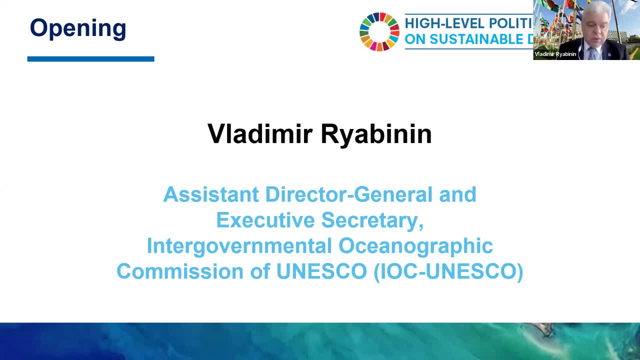 and ocean science is indeed needed to understand the changes in the ocean, also uh related changes in in climate and also in life on the planet. uh, and that would- we will very soon hear from uh participants- and jacqueline, who is going to present to you some results that shows, uh, that ocean science is critically underfunded and we do need investments. 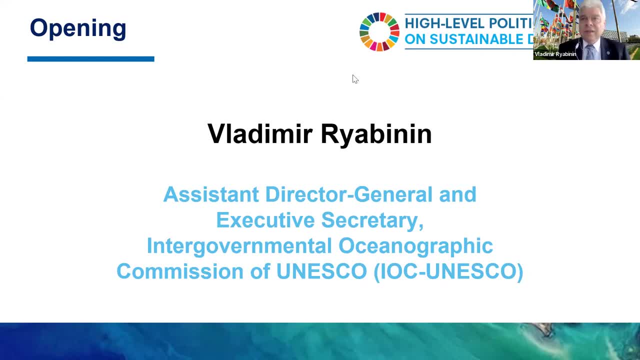 important investment. i actually insist on the world investments run than expenditures, because there will be very significant return. so we need investments, uh in ocean mapping, development of global ocean observant system, uh increasing prediction capacity, actual scope of predictions on ocean stressors, continue transfer of knowledge capacity, technology and also, of course, this has 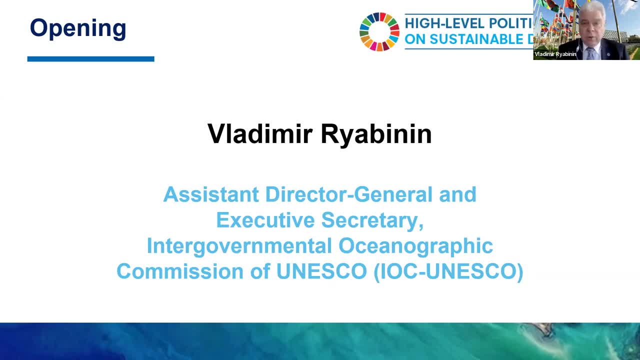 to be done between developed countries, small island developing states and least developed countries- we know how to understand theahah- and least developed countries. We know how to do it and there are mechanisms. So indeed, UNESCO and its Intergovernmental Oceanographic Commission play significant role, key role, in reporting. 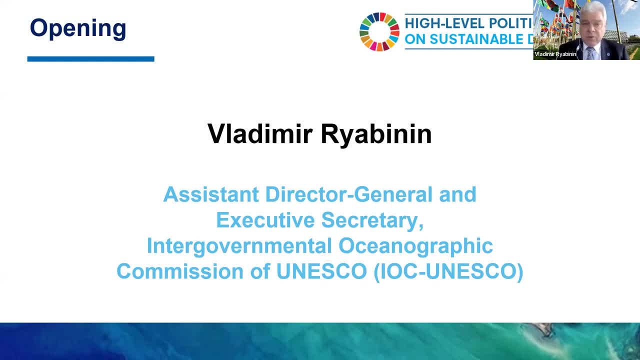 on SDG 14. And in the first part of that event you will hear more about our role as custodian agency for two SDG 14 targets. And then also we provide technical support, scientific support, to other United Nations agencies to work also and report to United Nations on marine pollution. 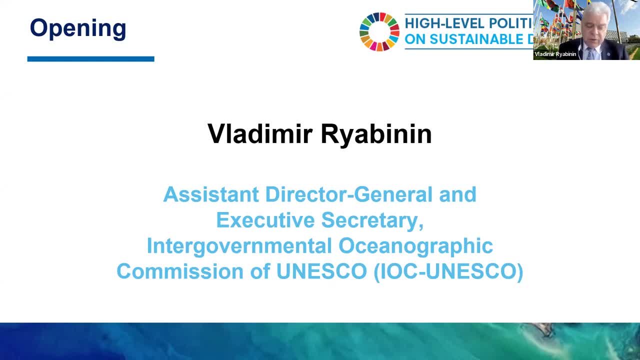 and ecosystem-based management. Indeed, RUC of UNESCO is the ocean science hub and because of that we accumulate knowledge on the state of the ocean. And at the conference last week we presented to the conference, to the world, a new report on marine pollution and ecosystem-based management, And this is a new report on marine 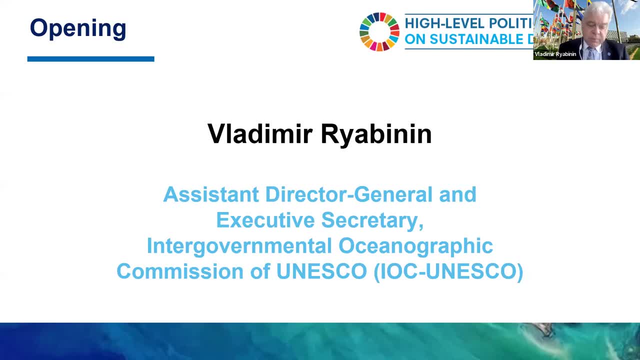 pollution and ecosystem-based management. And this is a new report on marine pollution and ecosystem-based management. And this is a new report on marine pollution and ecosystem-based management: State of the ocean report. It was launched in Lisbon and will be published on a regular basis to update. 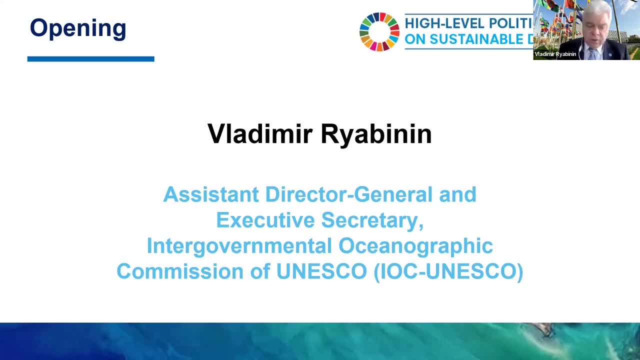 to keep the world abreast of the situation in the ocean, not only in terms of its physical or chemical biological state, but also in terms of management in the ocean. That is a big development And that report will be complementing activities of other United Nations organizations. 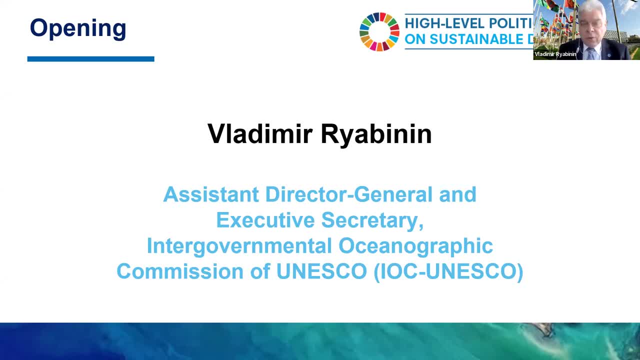 without any duplication. So I think from the old discussions it's clear that we have to create a revolution in ocean knowledge And for that we need a platform. So the international community agreed that we need also a significant time to make this initiative a large scale And because of that, United Nations proclaimed in 2017,. 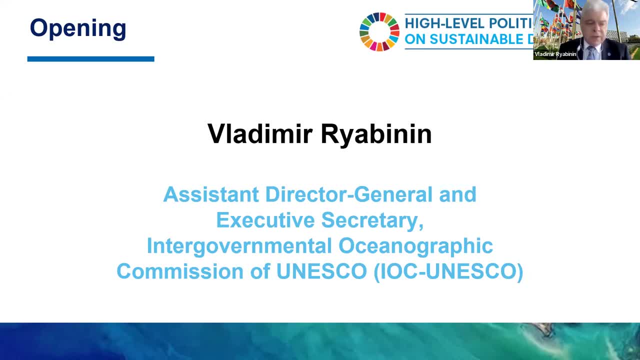 the Decade of Ocean Science for Sustainable Development and entrusted IOC of UNESCO to coordinate, prepare the plan, coordinate the implementation of the decade. I have to say I need to thank everyone for helping to craft the plan of the decade And now to reach unprecedented level of activities, turning the decade into largest. 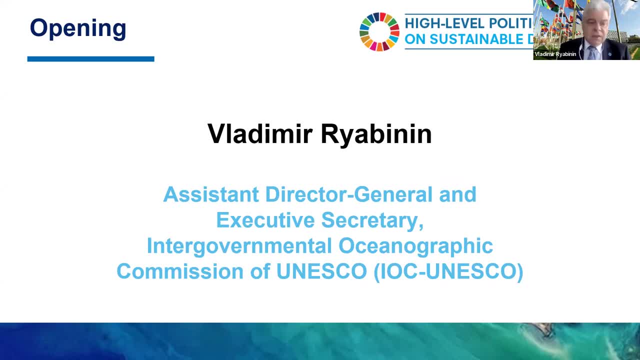 undertaken in ocean sciences ever. And indeed the declaration in Lisbon that was adopted last Friday calls specifically on nation stakeholders to support the decade and also the work of OECD to achieve the ambitions of the decade. So indeed, once again, the work on science is very essential. 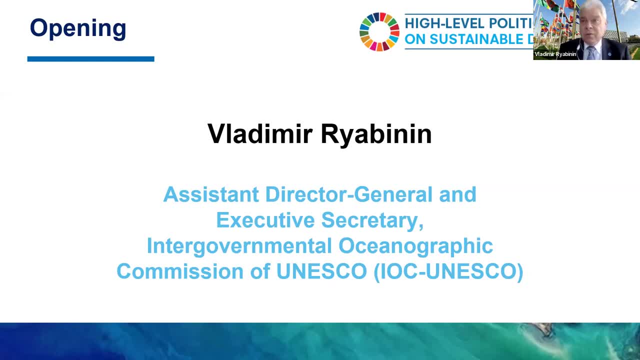 and we need to develop the knowledge. But you know, this knowledge has to be applied. We need philosophy and strategy for this And the philosophy and strategy basically, I think can converge to managing the ocean sustainably. We have elements of that work. 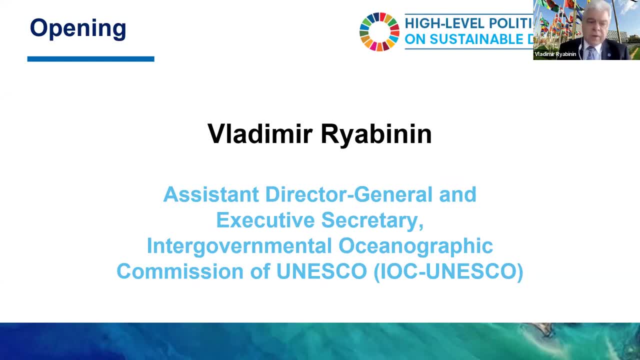 And UNESCO- not only IOC, but UNESCO is the big organization- provides framework for many activities focused on management of the ocean, For example, World Heritage, Marine Science. there are 47 of them. There is a network of 738 biosphere reserves, Many of them are coastal or marine, And we are really increasing dramatically the 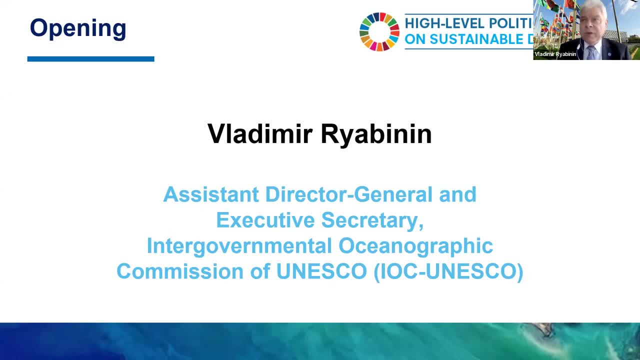 scale of maritime spatial planning. So the ocean is becoming more and more managed. But also we have to keep the world safe. And managing the ocean also involves keeping the world safe from tsunamis. So this is the ambition of the Tsunami Ready Program. 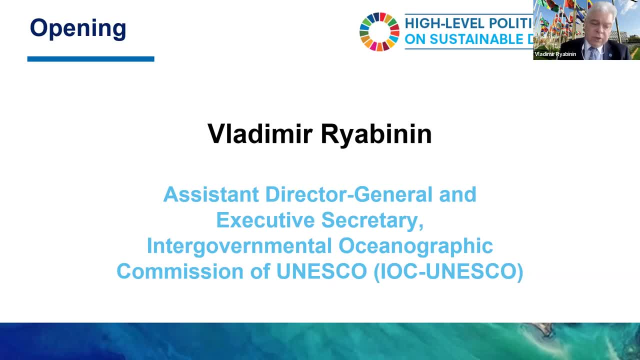 of OECD, to mobilize all available knowledge and not only to improve modeling of tsunami and warning system, but also enable societies to cope with natural disasters of this kind and really react when tsunami happens. and, of course, this is only possible when society understands the role of the ocean and what needs to be done with it. so, raising 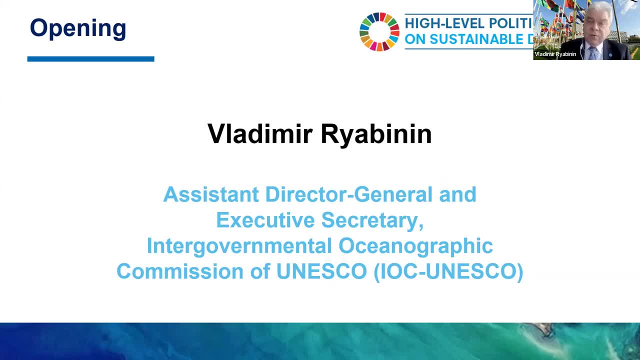 awareness is very, very important, and we need to involve many types of societal actors in this process. this, of course, requires also education. i'm very glad to see that our member states started to promote education in in schools about the ocean, and the vehicle for this is our work on ocean. 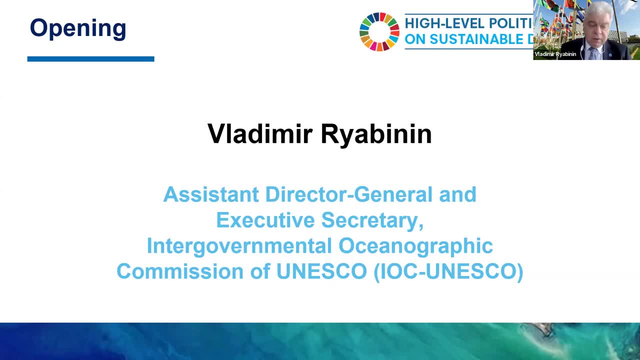 literacy that is taking, i think, unprecedented level and because of that we can cope. that will be a new future workforce and people will be developing their more human relations with the ocean. so working across the languages between many sdgs is important and because of that we organized this side event on the margins of the high level. 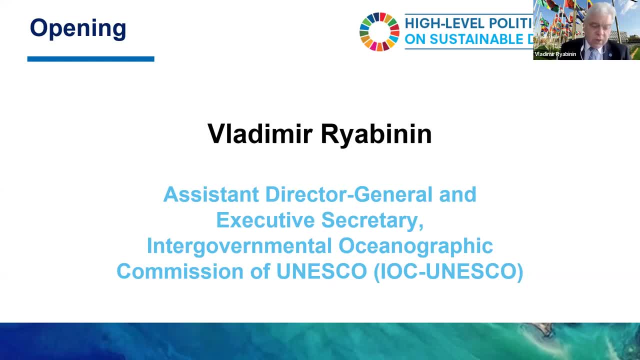 policy forum and we will try to explore how investment and partnership in research, observations feed for purpose data products, services can empower your member states decision making in relation to the ocean. this will definitely also support industry, local communities, support the better life of the whole world. so, with that very noble intention, contributing to your needs, i would like 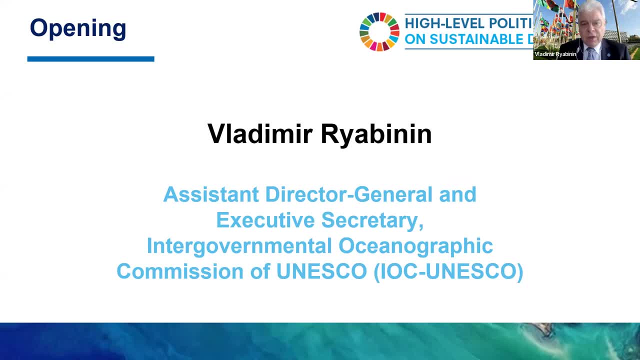 to uh return the floor to our moderator, julian barbier. thank you very much for participating in this important side event. thank you very much, vladimir, for for those good words and and for um defining and explaining the division of our, of our work uh at the integrand orthographic commission and unesco uh. so with this we can now go. 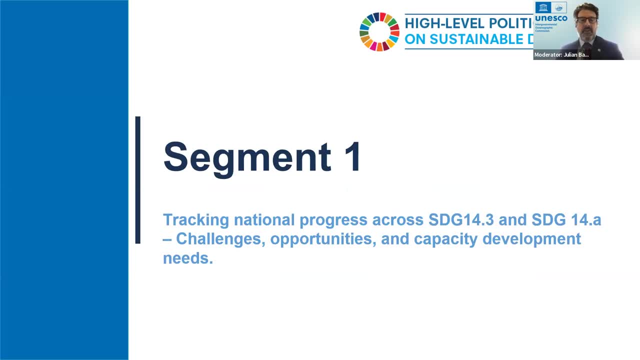 straight into our first panel and i have three grace great experts uh with us to talk about how nations are progressing uh with some dimensions of sdg 14.. we're going to focus particularly on ocean acidification and marine scientific research, looking at some of the challenges. 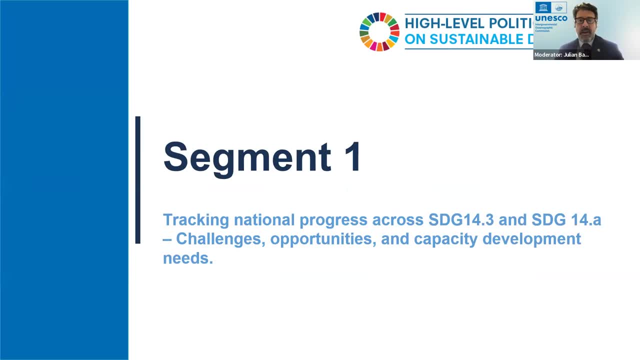 the opportunities, but also the capacity developments. so now to ask our three panelists to turn on their camera. so we have with us um dr jacqueline hooker, who is the director of the ocean science report, and uh jacqueline, who's the co-chair of the editorial board of the global ocean science. 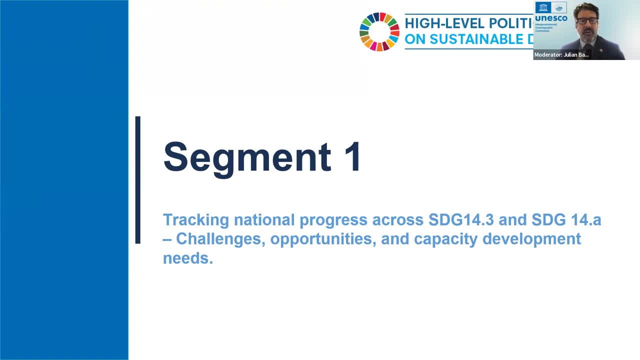 report, and uh jacqueline is with the kenya marine fisheries research institute. uh, we also have john newton, who's the co-chair of a global ocean acidification observing network. go out, and he's a senior principal oceanographer at the university of washington in the us. and then, finally, uh, we also have a pleasure to have uh evgenia kostianaya, who is a 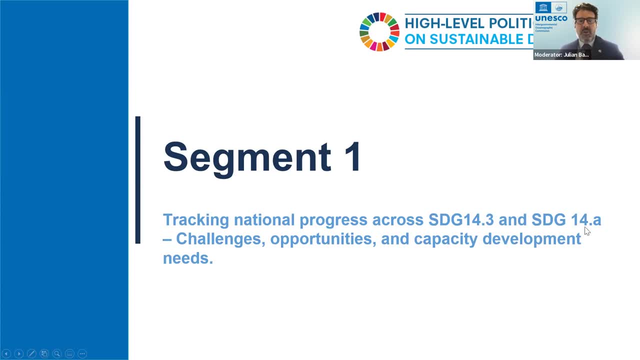 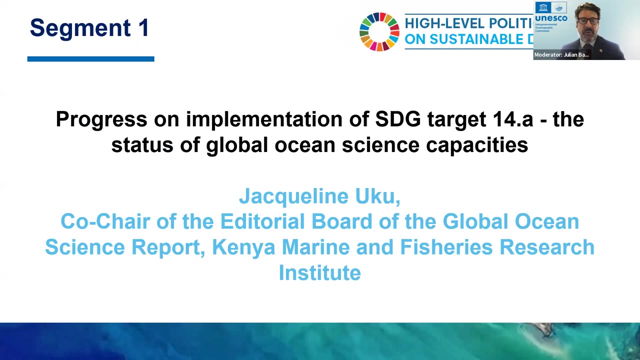 leader, the global leader for the un ocean decade program, focusing on the engagement of early carrier ocean professionals. so, with uh this short introduction, uh i think we're gonna go straight into our topic and i will uh first of all invite uh professor uku to give us an overview on where 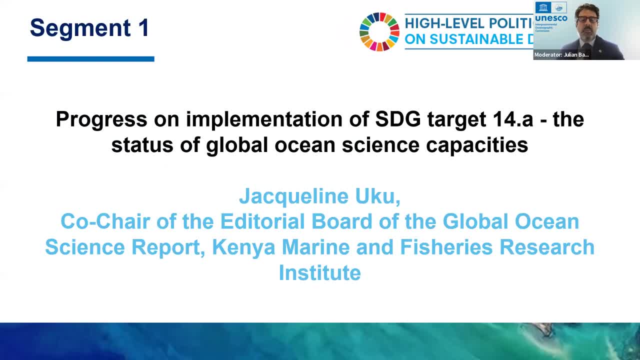 we are with the with this particularly important target, marine scientific research- and whether she's part of sdg 14 and what where we are with the status of uh of ocean science capacities around the world. over to you, jacqueline. thank you very much, julian. 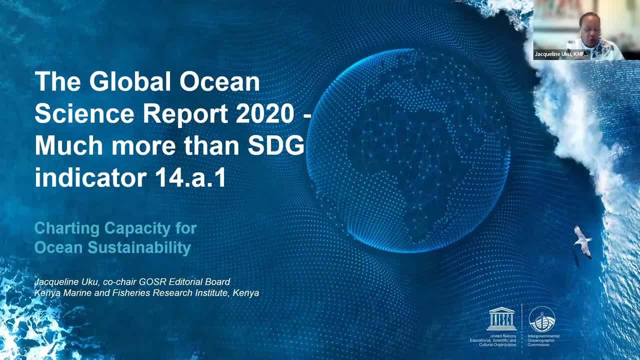 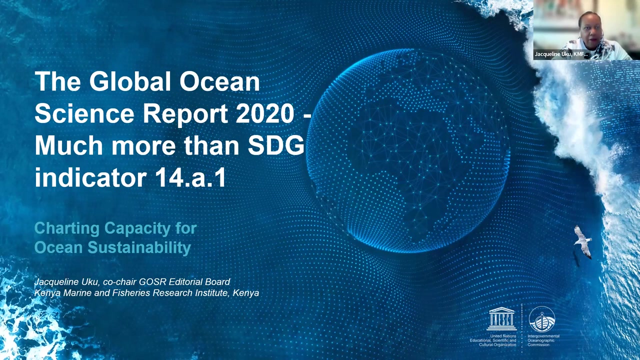 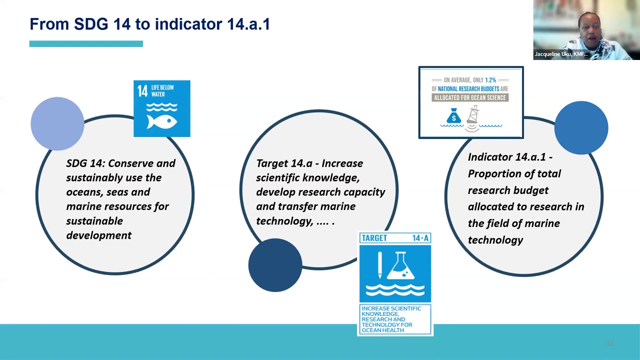 good afternoon, good morning, good evening, distinguished guests and ladies and gentlemen, my job uh today is to talk a bit about uh the ocean science uh report 2020, specifically the sdg indicator 14.a1, so we can have the next slide. uh indicator 14.a1 specifically looks at increasing scientific knowledge through the 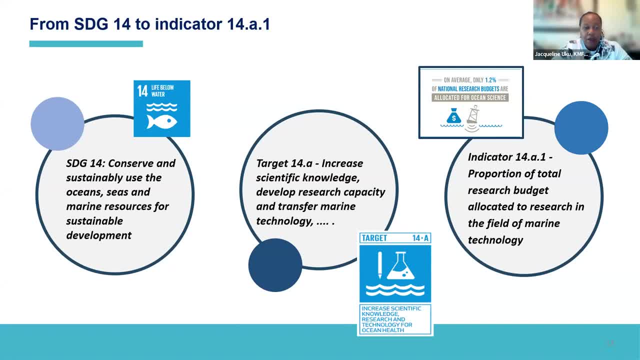 development of research capacity and transfer of marine technology and it falls within uh the sdg-14 which looks at uh life. Chapter 14 for became more famous during ten years from такой coverage over the decisions we have made in history over the last 30 years and we also punch plenty upon the progress of the India WOODRUFFI rules relevant and not only the ‑‑ and weächn inбоm qualified science studies, reading celle, the studies equality, Sanders sdg theuru getting class Aubrey, shesha huang, Michael Howay, fush, the katanya sdg indictionary for this 14 point a one specifically the sdg indicator 14.a1 specifically looks at increasing scientific knowledge through the development of research capacity and transport marine technology and it falls within the sdg14 which looks at life under development capacity and transport marine technology and the tail onun types as part of the. 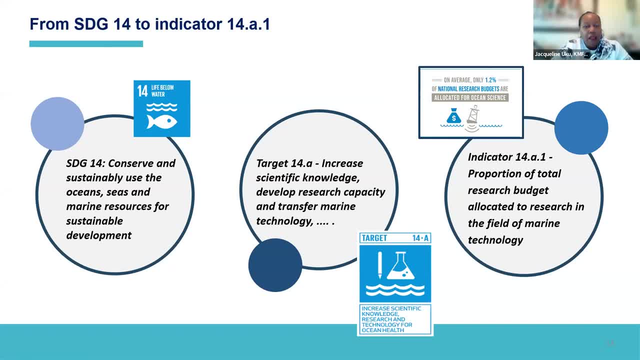 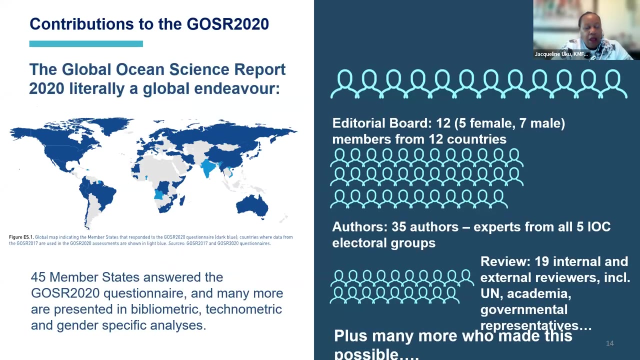 looks at life underwater and, more specifically, what we measure for this specific target is shown on this slide in 14.8.1, which is the proportion of total research budget allocated to research in the field of marine technology. we can go to the next slide. I'll on this slide I'll just explain what we did to undertake measurements of ocean science. 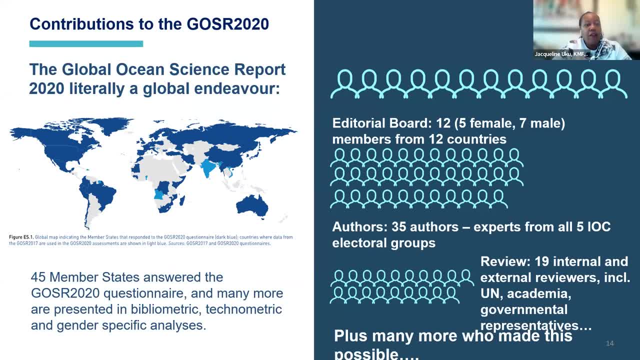 and contributions of member states towards ocean science. and we set out to measure and to get statistics and data to just evaluate where we are in terms of the targets that we had set under SDG 14.. and we sent out questionnaires and I'll go a bit more into the process, but what I'd like to point out is: 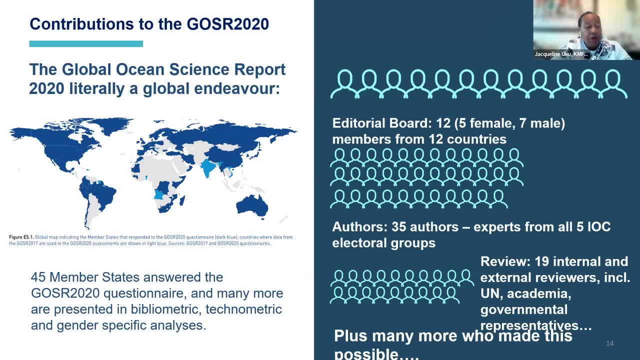 that, out of the maybe around 150 member states, we had 45 member states that responded to this survey, the questionnaire, and also we gathered information through bibliometric, tetra metric and genus gender specific analysis. our board was a board of 12 members, five female, seven male, from 12 of these member state countries. we had expert authors, expert 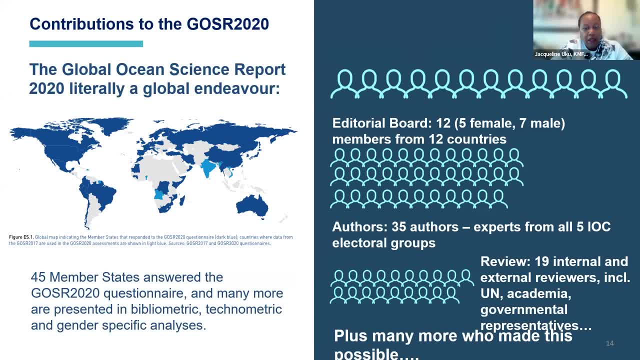 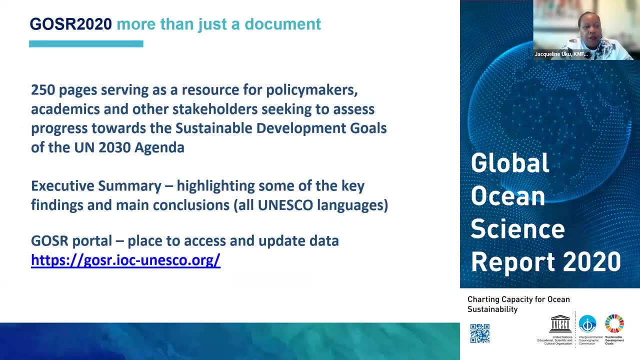 reviewers, and the report as it stands today is used as a baseline of our contribution to ocean science, and so we'd like to acknowledge all that contributed to this process and this report. next slide. it is a resource for policy makers and it can be found at that link. 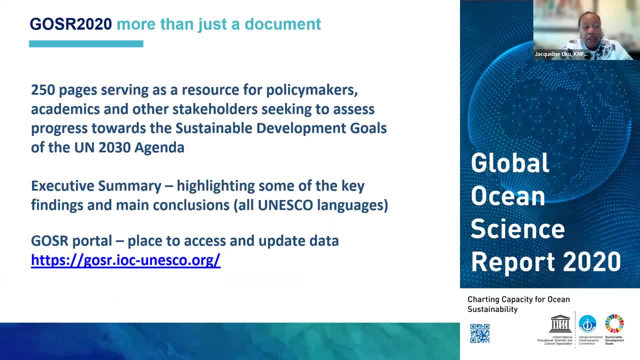 and the IOC UNESCO website and now, and it has an executive summary that highlights some of the key findings today. I'll just scope on some of the findings. and that is a very small amount, the proportion of the data that we collected. it's more than a document, it's actually our roadmap. 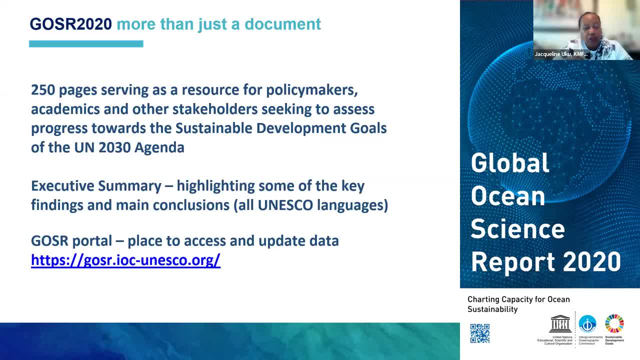 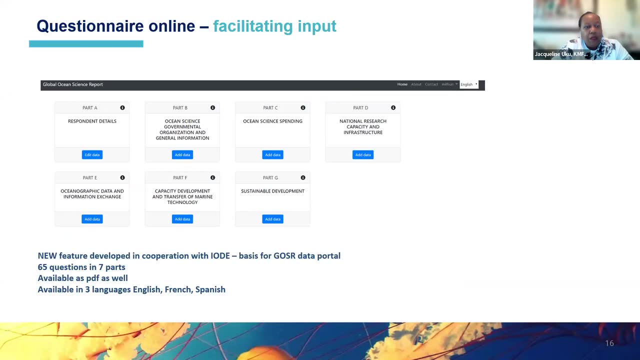 towards understanding how we are really contributing and how we value the ocean that we have been talking about, I think, in many, many dialogues and on many platforms. Next slide: Our questionnaire facilitated inputs. We had questionnaires that the questionnaire captured: governance and organizational information. 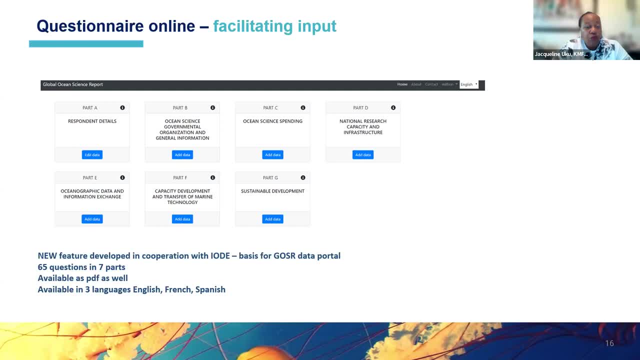 how countries spend on science, national research, capacity and infrastructure, oceanographic data and information And capacity development, as well as SDGs and our contribution particularly to SDG 14 and how it links with specific SDGs, And the report is available in three languages. 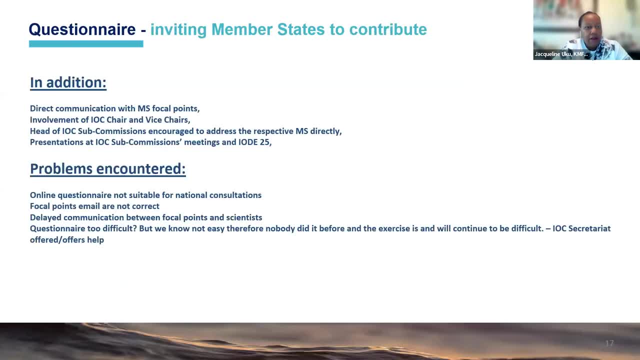 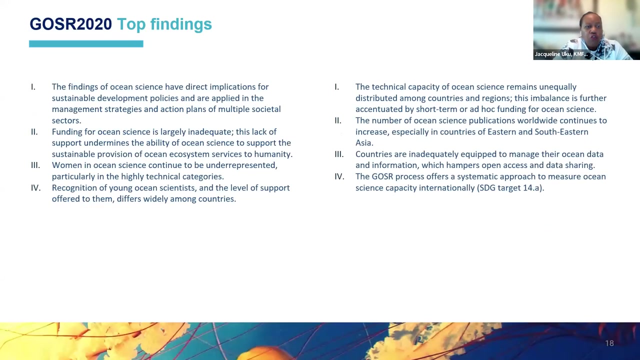 English, French and Spanish: Next slide. In addition, we also tried to push to get views and inputs from various focal points. We had a conversation with a number of Member States, we had interactions with IOC chairs and vice-chairs, and we also gave presentations at various IOC sub commissions. 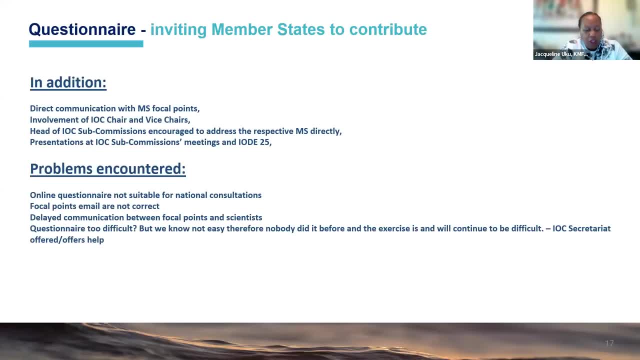 just to be able to put information forward. But we had challenges. The journey was not without its problems. Many countries found it very hard to input onto an online questionnaire platform. We found that focal points that were required to give us information had incorrect information on email accesses. We had delayed communication. Some found the 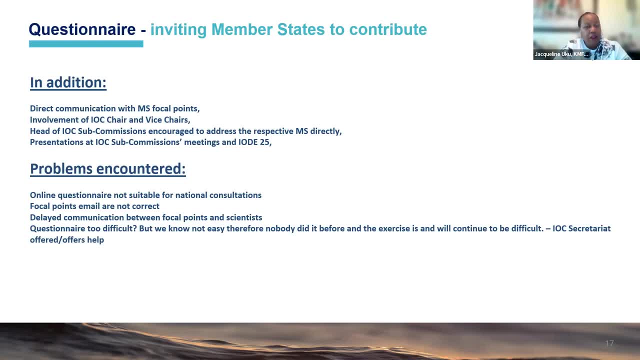 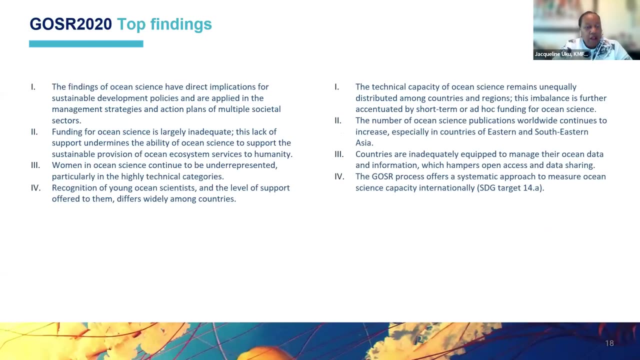 questionnaire quite difficult, but it's an exercise that we are reviewing and will continue to pursue, even as we update the report with help offered through the Secretariat. Next slide: Now we had some top findings and I'll elaborate some of them, And I'd like to just emphasize that. 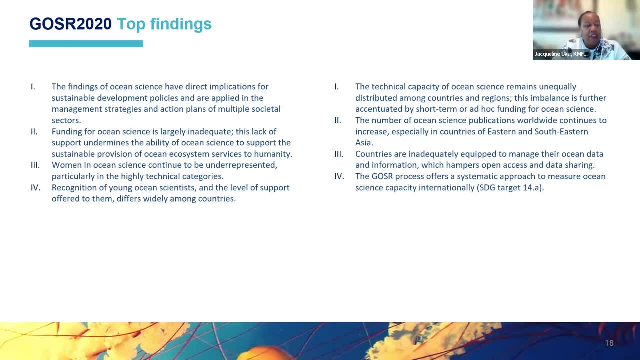 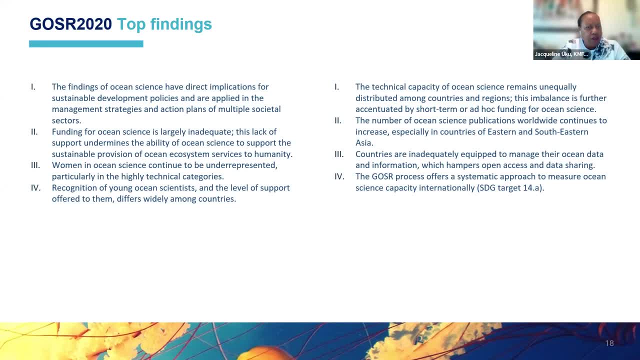 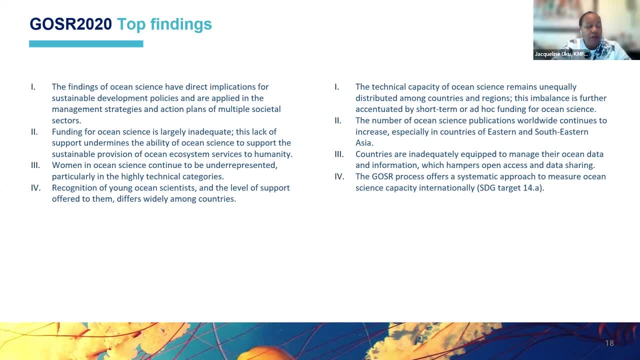 can be applied to management strategies and action plans in several sectors, not just the ocean sector. We found that funding for ocean science in Member States is largely inadequate. uh, we found that women in ocean science continue to be underrepresented, particularly in technical categories. we also learned that there is recognition of young scientists and the level 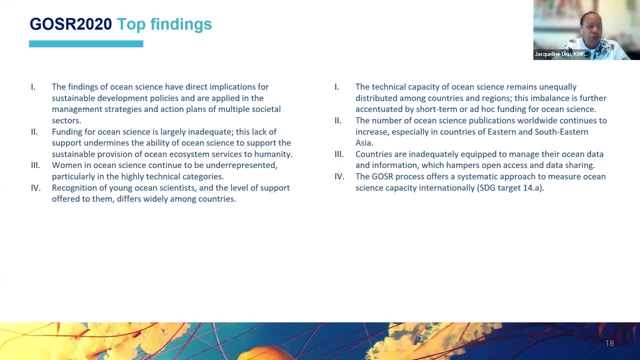 uh offered of support offered to them to grow their careers, is widely uh differential between countries. we also found that publications worldwide continue to increase, especially in eastern and southern asia. in africa, our publication level is still has not met the global threshold. we found that uh in terms of ocean data, which is critically important. 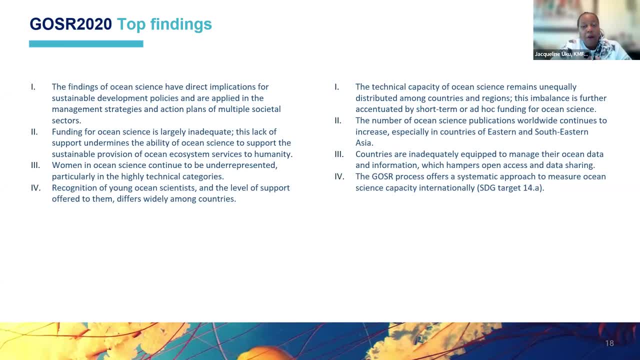 uh for the safeguarding of our oceans. um we are in countries are inadequately equipped to manage uh the data, to even obtain the data, and there are also uh critical issues around open data and data sharing. and so, um stg14a, which is uh mandated to ioc, unesco, um and put the geo global offering. 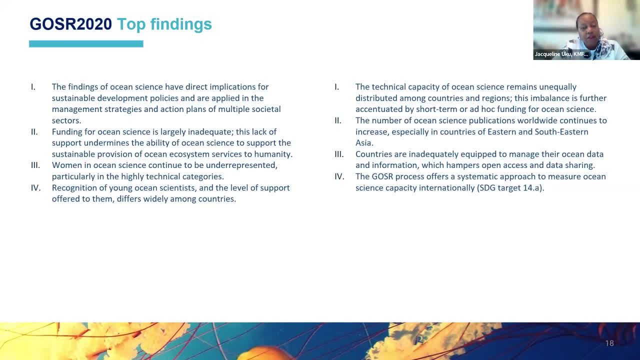 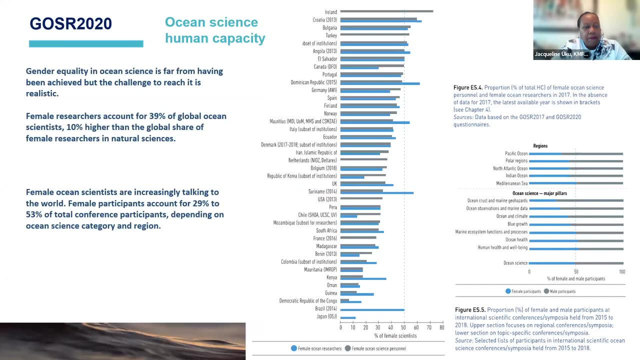 science report forward as a process that can systematically assist us analyze and understand the status of our ocean science data, both to stakeholders and stakeholders now. so the in our our contribution to ocean science, which is critically important for us to move forward next slide. so here we look at human capacity and the report has a very beautiful and concrete data sets that 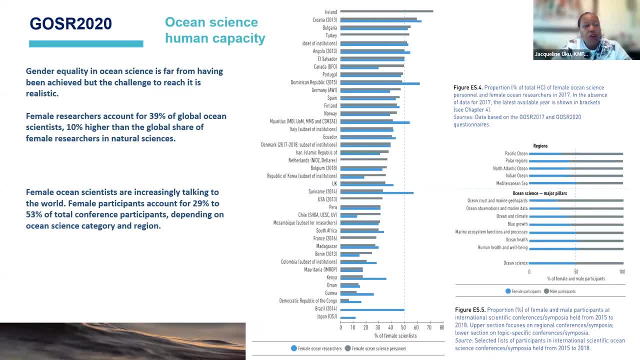 can be used for decision making, and we found, as i said earlier, that gender equality is far from being achieved. female researchers account for 39 percent of global scientists, but what we found that was very interesting is that for ocean science, this was 10 higher than the global share. 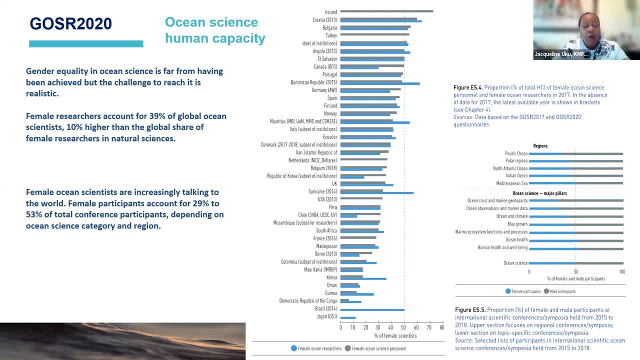 of female researchers in natural sciences. we also found that women are participating in conferences. they increasingly talk to the world and in any given conference, we'll find at least 29 to 53 percent of uh participants being female within ocean science categories and also within the regions. next slide. 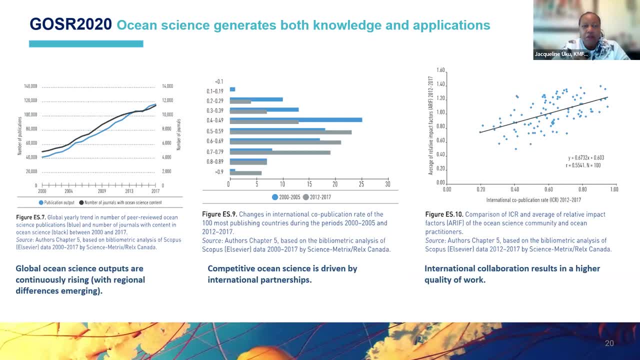 we found that ocean science is important because it generates both knowledge and application. the outputs of science are increasing both across the world. competitive ocean science is driven by international partnerships. so there is a trust to create a fruitful partnership, significant and strategic partnerships to be able to drive ocean science. and we also found that international collaboration 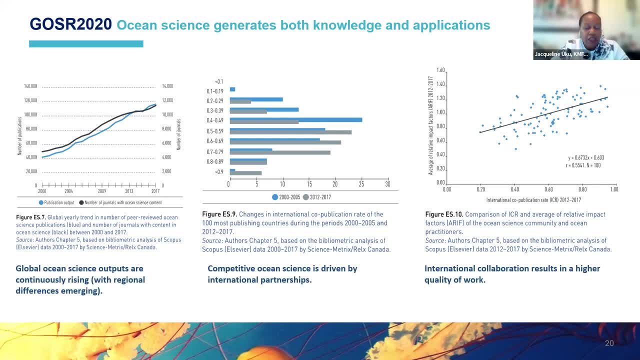 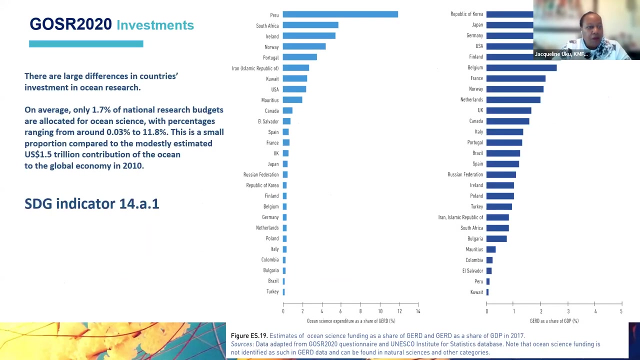 has driven a higher quality of work, especially in countries that and do not have traditions of ocean science or are growing that capacity. we found that collaboration is vital in uh just growing capacities within nations, especially in africa and the island states. next slide, in terms of investments: how much is our governments? 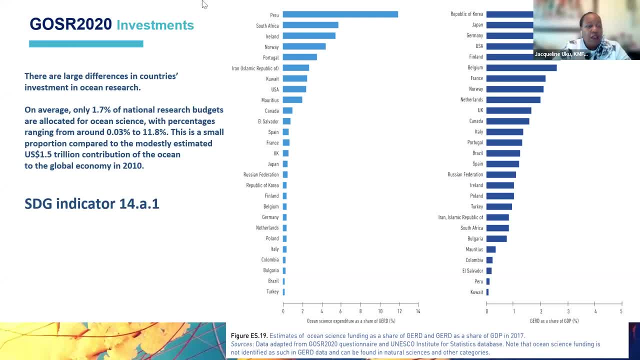 contributing to ocean science in terms of their budgets and, on average, only 1.7 percent of national research budget are located to ocean science, and the percentage could go as low as 0.03%, which is really small compared to the 1.5 trillion us dollars that the ocean contributes to. 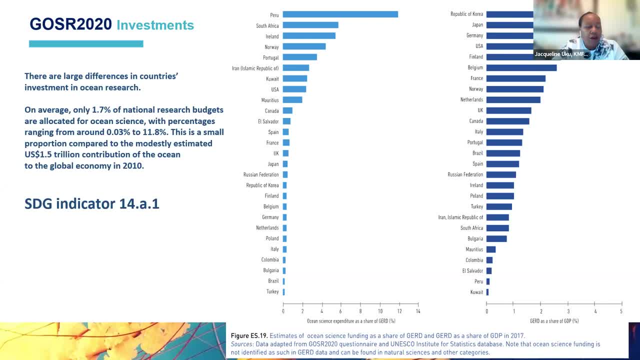 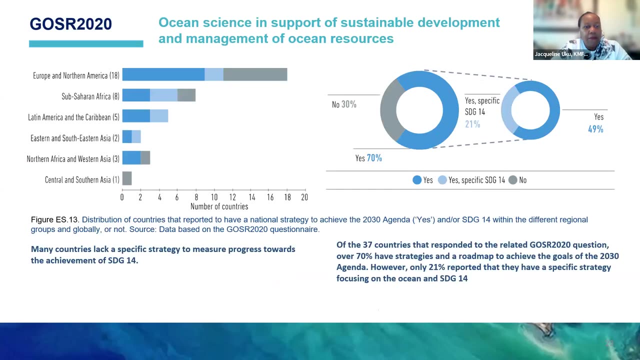 the global economy, and so that also shown a spotlight on how much more we need to do to push nations, push governments, to contribute to ocean science from their own budgets. next slide um that, in terms of strategy, many countries do not have a specific strategy to measure the progress and the achievement of sdg 14.. many countries talk about blue economy, but 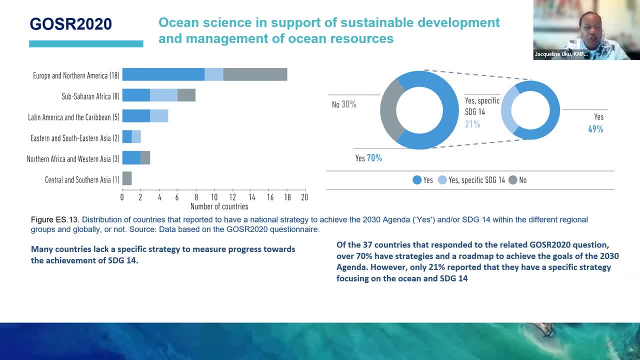 lack a blue economy strategy, which is part of this dialogue, and that then means that we are not sure which direction nations should take in the absence of strategic alignment and visions. to that target the ocean. we found that, uh, 37 countries that responded to this question, um, some have a roadmap, but um only 21 reported they have a strategic document and a strategic 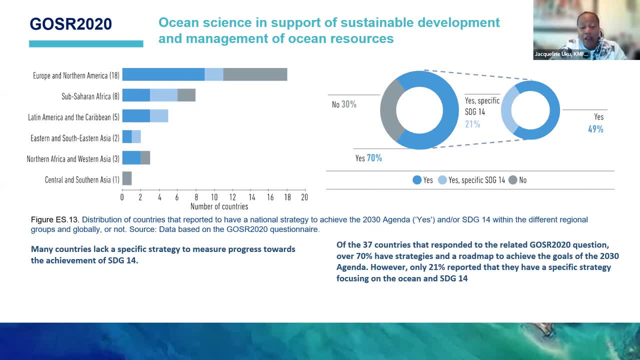 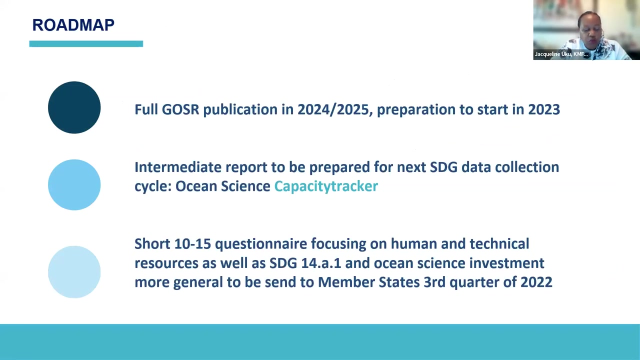 approach, and also not only that uh strategic approach, but a department, uh or a ministry that is focused solely on the achievement of the ocean, of ocean-related goals: SDG 14, and the blue economy. Next slide, We have a roadmap. Those are just a few results. 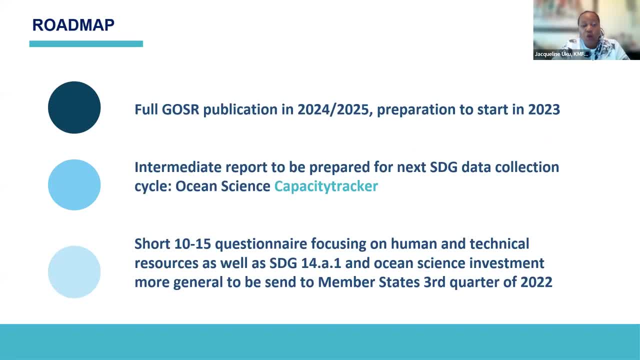 The report, as we indicated earlier, is full of weighted results that are very critical in helping us understand where the gaps are within our nations, And we are beginning to prepare for the next stage of this report. Remember I said it is a baseline and our preparation will begin next year. 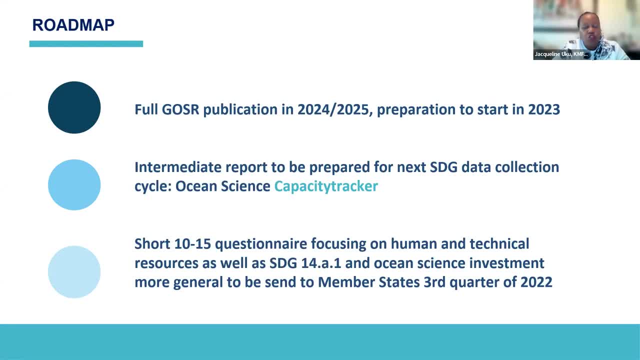 And we would like to continue to track how much ocean work, how much ocean contribution governments are putting in to the dialogue. We will also have a short questionnaire focusing on human and technical resources. This will be sent to member states in the third quarter of 2022.. 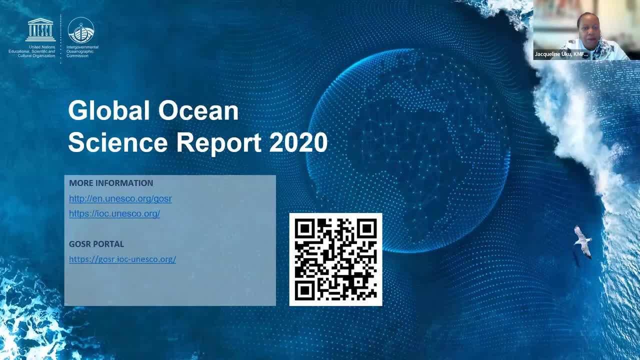 Next slide. So this brings me to the end of my presentation. I would love to share many of these results, and we've been sharing them over the past year, since the report was launched in 2020,. and having dialogue on critical aspects that we need to look into as member states of IOC UNESCO. 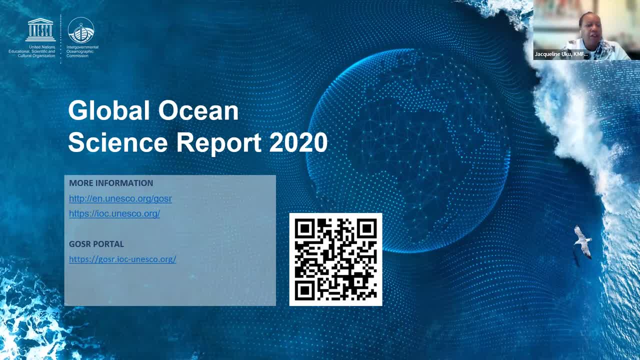 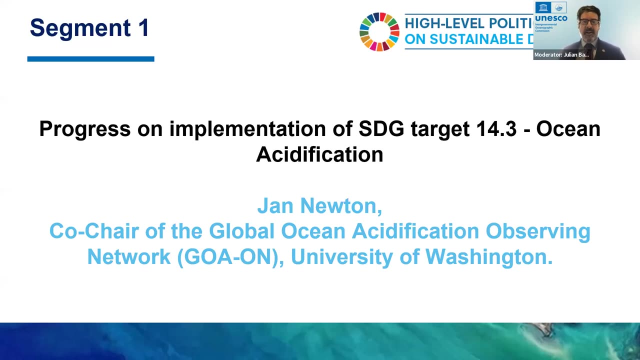 and also as global partners in this journey. So thank you, Julian, for the opportunity I'd like to hand over to you. Thank you very much, Jacqueline, for giving us an overview of this very important report and how it really provides a snapshot of the you know. 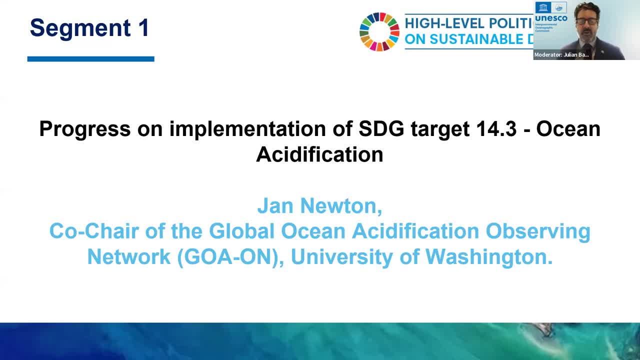 how you know, capacities are distributed around the world, but only but also how science is also being used to support sustainable development very concretely, and i think the message is clear is that the the capacity of countries to to to implement sustainable strategies is also very much. 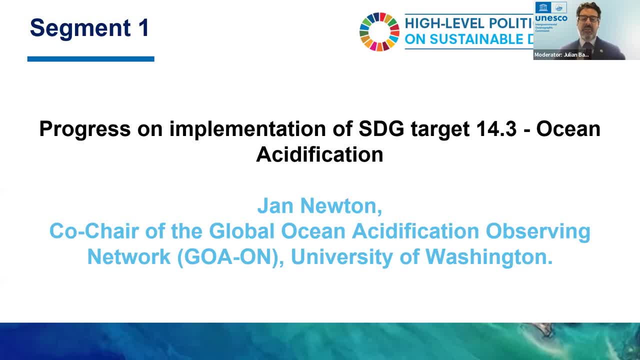 interlinked to their own scientific capacity at the national level. so, uh, some very important messages as well for for the future. uh, thank you very much. we'll move now to uh john newton, who is going to talk to us about the sdg target 14.3, which is focusing on the impacts of ocean. 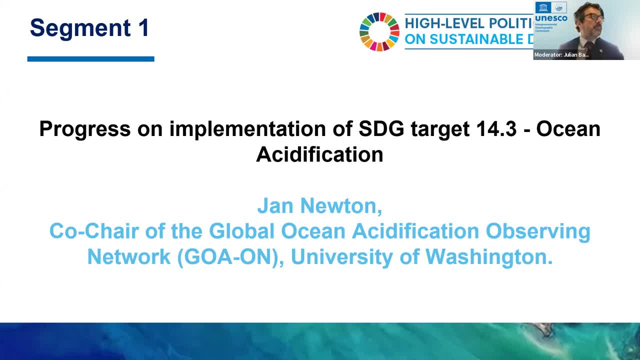 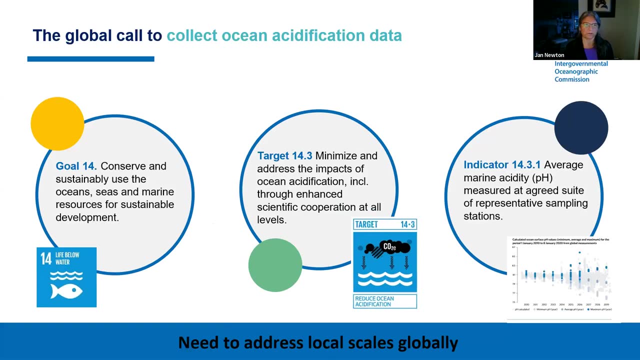 acidification john over to you. thank you very much, julian. it's my extreme pleasure to be here. it's an honor to be yet another spokesperson for the ocean. thank you to all those attending, and so what i'm going to focus on after that wonderful introduction. 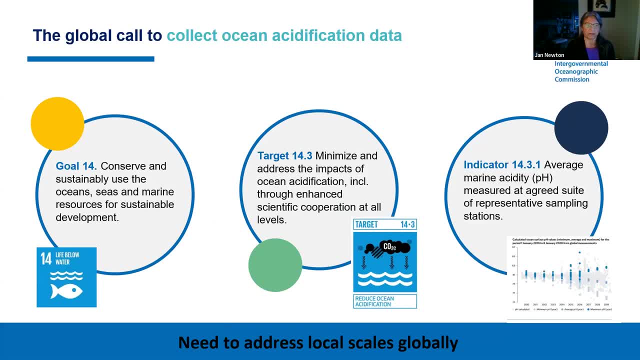 jacqueline is the. the target that is focused 14.3 within the goal of 14, to minimize and address the impacts of ocean acidification, including through enhanced scientific cooperation at all levels. the indicator for this has been chosen to be the average marine acidity, or ph. 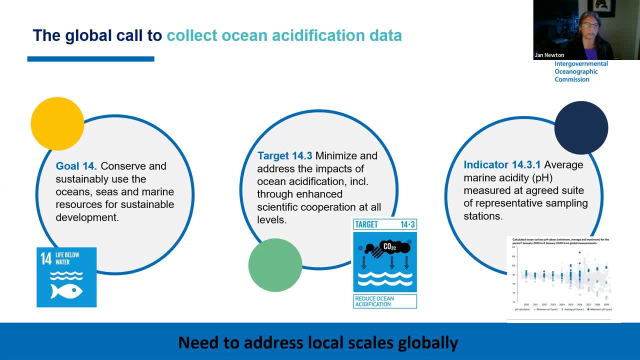 measured at agreed suite of representative sampling stations. so we have a global call to collect ocean acidification data that can support this goal, and what i'd like to do is talk to you about the progress on that, but also, to frame it, that we need to address the local. 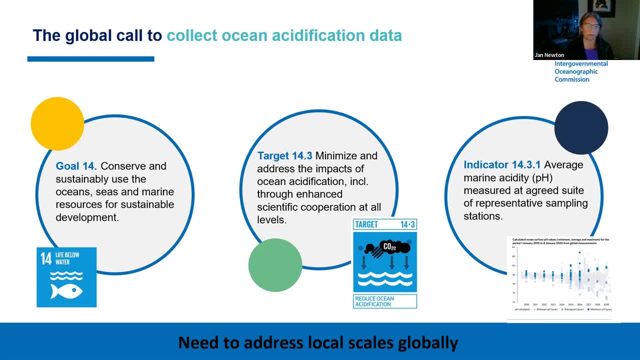 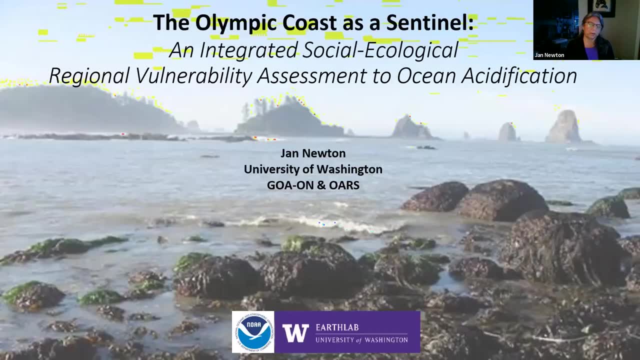 scales, on a global scale, in a global manner. so, to start that next slide, please. i'm going to share with you a story from some research that i'm actively involved with out of the university of washington, funded through the united states noaa national oceanic and 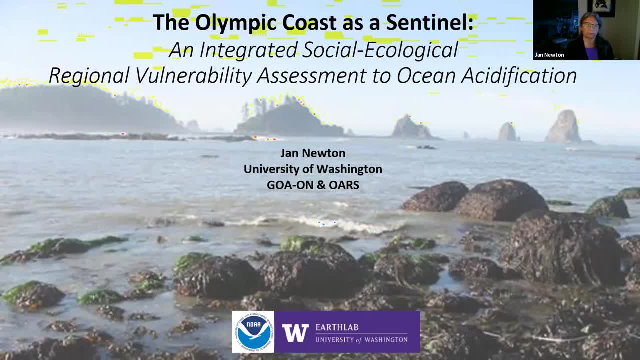 atmospheric administration, which is a regional vulnerability assessment to ocean acidification. it's an integrated social, ecological look at that, so working with social and natural scientists, and it takes place on the outer coast of the state of washington- maybe many of you have not been there, but it has been home to four. 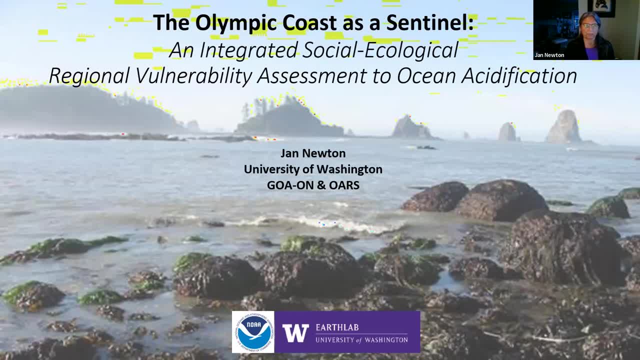 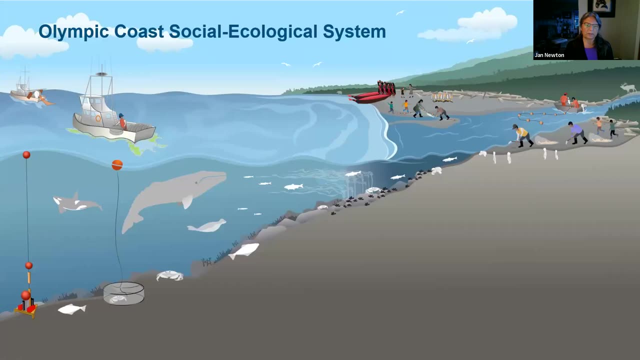 treaty tribes since time immemorial, and i think it paints a really important story of how these local stories are so important, and so i'm going to tell you a little bit about that local story. okay, so with the next slide, here is a schematic of the olympic coast social ecological system and 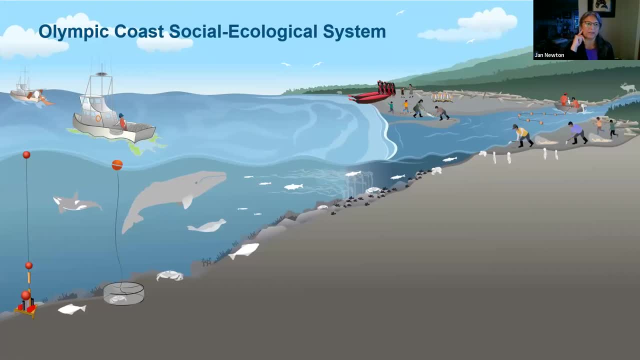 i'm a biological oceanographer, as i think of of an ecosystem. prior to this work, i'm also a geneticist and i'm a medical research associate of the ocean levels research and preservation and environmental and conservation team and, um you know, um i've been involved with. 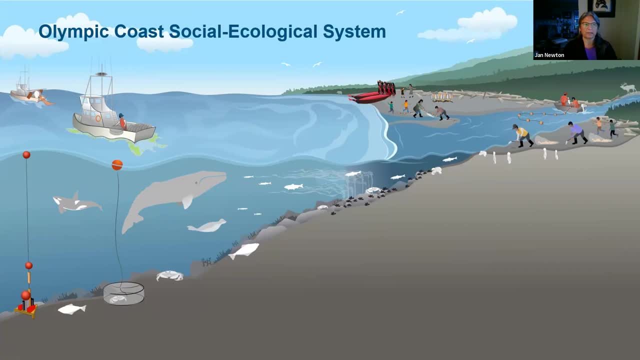 a number of the the ocean's, oceanic welfare programs and the oceanic way of the ocean, which is based on scientific research, and the oceanic. oceanic space is, and i'm really interested in the area of oceanic conservation and the oceanic region and the oceanic sand. 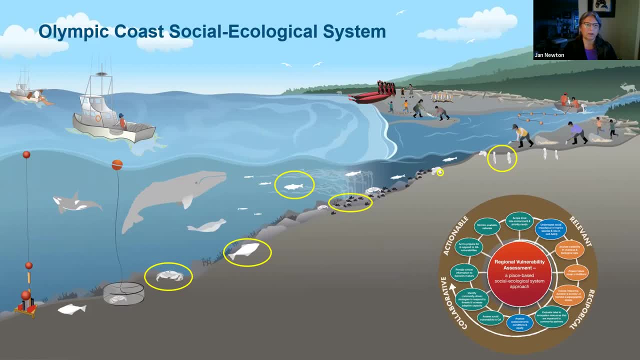 and what the oceanic ocean does to marine life. so i'd also like to talk a little bit about the oceanic species that were so critical for the sustainment of the culture And that little wheel that you can't see, but the different colors there represent social science steps, natural science steps. 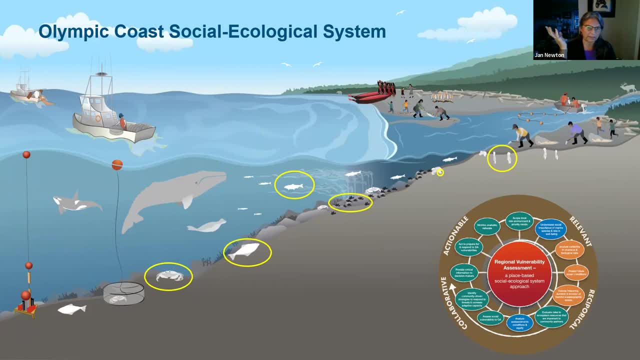 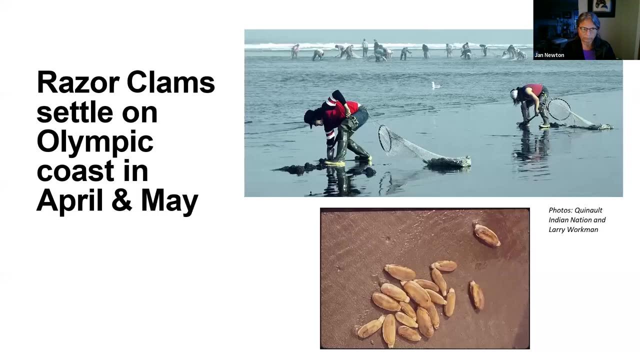 and together, working together to make this vulnerability assessment, And I can tell you what has come from this is some really important results. So, with the next slide, one of the things that emerges is the importance of one clam, a razor clam to the tribes. Obviously, that has been since time immemorial, But thinking now in terms of 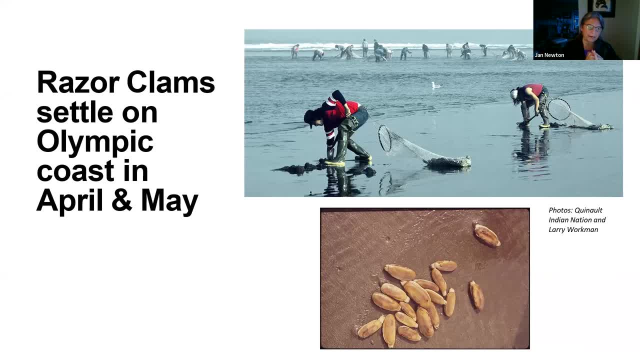 how do we make a scientific assessment? looking at when they settle in April and May and thinking about what are the conditions- things like aragonite saturation state that go even beyond pH- But help us to understand how this whole system is supporting this culture and the people who live. 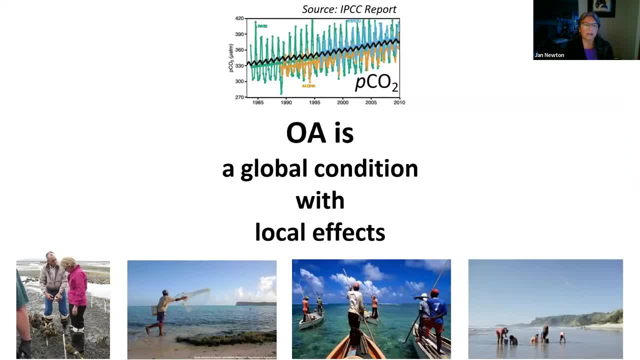 in it. So the next slide. So with that little example, I want to bring us back now to this global focus. And we know ocean acidification is happening on a global scale. IPCC reports for years, All the major basins are encountering this, But how it plays out on local shorelines with local cultures. Well, I'm going to go ahead and jump in here. I'm going to go ahead and jump in here. I'm going to jump in here. I'm going to go ahead and jump in here, I'm going to jump in here. So the 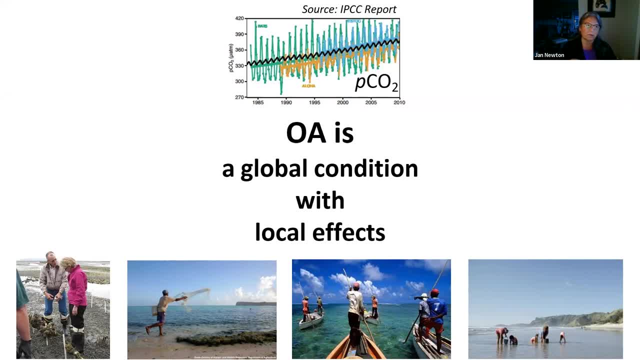 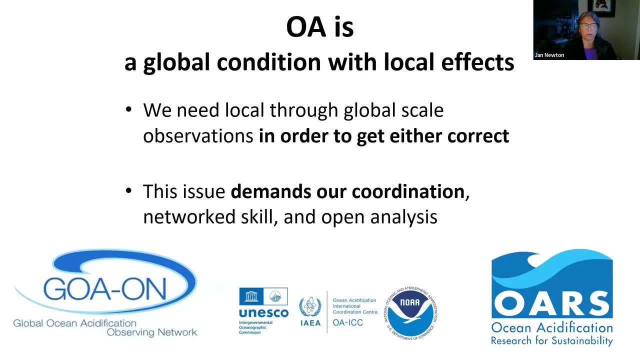 local species is very different, And also with how other things like nutrients or river mounds may be affecting the acidity of the water. It's really important that we think about the system. So with the next slide, I want to say that in order to understand the global 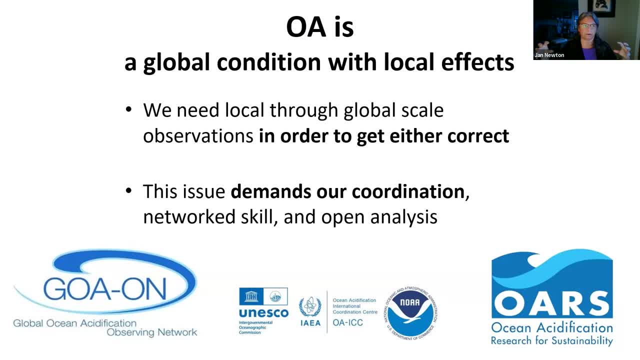 status. we need to understand the myriad of these local pictures, But also to get give the local pictures correctly, it has to be embedded in that global context. So we need both of these scales and we need to be able to integrate back and forth. That demands our 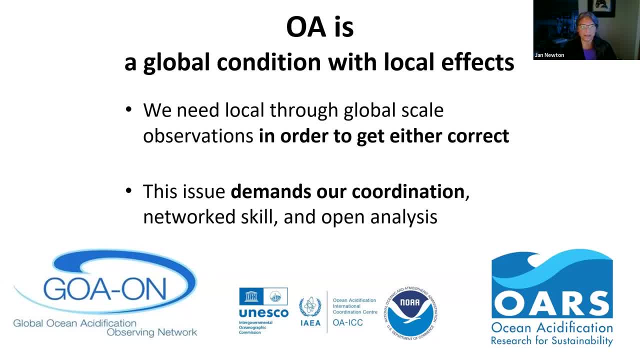 coordination, our network skill and our open analysis. And I want to give a big shout out to the Global Ocean Acidification Observing Network, or GOAN, and its UN-endorsed program, ORS that will work to coordinate these activities, And a huge shout out to UNESCO, IOC, IAEA. 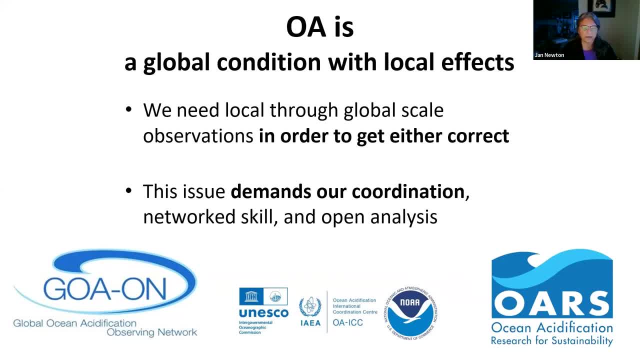 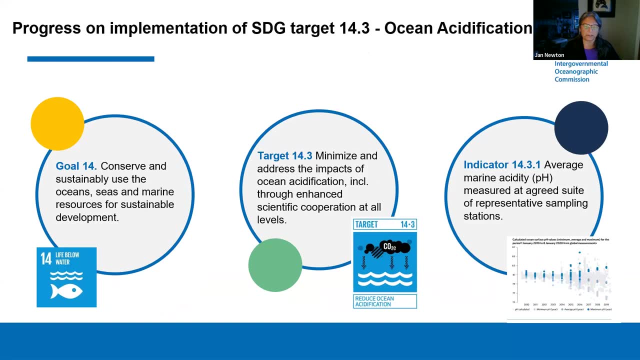 Ocean Acidification Coordination Center and NOAA, who have been supporting GOAN and ORS to try to achieve these results with the scientific community. So the next slide. how are we doing So? coming back to this initial slide and now focusing on the scientific community, we're going to talk a little bit more about the 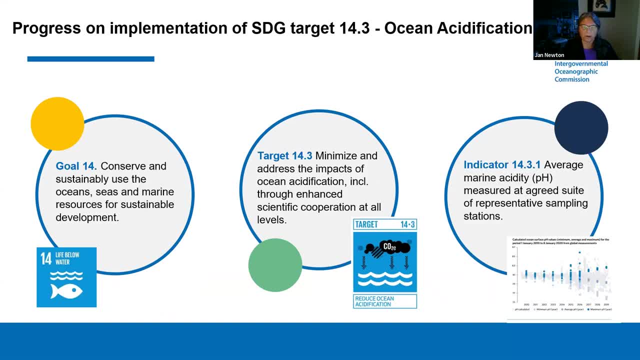 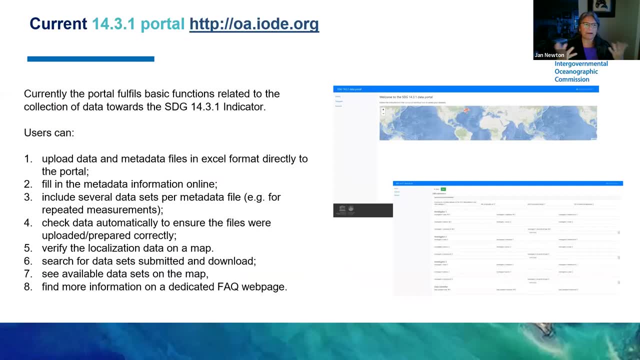 focusing on that indicator 14.3.1.. Where are we with that? It's a bit of a big lift, yes, And so what we needed to do is have a portal that will allow people to put data in The International Oceanographic Data and Information Exchange. IODE has that portal There. you see all the 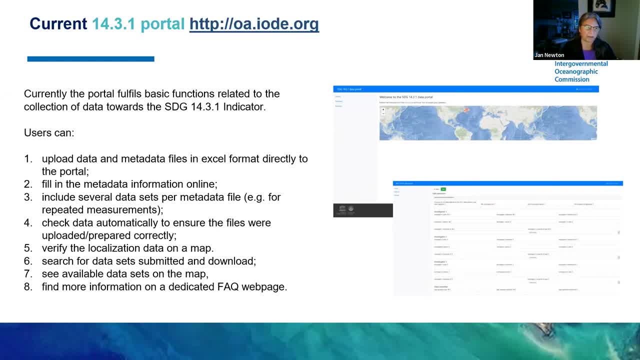 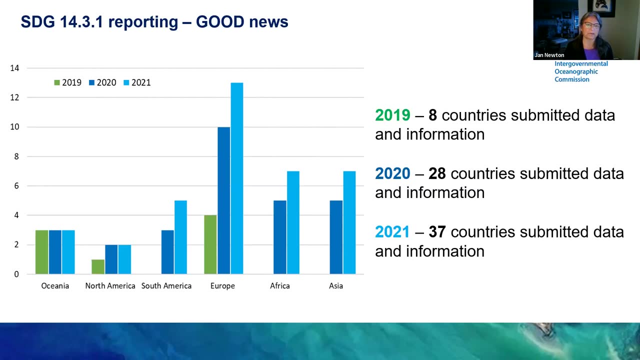 details of what you can do. So there's great progress on this data portal that has a lot of data. And then we have the data that allows the input of data. Next slide, And here's the good news: We are seeing growth in the people participating in the numbers of. 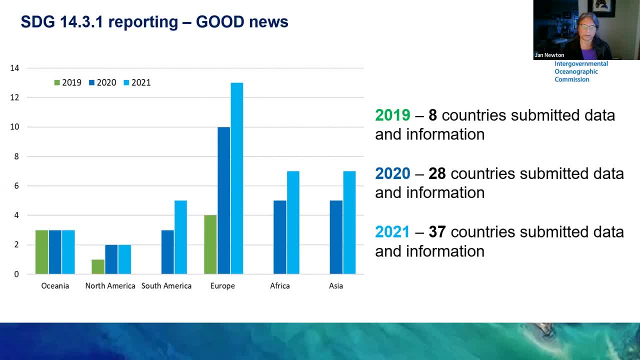 countries participating from 2019 to 2021, increasing from 8 to 37 countries. So 37 countries is good, but we know there's a lot more countries in the world, So we need to keep pushing harder And with the last slide, 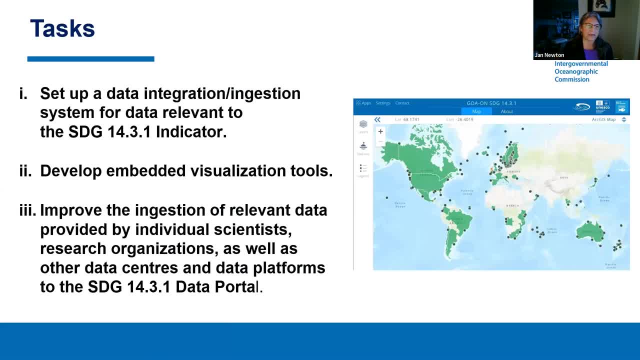 we want to reinforce some of these tasks that we have to go forward. We need to reach more people, more nations, and to make it easier for the on-ramping of getting those data on that local scale, And so here's an example of a visualization tool that GoLON is seeking to release soon: that 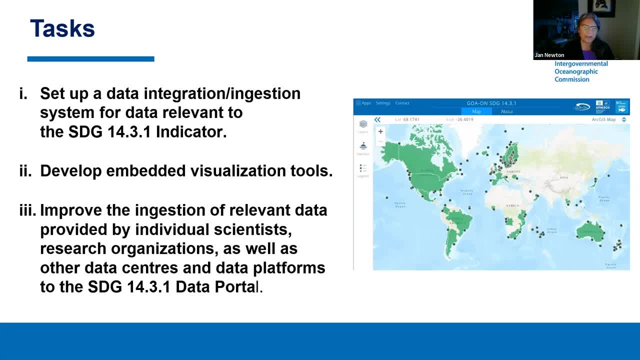 will help elevate- you know where the data are coming from- and to be thinking and working with the community, And so we want to reinforce some of these tasks that we have to go forward. We need to work with the community on how we really get the relevant data, how the scientists have the ability. 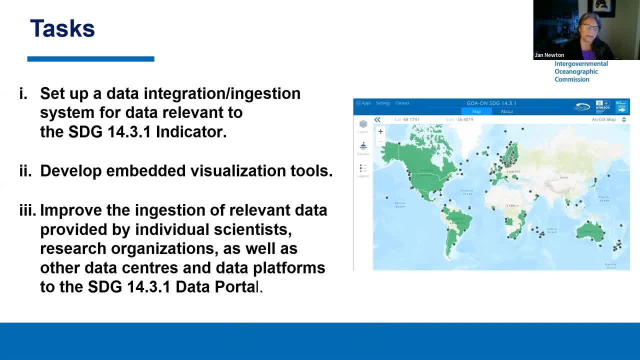 to put input on what its significance is. But, as I hope you've seen from that short little local talk how important it is that we get this right. So many cultures and people are depending on this, So we need to work hard to get this done. Thank you so much. 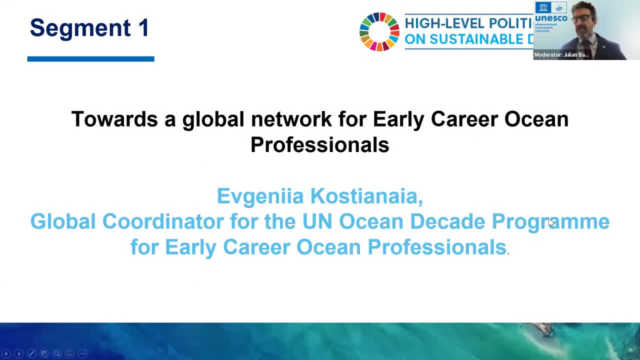 Thank you very much, Jan Great. So the message I get here, I mean first of all we need to, as you said, you know, also focus on the local scale, because we are talking about a global process But really local observations are so important- It needs to be really integrated. 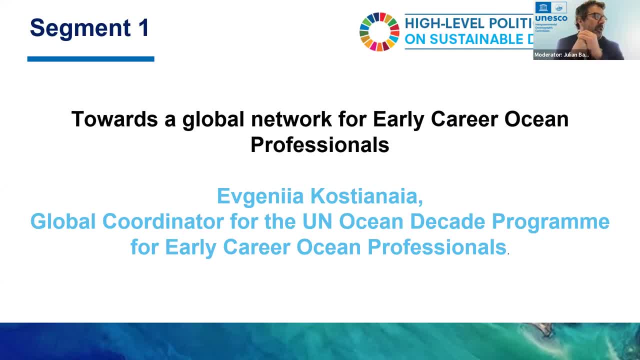 into that global picture. Very nice to see some growth in measurements of countries. We have 37 countries now reporting on these indicators. We have in the IOC 150 member states, coastal member states primarily. So I think we there's progress, but there's still a large 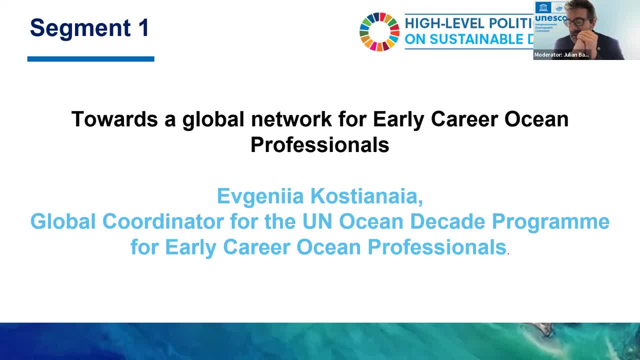 gap to be filled. And again, you know this, integration of data through different tools and also integration of different sources of data is very important. So thank you for that. I would like now to go to our last speaker for this first panel. 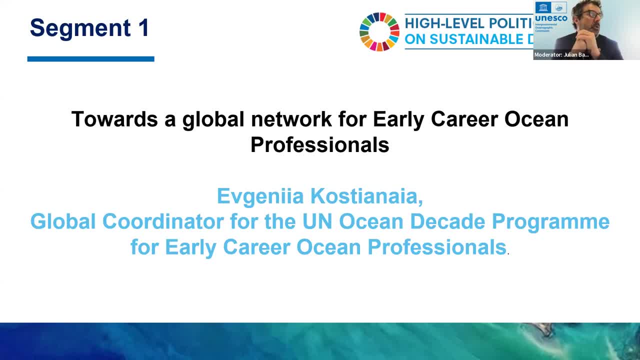 And this is Evgenia Kosianaya, who is going to talk to us about the importance of engaging early career ocean professionals in all this work that we are describing in research, but not only research. Over to you, Evgenia. Thank you so much, Gervin, And I would like to thank all the participants that are here today. 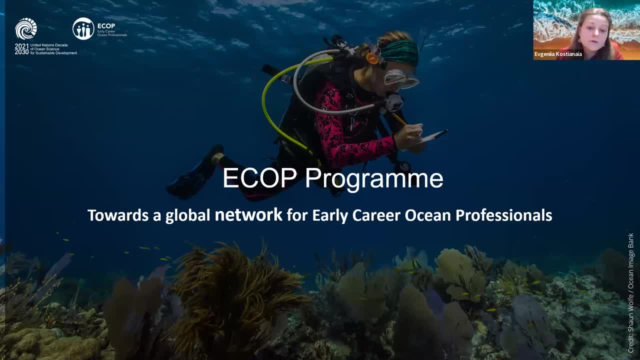 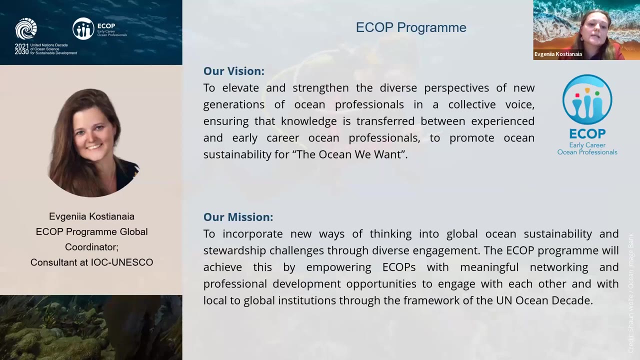 And I'm very happy to introduce the ECO programme and the work that we are doing within the programme for capacity development for early career ocean professionals. So we can start with the presentation, Thank you. So in short, yeah, I will just start with a brief. 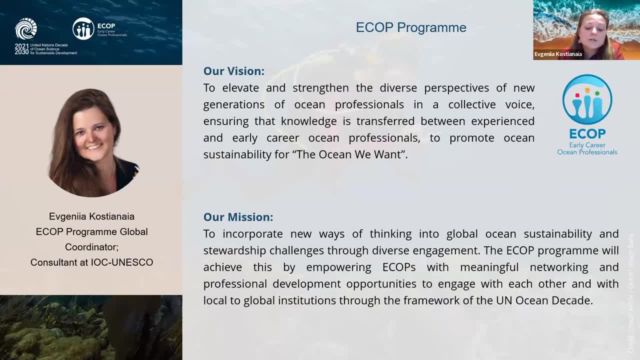 overview of what our aims are. So our aim is to elevate the diverse perspectives of the new generations of early career ocean professionals and to make sure that the knowledge and skills are transferred from experienced professionals to younger generations, to early career ocean professionals, And we are doing so by providing ECOs with meaningful networking opportunities and 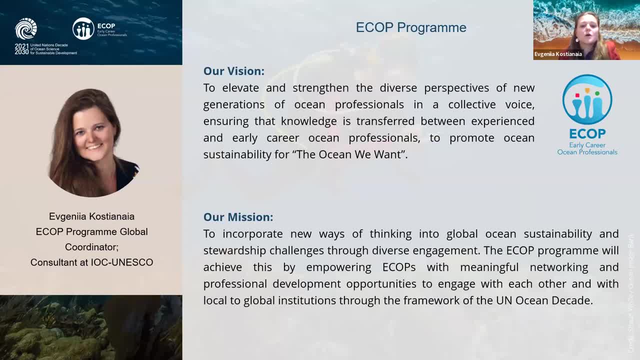 capacity development opportunities so that ECOs could engage with each other, both regionally but also globally, and not only among themselves but also with various stakeholders from local to global institutions. within the framework of the United Ocean Decade, but also the 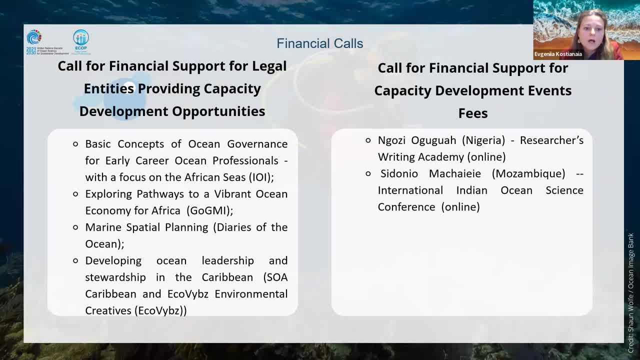 around it. Next slide, please. So we ran a global survey about two and a half years ago, And from that survey we found out that capacity development was certainly one of the top priorities for ECOs in any part of the world, So that was really one of the most pressing challenges. 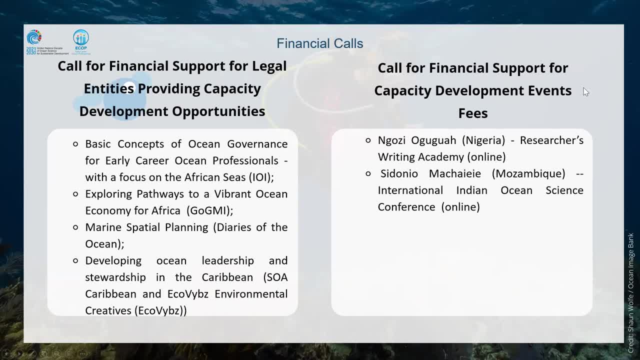 for ECOs. So this is why, with the, with our continuous work, we are focusing on providing capacity development opportunities for liquidation professionals. you were muted for a minute. yeah, just nothing. we can hear you now. yeah, sorry, okay. so, with the help of the IUC, UNASCO and, you know, region agency for development, 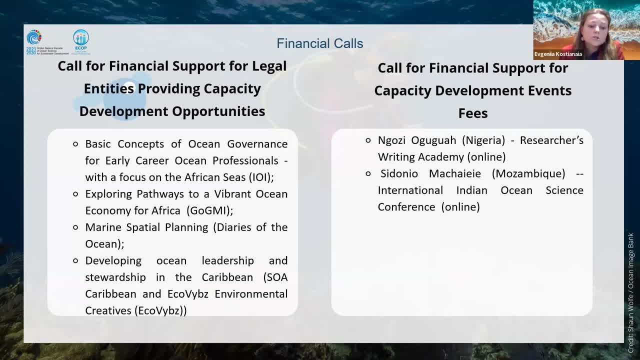 cooperation. we managed to launch two financial calls to support e-corps in their capacity development. so first call, the first call, was to cover participation fees for conferences or training opportunities. that was kind of individual support. and the second call was to provide legal entities or legal organizations who would provide trainings. those were online trainings. 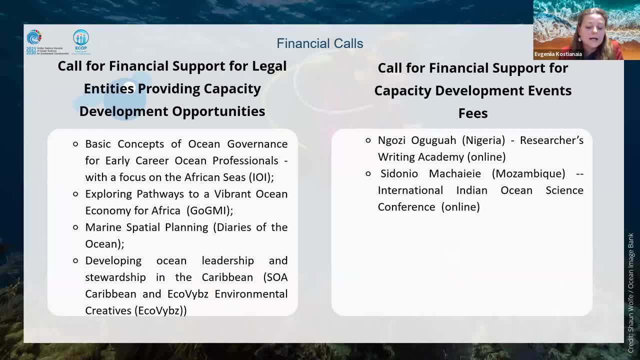 the focus was on the Caribbean seeds and Africa and the participation and those trainings were free for e-corps. so here on this slide you can see the titles of four trainings that happened this spring, and so two of them were in Africa and two of them were in the Caribbean seed. 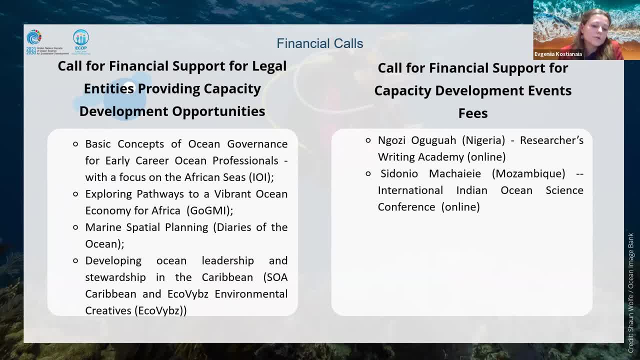 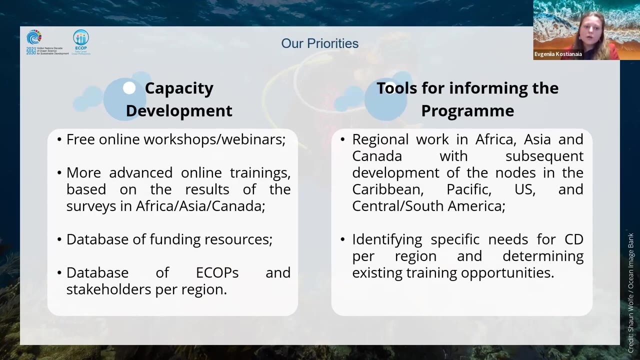 interesting was the example of theustering of the international impacts of the Что sus and there were very few trainings, that these trainings were focused on ocean governance and blue economy, so there were not purely like scientifically, let's say, on oceanography specifically. so they were very successful and we are planning to repeat them later this year and in the future as 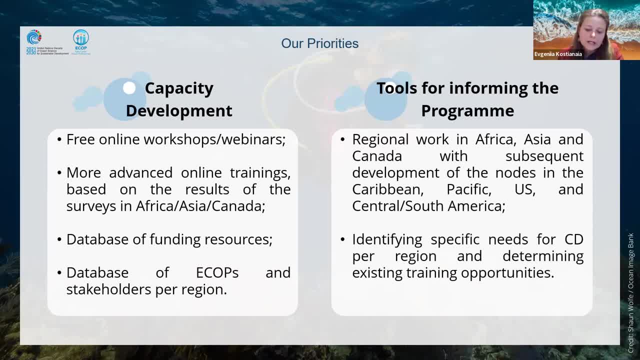 well, can we move to the next slide please? development needs in the regions, because capacity development needs with ECOPs vary significantly among regions, but also within regions, within a single region, so among countries. We started this work especially for Asia and we already see that capacity. 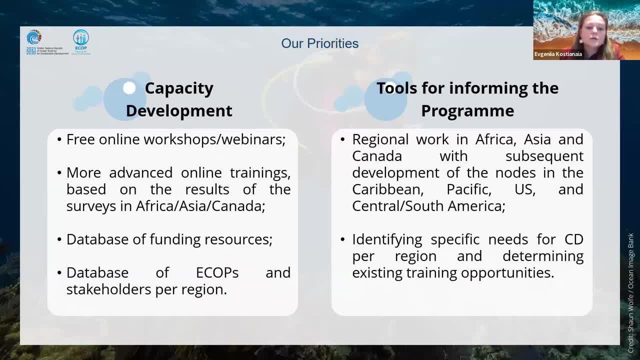 development needs are different there. So for some countries this is definitely the funding problem. For some other countries this is a language barrier, which is a tremendous challenge, And for some others still it is more about a lack of career development. 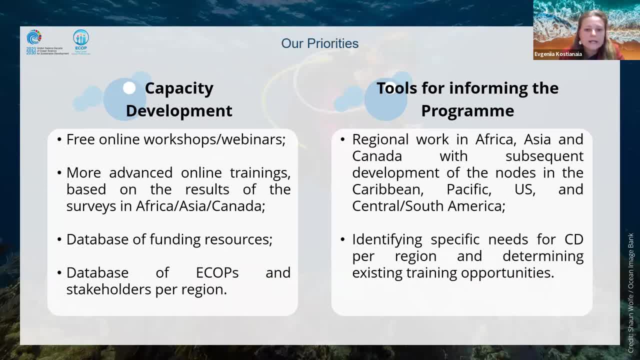 options. So currently we have regional coordinators working in Africa, Asia and Canada and we are planning to expand that work also for the Pacific region, the Caribbean region, US and Central and South America, where we'll And we'll continue to look into those details and these cultural and contextual differences. 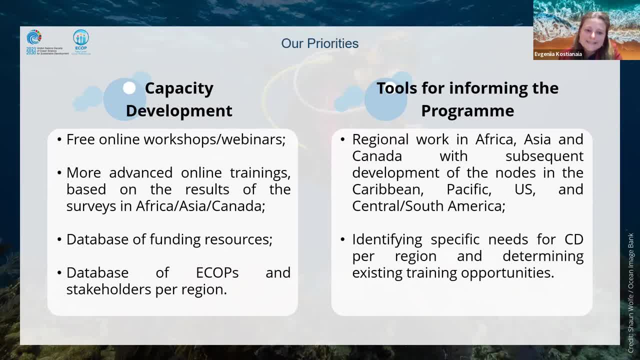 So we're also identifying existing training opportunities, because we do not want to reinvent the wheel or we just want to make a database where such training opportunities already exist and see what is missing and how we can address that with the help of the whole. 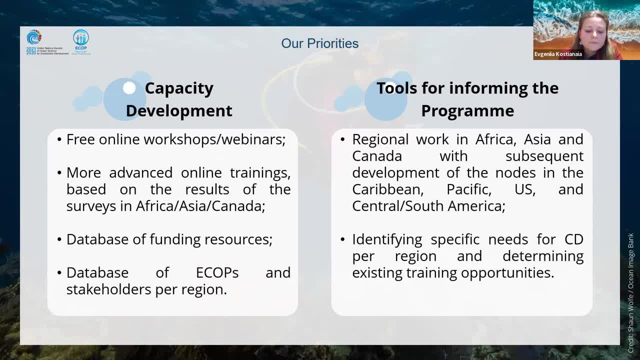 infrastructure of the UN fishing decade. So, I have already mentioned, we will continue with the online trainings that we started this year, based also on the feedback from the surveys that we ran also in spring this year in Africa, Asia and Canada. Then we will start with a series of free online workshops, webinars. so that would be. 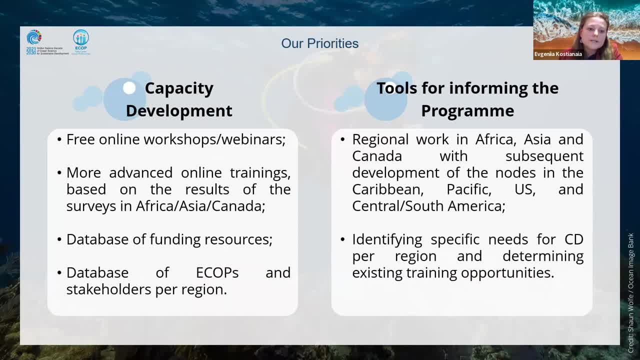 some really short, a couple of hours maybe- webinars that would mostly target not some scientific topics but rather interdisciplinary topics, because this is something that we continuously hear from ECOPs: that we need to more focus on interdisciplinarity. So things like science communication. 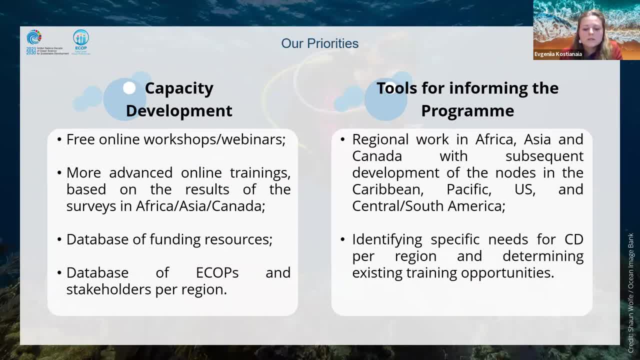 and how do you communicate your science to your audience, things like how to start an NGO or a startup in the environmental field. how do you find funding for your project? how do you switch careers? what should you do first? what should you do later? 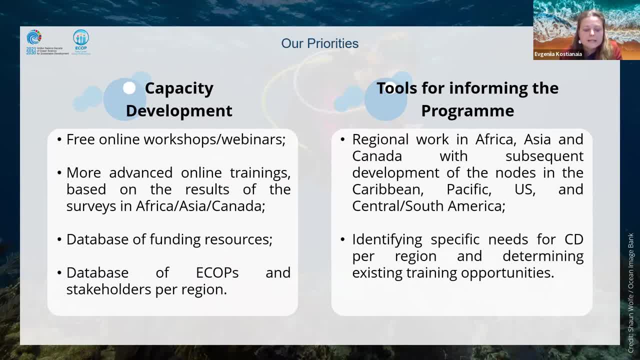 When you want to move to the marine related career at a later stage in your life- and we do think that this would be very important and interesting for ECOPs- Then we are working on a database for funding resources, which will be freely available on our website at ecopdkorg. 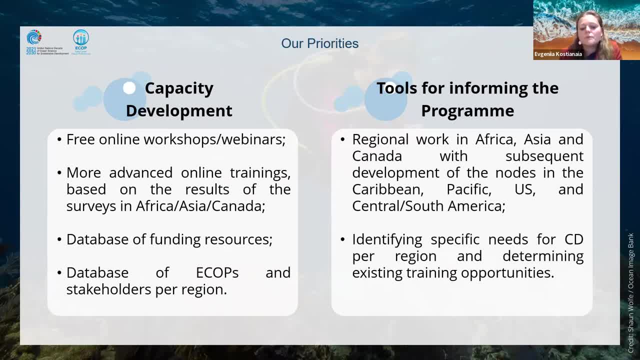 and again. we consistently hear that ECOPs do need more paid internships. they lack funding for going to conferences, fulfilling their projects, etc. So we want to combine all this information. There are various funders all over the world. it's just a matter of compiling this information. 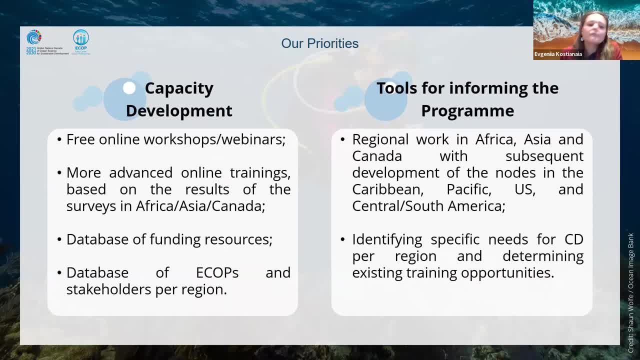 and making it easily available for ECOPs. We have also created a database for ECOPs for all over the world, and we are also mapping stakeholders per region, So this will help to easily distribute information for ECOPs about the developments of our program. 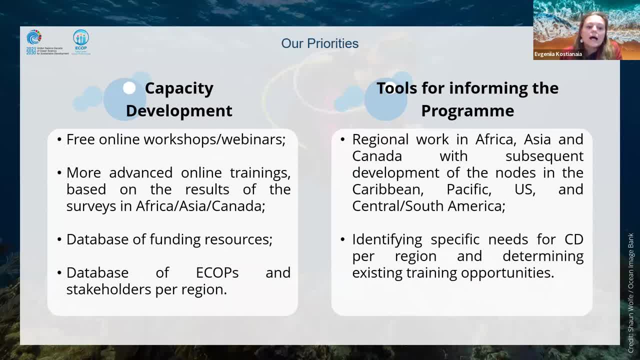 This database will bring together many stronals of the ocean decade and it will help connect ECOPs with various stakeholders- not necessarily academic institutions, because we want to think outside of the box and involve many other sectors related to the ocean. On. the next slide is just a compilation of our social media. 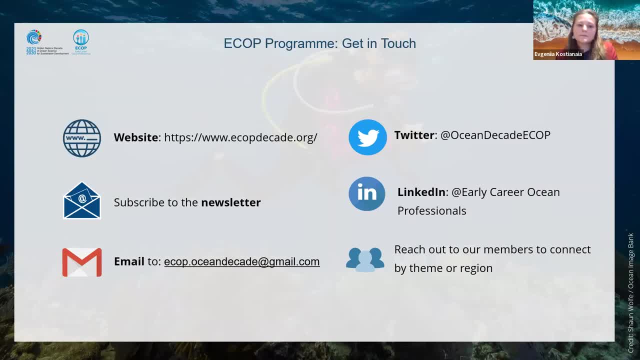 accounts and ways to stay in touch with us, as well as our website. Thank you very much, and thank you very much, thanks. thank you very much, evgenia. here we go. you've learned, uh, today a new acronym, e-cop, an important one. and, of course, if you are an e-cop, please do get in touch with evgenia, i think it's. 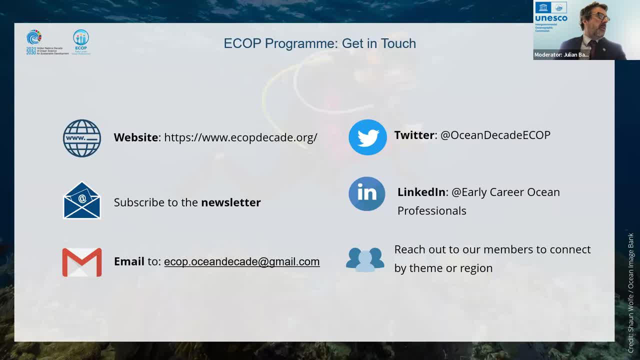 it's a great group and i was very happy to see many of the early career professionals with us in lisbon last week taking part in several events. and again, this is the beauty of this is that this is a self-driven group and and they are defining their own needs and we are trying to facilitate. 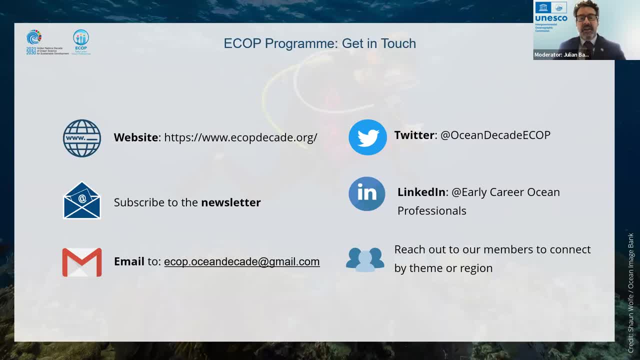 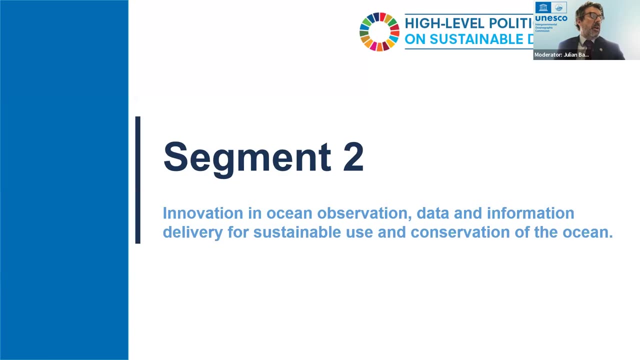 access to specific uh resources and collaborations. so with this um, we are not doing great on time, so i'm gonna. i was gonna open the floor for questions, but uh, just for equity and for our next group of speakers to have a sufficient time, we will move on to a segment, number two, which is focusing on 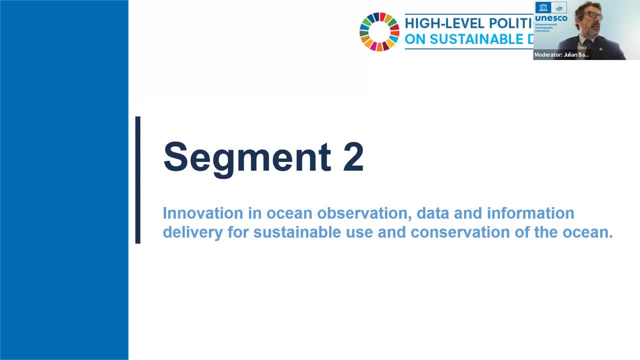 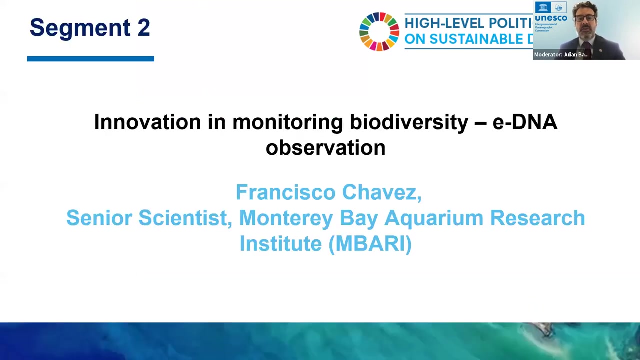 innovations in observations, uh, in in data and in information generation and in community-based management, and then, if we have a little bit of time and we can maybe go a little bit over the hour, we can take a few questions. so it's, then, my pleasure to invite our next three speakers, and those are: francisco chavez, who is a senior, 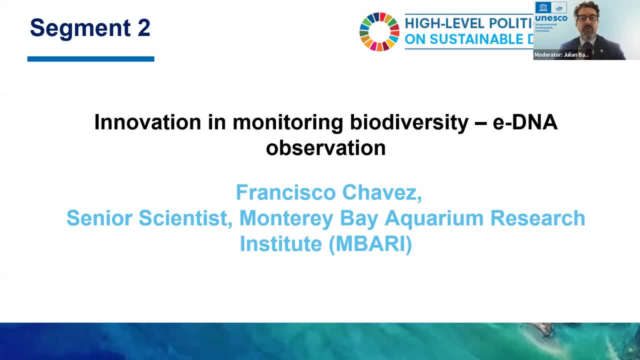 scientist at the monterey bay aquarium research institute in mbari, similarly to jan, is waking up in the middle of the night to join us. so so thank you for that. uh, we have also with us anya waite, who is the co-chair of the global 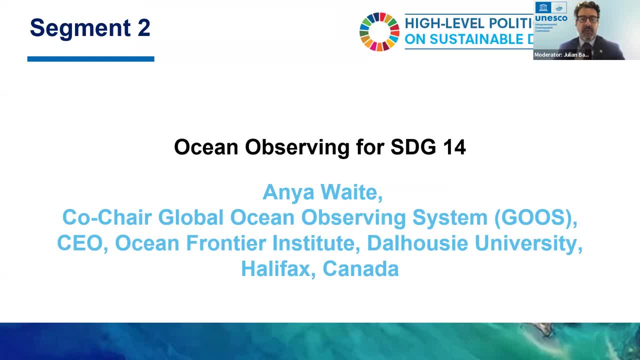 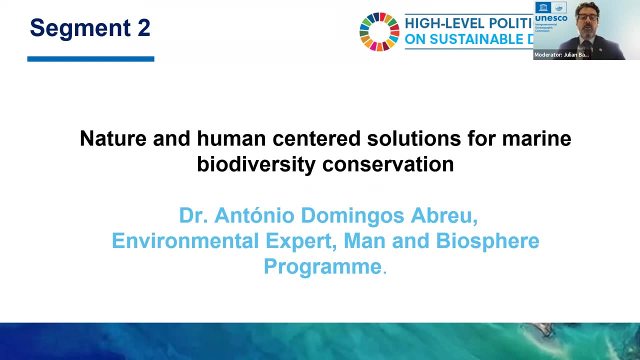 ocean observing system, and she is the chief executive officer of the ocean frontier institute at the lousy university in halifax. and then, finally, joining us from portugal, we have a pleasure of having dr antonio domingos amber, who is an environmental expert, also contributing to 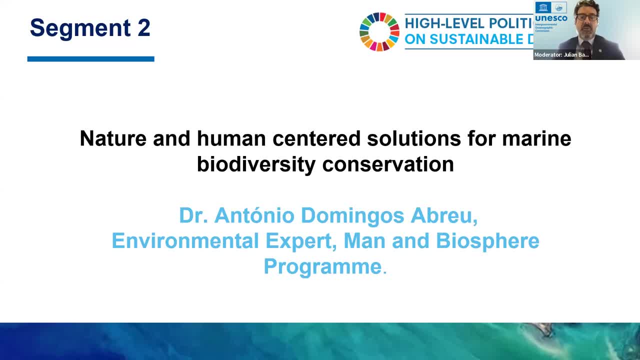 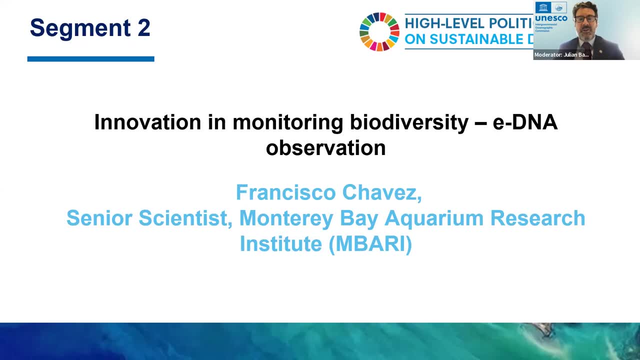 the unesco's work on man in the biosphere program. so let me then start uh straight into the next presentation and let me ask uh, francisco, to explain to us first of all, what is e-dna observation and why is it a such a novel approach to really understand the, the oceans, biodiversity. over to you, francisco. 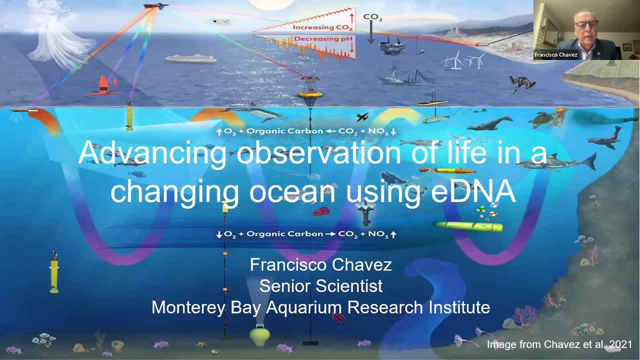 yeah, thank you for the invitation, julian. so we all know that the ocean is threatened in a number of ways. the uh uh global climate warming of course always has been, has taken uh most of the attention, but uh, the ocean, of course, is threatened in a number of of different ways. uh, next slide, please. 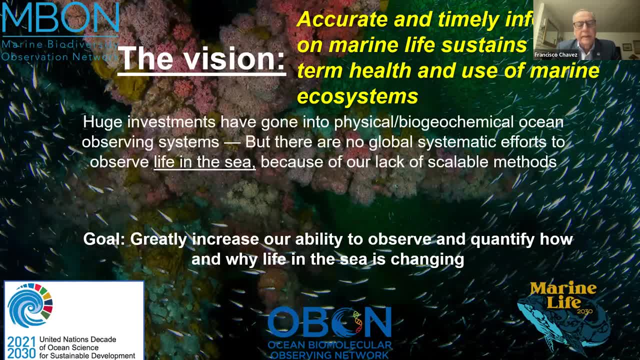 so, uh, i think one of our early speakers mentioned the importance of accurate and timely information on marine life, which really sustains the long-term health and of our world, and and we need to know it, uh, to manage it well, and we've made significant investments in physical and biogeochemical ocean observing systems. 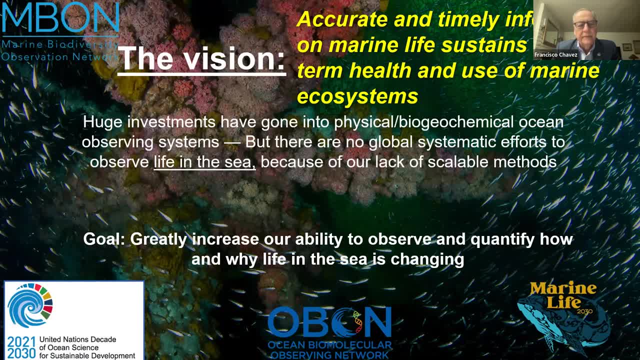 but today there's really no global systematic effort to observe life in the sea, and, and i would argue, that's because of our lack of scalable methods. so, uh, our goal is to greatly increase our ability to observe and quantify how life in the sea is changed. next slide, please. 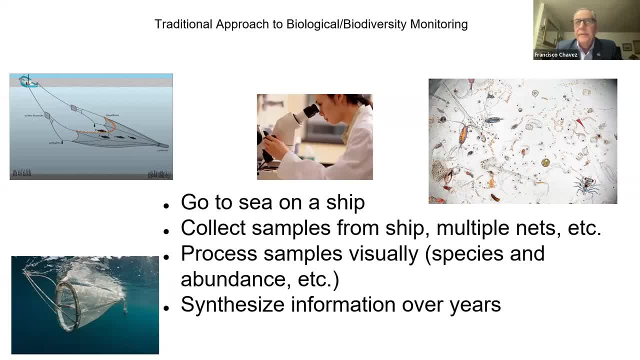 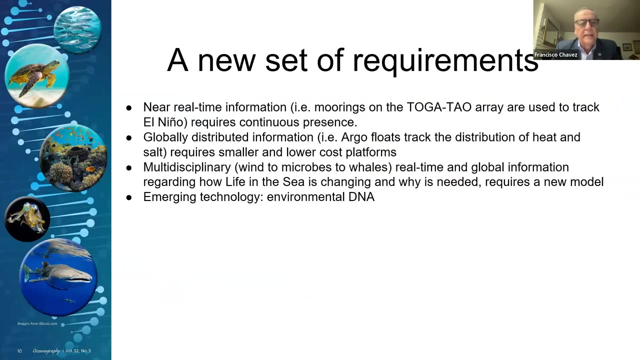 our traditional way of of monitoring biology or biodiversity in the ocean is to go to sea on a ship, collect samples using nets typically, process those samples visually and synthesize that information over years or sometimes even decades. next slide, please. we argue that, uh, there's a new set of requirements. uh, today we really need. 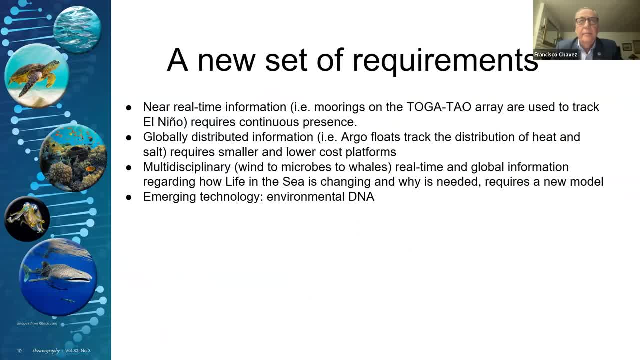 near real-time information, much like we get from moorings of the toga tau array. we need to have that information globally distributed, like we do from argo floats with physics, and we need that to be multidisciplinary. uh, we need to have this so we know how life in the sea is changing and why it's. 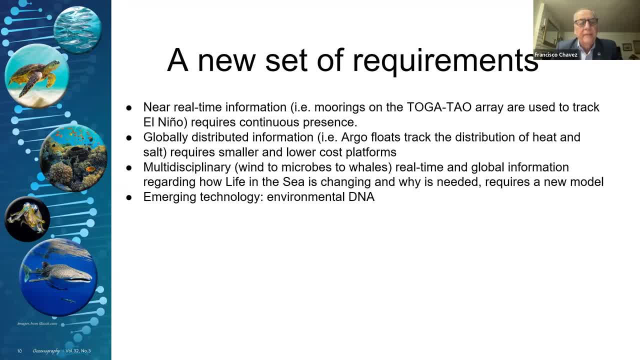 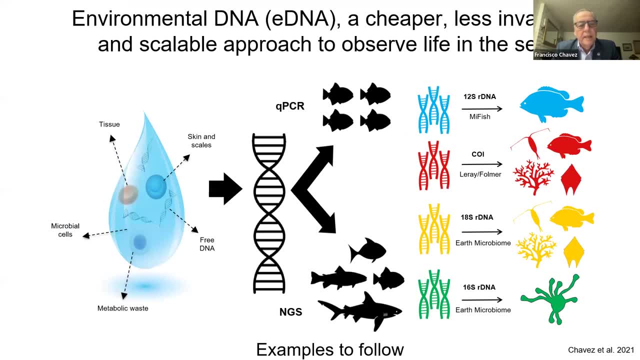 needed and that requires a new model and perhaps we have an emerging technology- environmental dna- that could help us with this. next slide, please. next slide, please. edna is kind of like forensic science: there's a crime, the crime scene investigator comes in, picks up residue used left behind by the suspects, analyze their, their dna content. 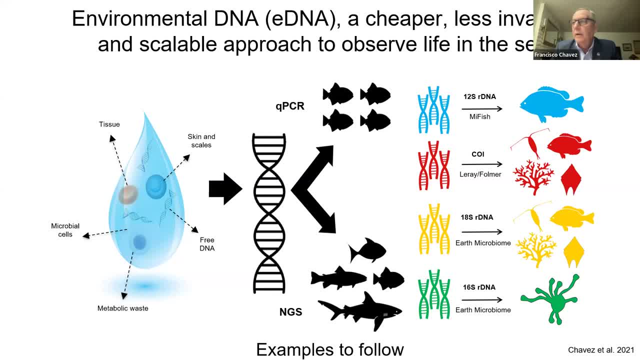 and matches it against the bank of suspects in the interpol or the fbi to identify the crime perpetrator. In our case, life in the sea are our suspects. We can collect water that contains living cells or residues of larger animals, analyze that eDNA and figure out who is left. 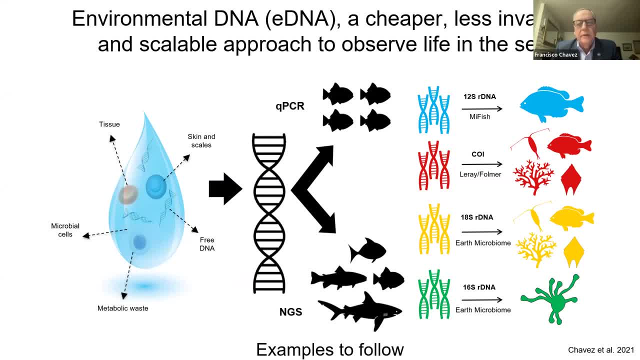 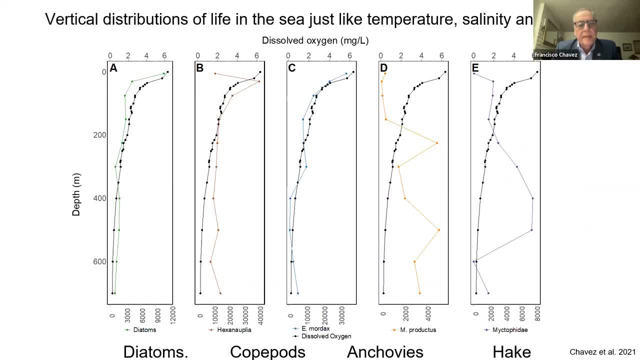 behind. We can target individual organisms or communities. I'll give you some examples of that now. Next, please- I apologize- for a little bit of science here. These are vertical profiles of different organisms, analyzed by eDNA, compared to the vertical distribution of oxygen in the ocean. 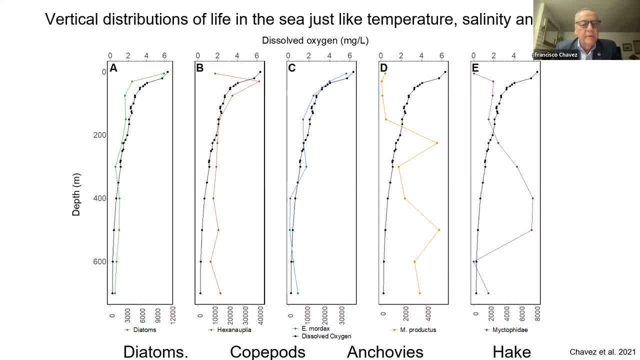 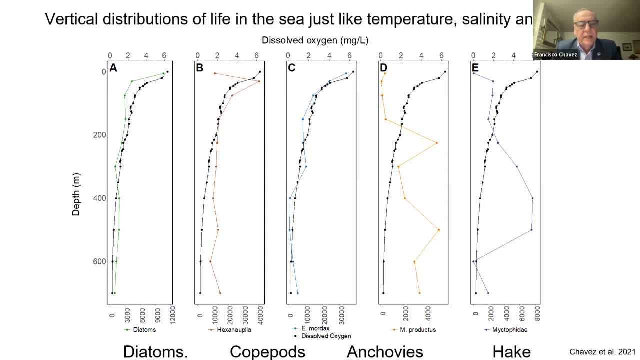 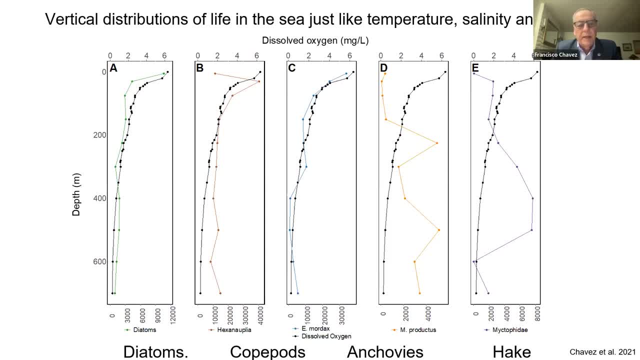 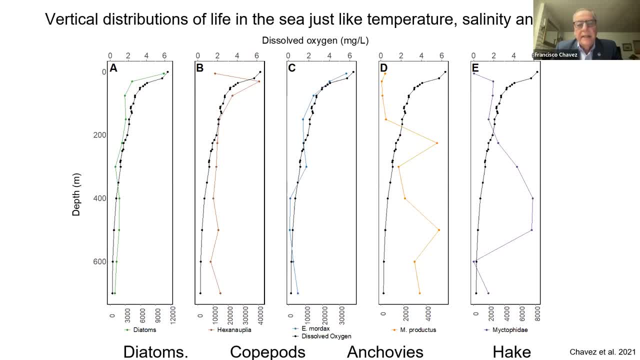 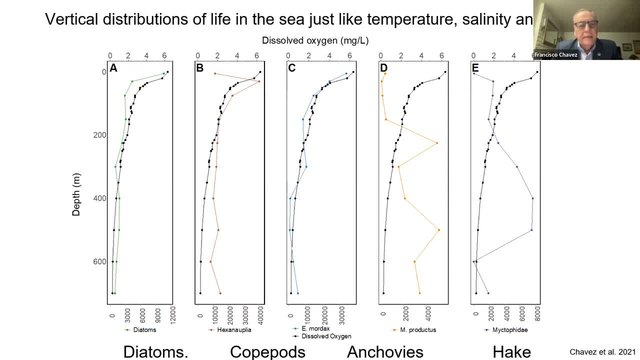 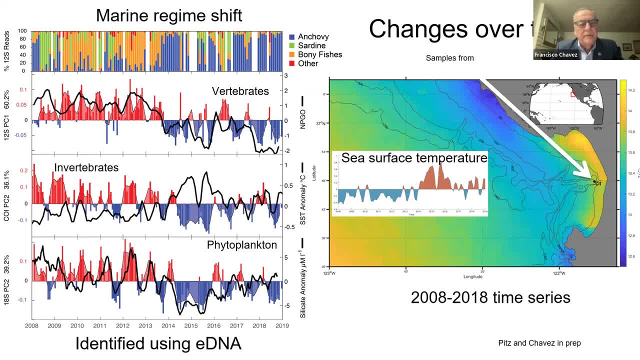 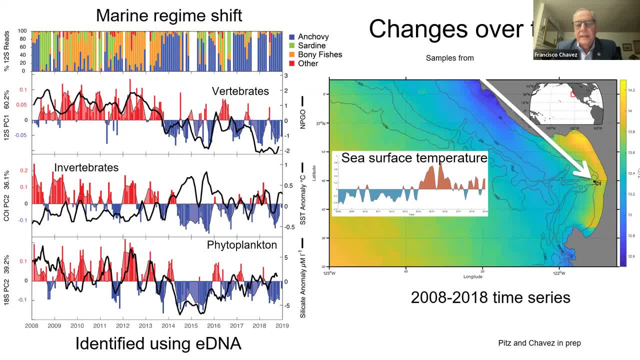 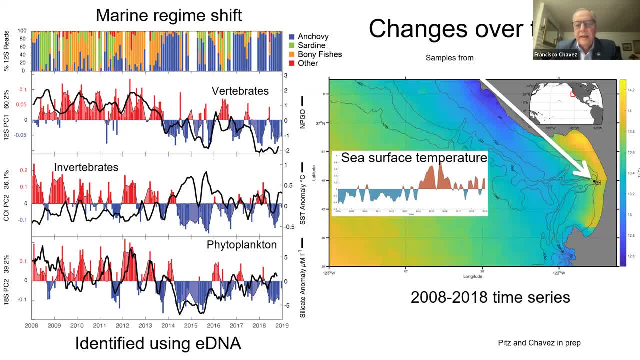 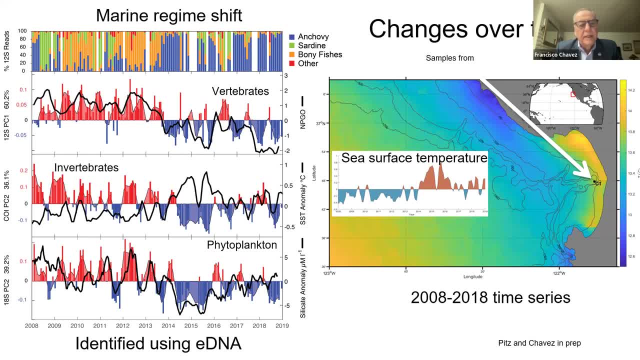 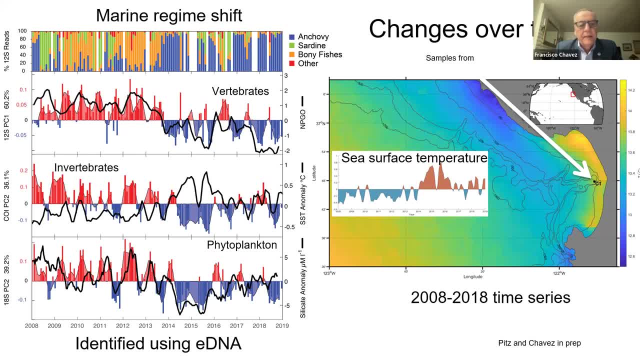 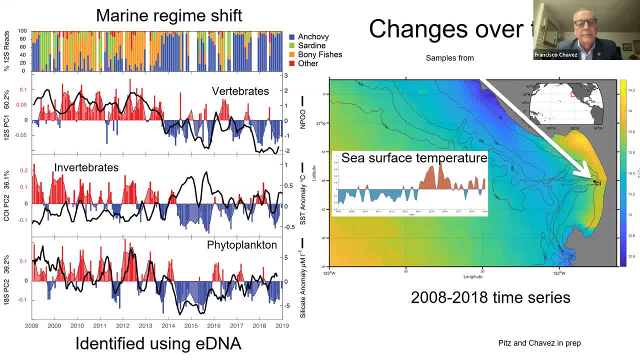 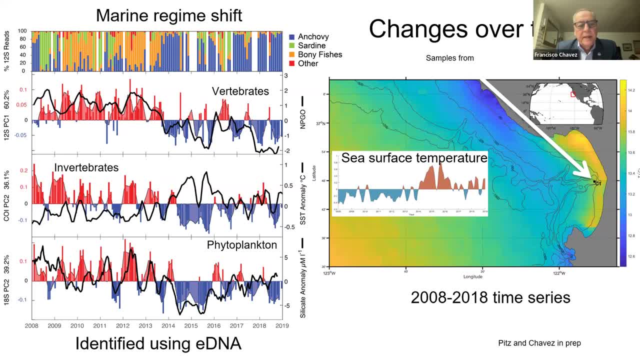 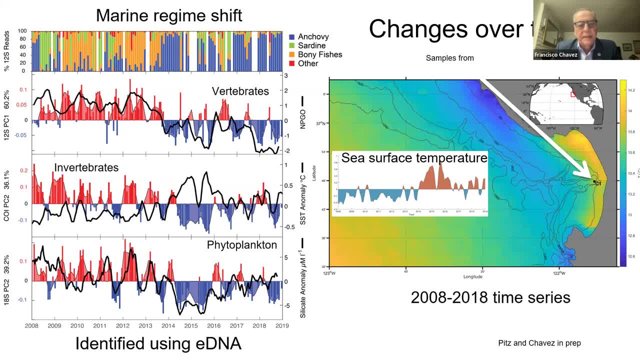 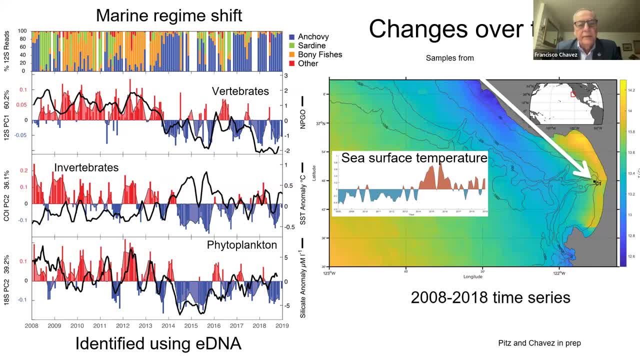 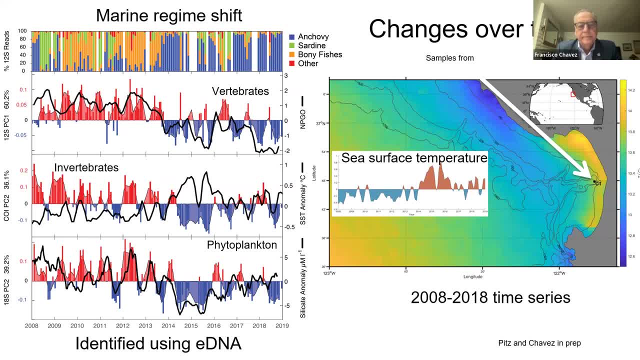 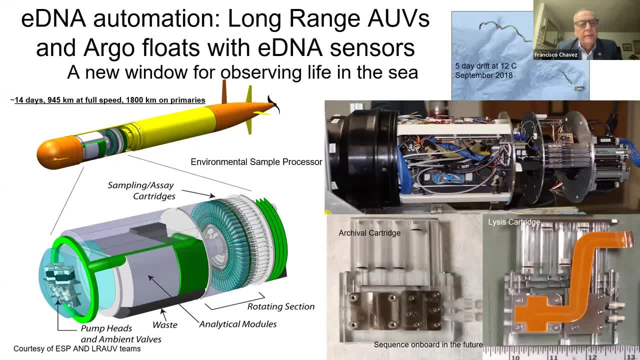 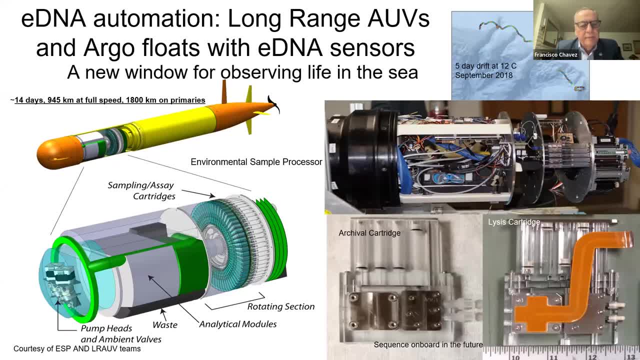 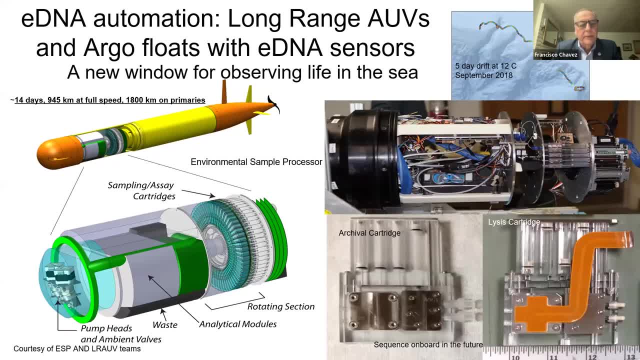 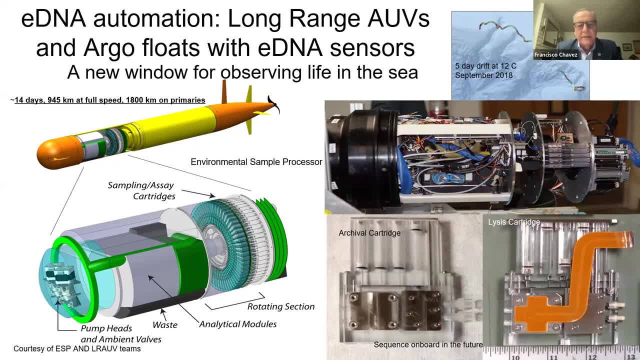 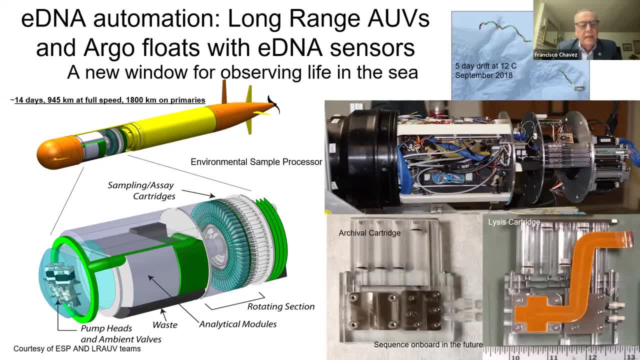 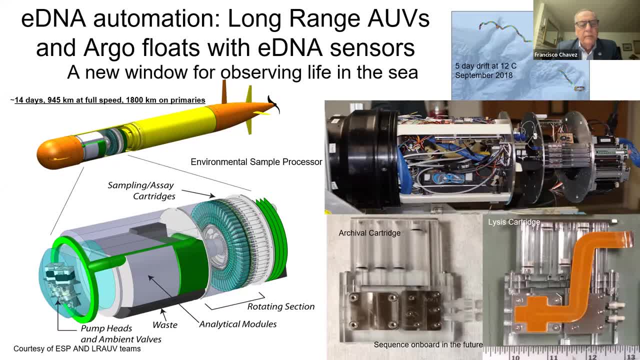 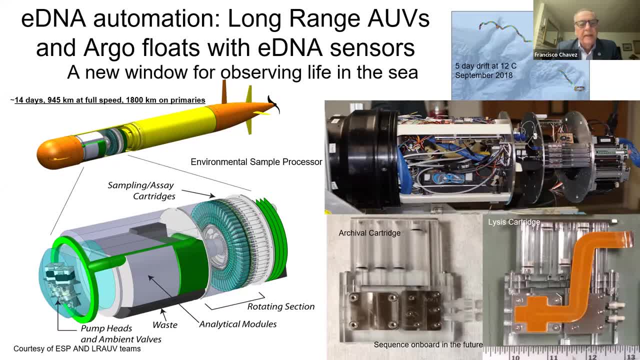 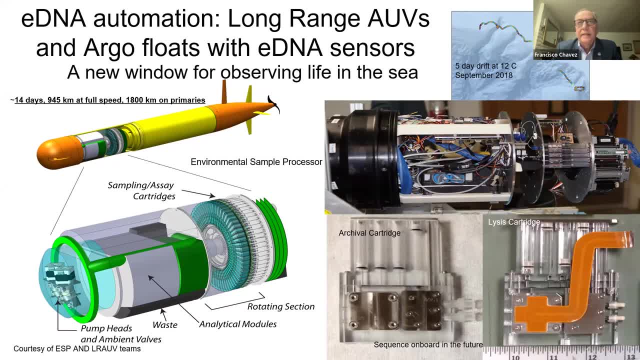 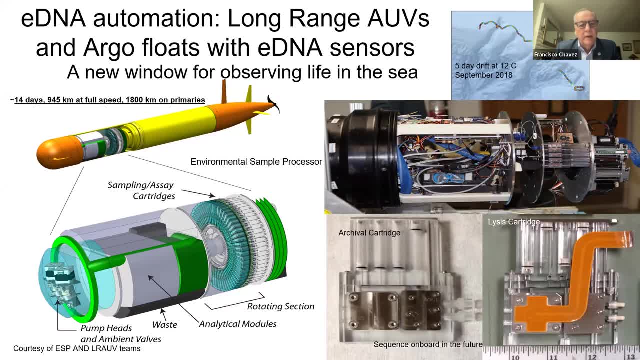 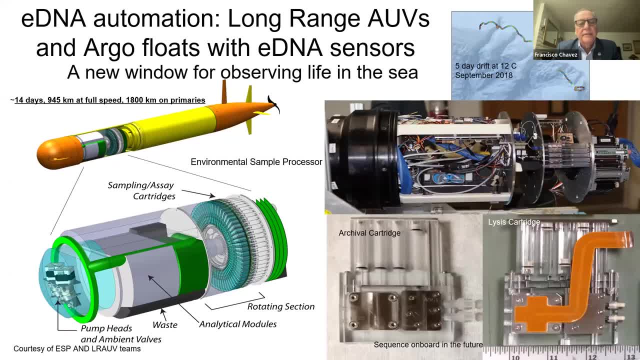 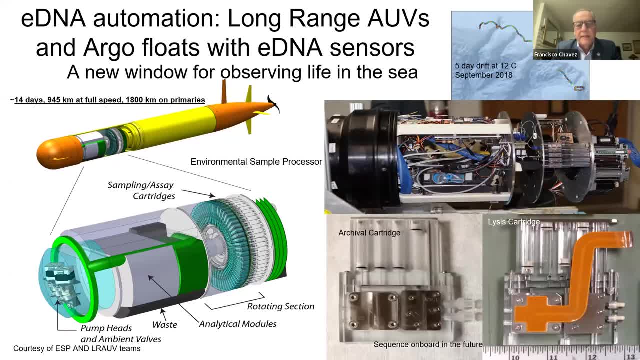 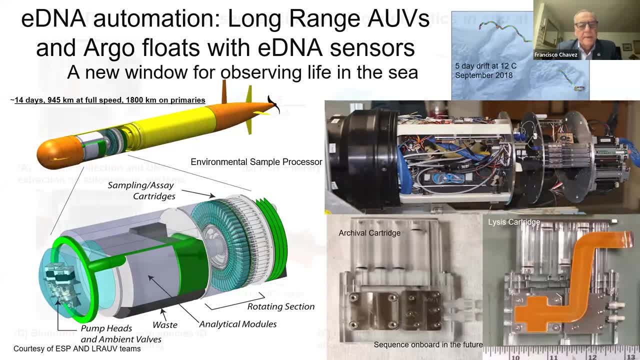 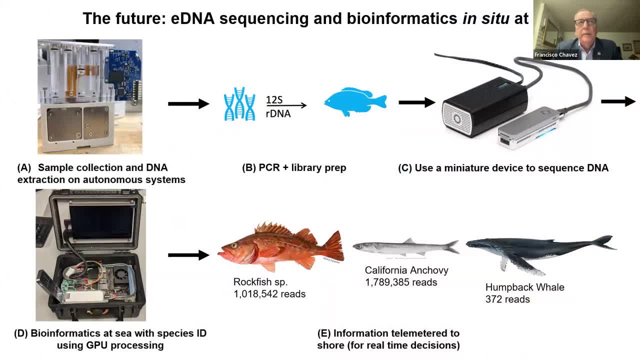 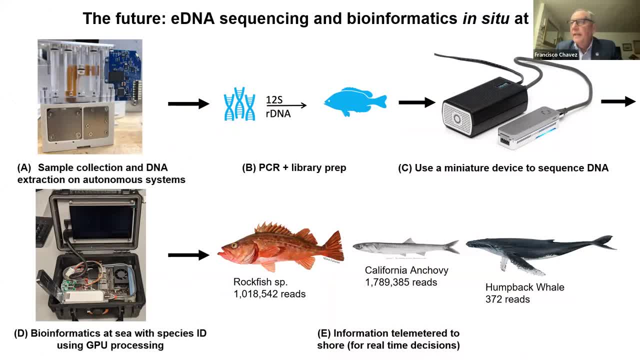 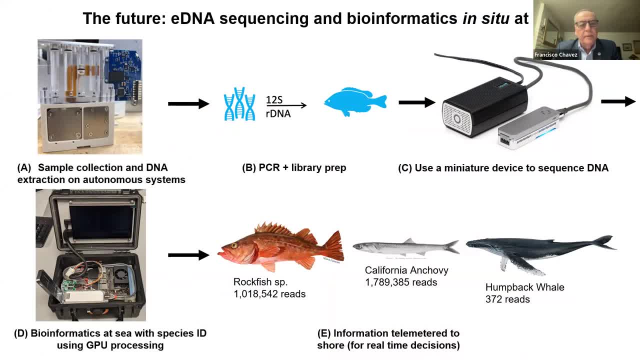 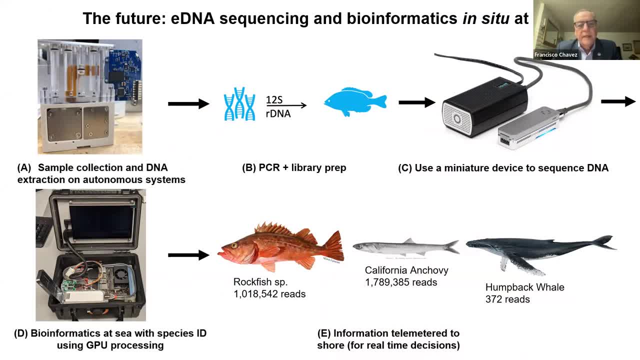 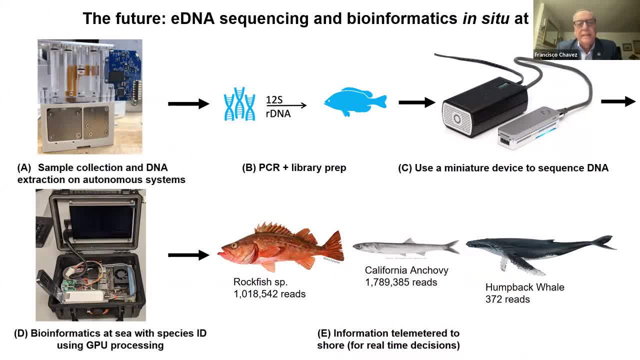 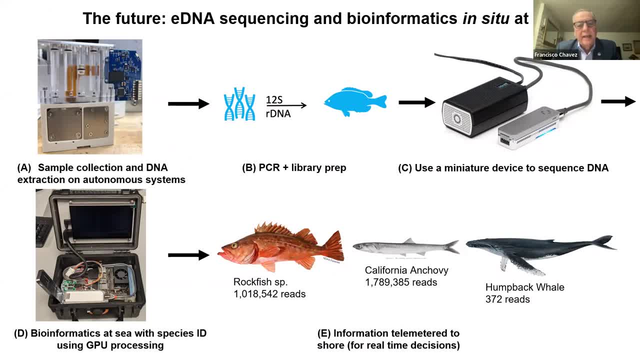 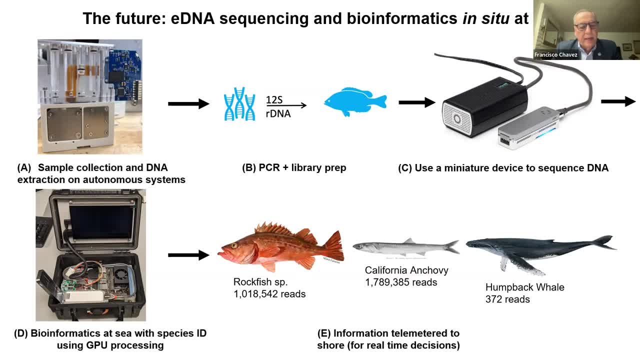 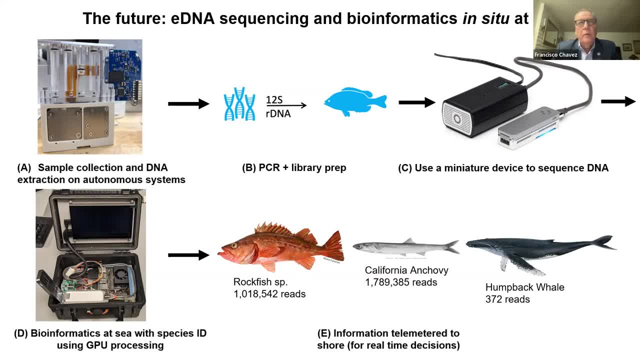 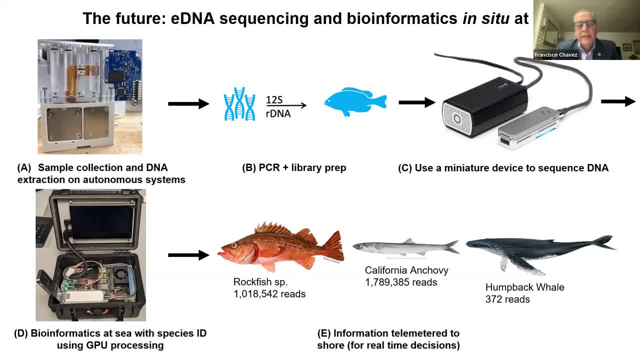 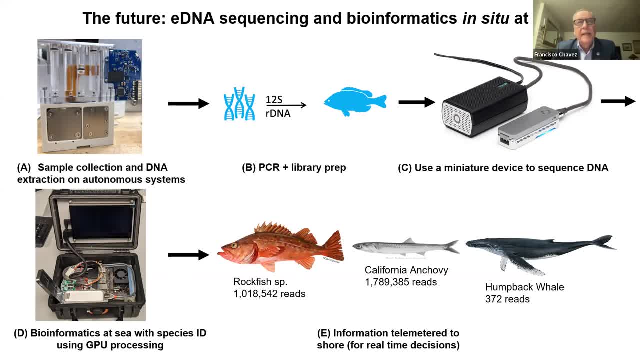 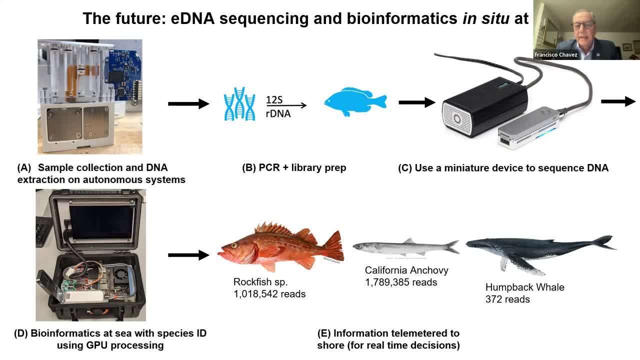 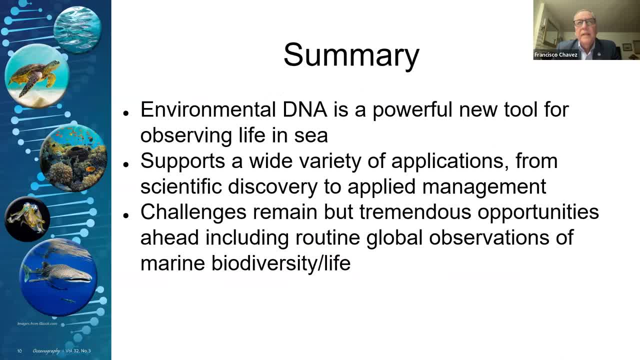 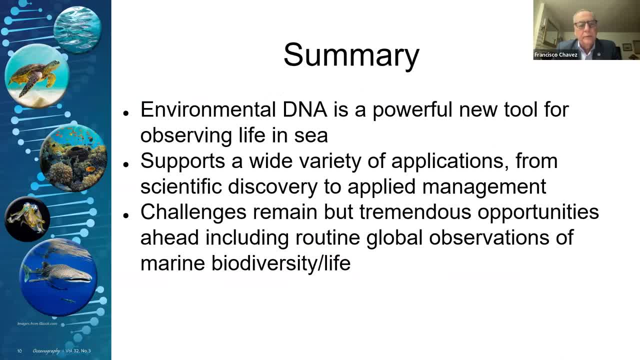 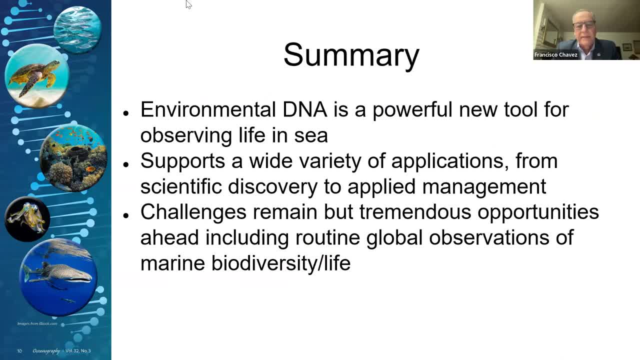 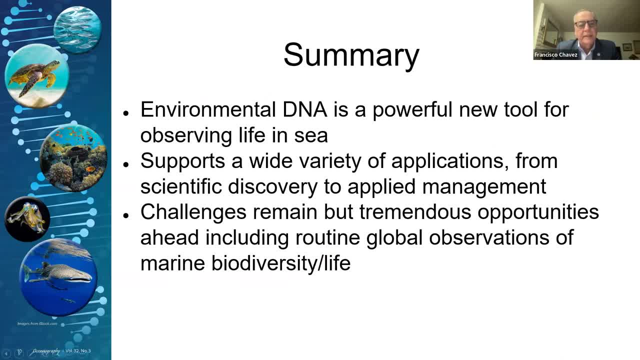 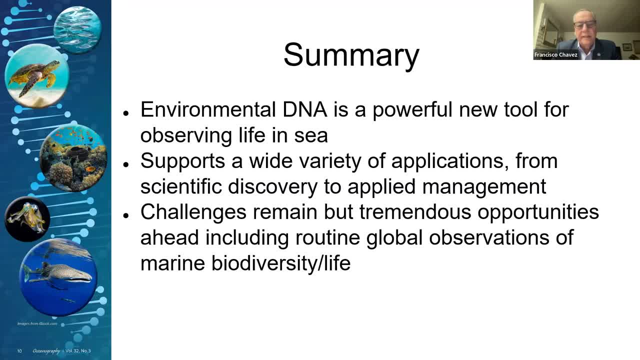 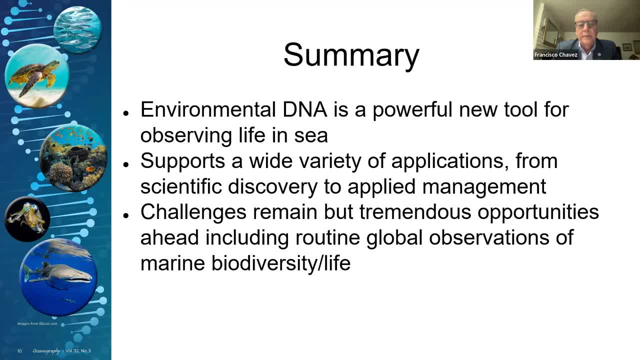 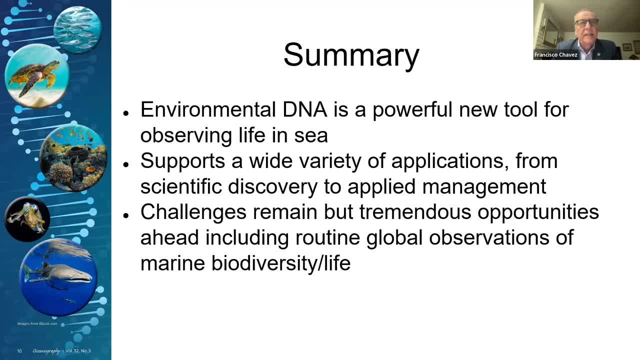 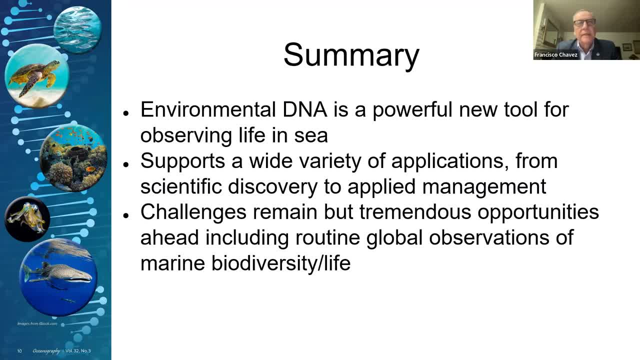 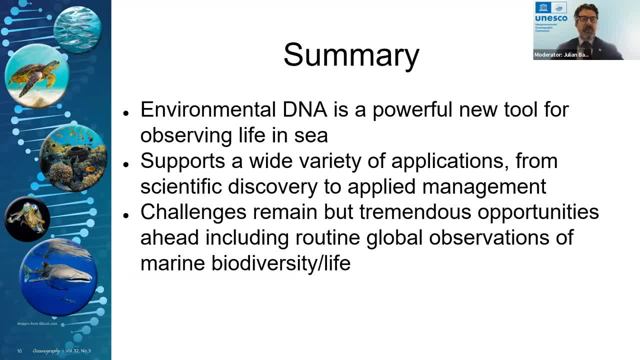 Thank you very much, Francisco. This is very interesting stuff. I'm not going to try to summarize, but I have a question that I've been struggling with and maybe you can try to give me a hint there: Knowing that we have so many species we don't know about in the ocean- and we've heard figures of about 700,000 species that are yet to be discovered by science- 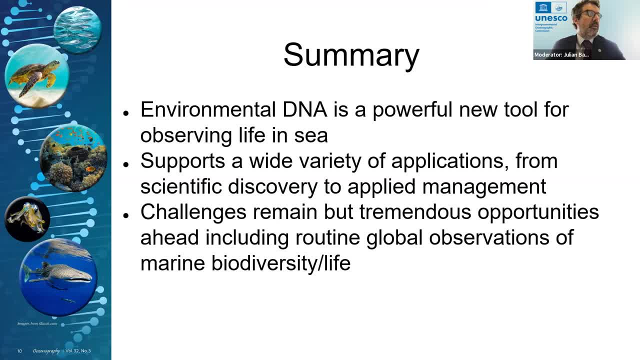 can the eDNA provide a tool for identifying those species, or species needs to be already referenced? It's kind of the same problem we have with our FBI or Interpol right. Many of our suspects are not in those databanks. The same is true, of course, for Life in the Sea. We have parallel efforts where we want to be able to get those sequences in the databanks. 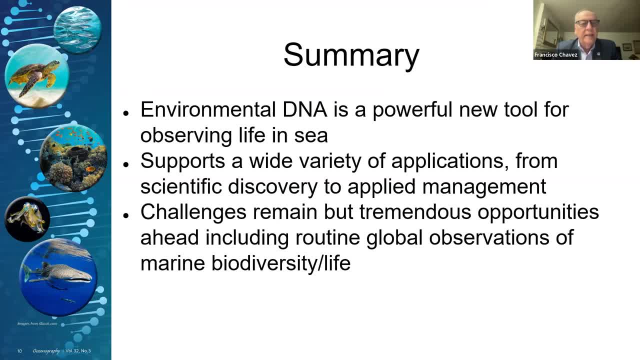 So that the eDNA can identify them. Today we can only identify maybe 50% of the species. we can identify with eDNA all the way down to species level. So that's one of our challenges is to build those libraries and complete them. 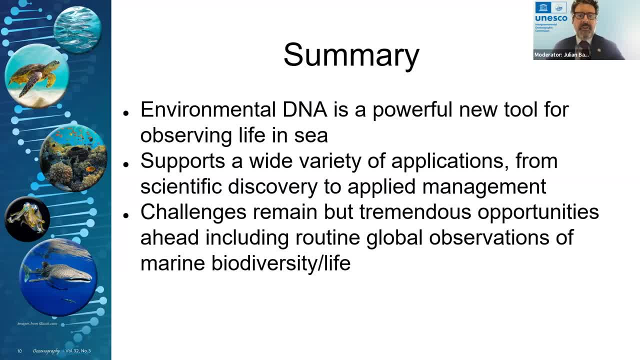 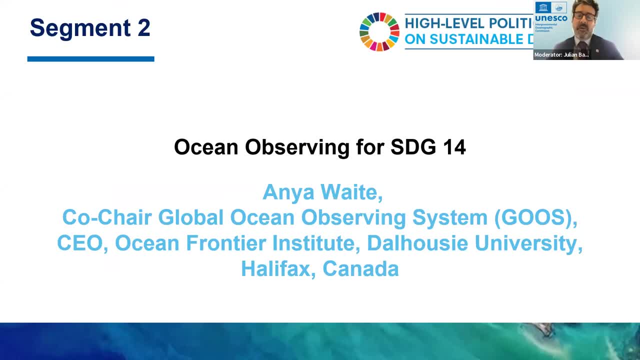 Great. Thank you for that. So we're going to stay on the topic of ocean observation and, of course, observation. We have a lot of data that we need to generate on the SDGs. So what are the challenges? And then we're going to also talk about how the SDGs are very important to generate the data that we need for reporting on the SDGs implementation, for example. 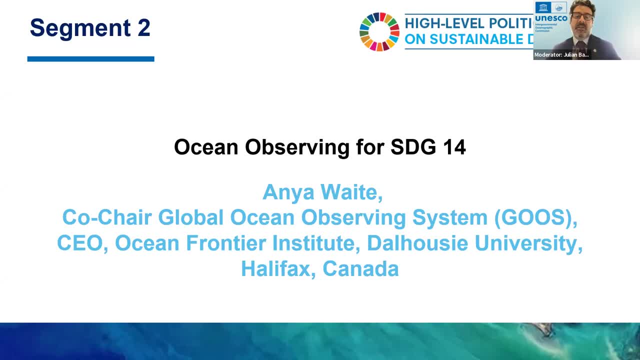 So let's now go to Ania Waite to tell us a bit about the international efforts that are ongoing in terms of ocean observing and how those actually contribute to the SDGs. Great, And thank you very much, Julien. Thank you, Can you hear me? Can you hear me now? 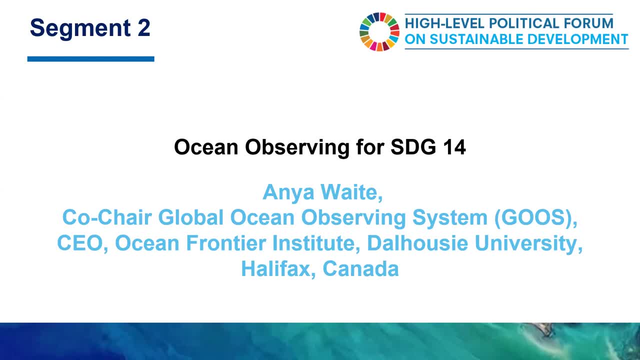 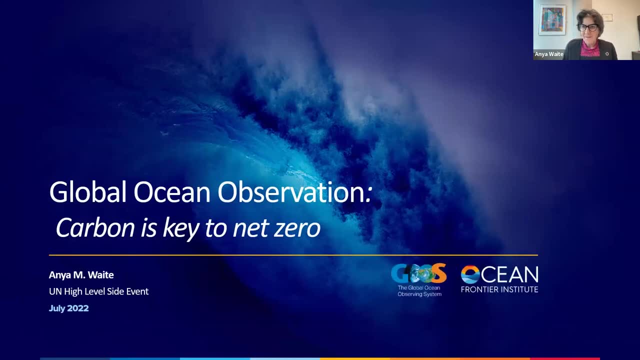 Can you hear me now, Julien? We can. yes, Okay, great. Thank you very much, Julien, and thank you to IOC, UNESCO, distinguished guests, ladies and gentlemen, Julien today asked me to speak to you a little bit about global observation of carbon and of the critical importance of the ocean in the climate system. 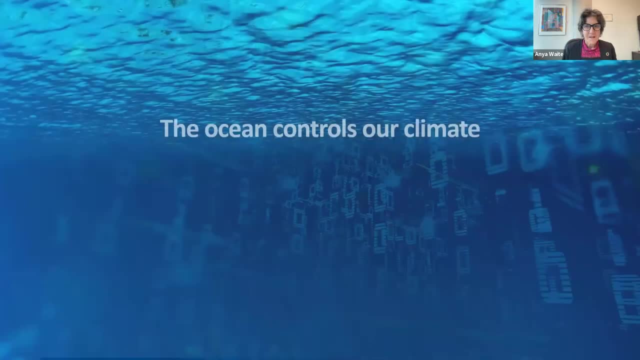 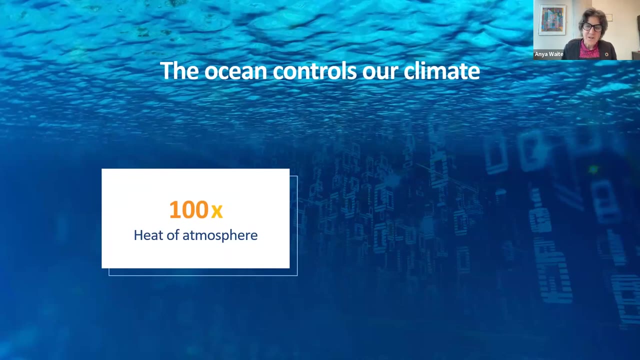 Next slide, please. So something that many are not aware of is that the ocean actually controls our climate. It holds 100 times the heat of the atmosphere next and 50 times the carbon that's held in the atmosphere. So in a sense, the ocean is our climate. 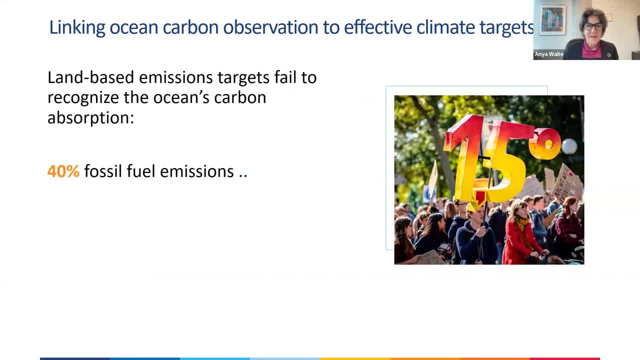 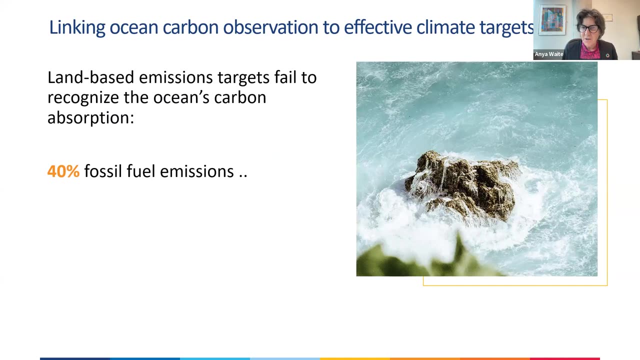 Next slide. So how do we link? How do we link the ocean to creating and achieving effective climate targets? The IPCC has highlighted for us that we only really have eight years at current emissions before we cross a threshold and rise above 1.5 degrees of warming, with serious consequences globally. 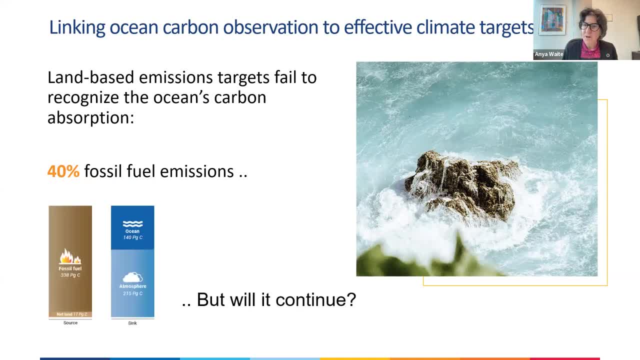 Very often we do our work on land, We do our policy work on land And land-based emissions targets. And land-based emissions targets fail to recognize that most of the work in the carbon cycle is being done by the ocean. So 40% of our fossil fuel emissions have actually already been absorbed by the ocean and that absorption may not continue. 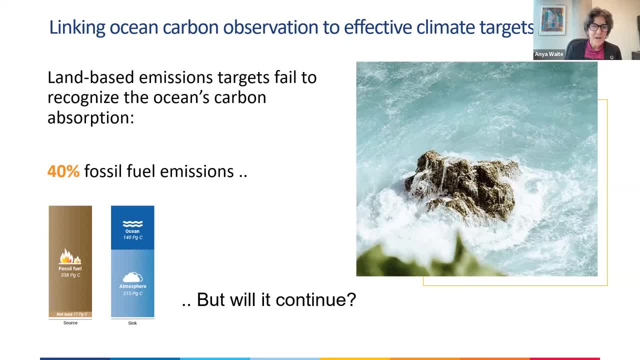 So on the left there you see two bars on the left-hand side, the source of fossil fuels: 340 petagrams of carbon from land-use changes and also from fossil fuel emissions, and then ocean and atmosphere absorption. And then on the hader side you see two bars on the right-hand side the source of fossil fuels: 340 petagrams of carbon from land-use changes and also from fossil gas Michaela Passie was talking about. and the third parts are that after carbon has gone into the surface of the ocean and has expanded into the atmosphere, most of its known has gone into the atmosphere, but the rest of it has gone into the ocean. 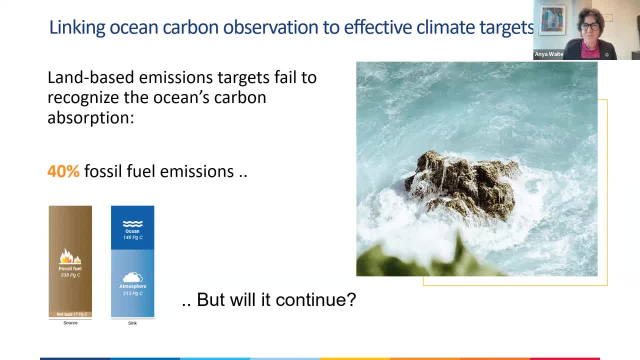 So if the ocean changes or starts to re Imit the carbon that is absorbed, that means that our land-based actions could be swapped By the release, for example, of carbon. um, so we, if we don't understand the trajectory of ocean carbon, we can't actually be confident in our climate targets, and it really undermines our effort to tell industry, for example, to stop a flood of carbon that is not actually a factor in these actions. 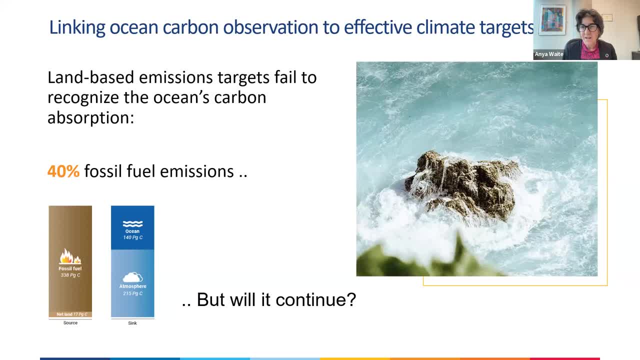 But if we improve to a solve our climate's available challenges, there will be resistance over our energy be confident in our climate targets and it really undermines our effort to tell industry, for example, to stop emitting carbon If we can't have enough confidence in the ocean carbon cycle. 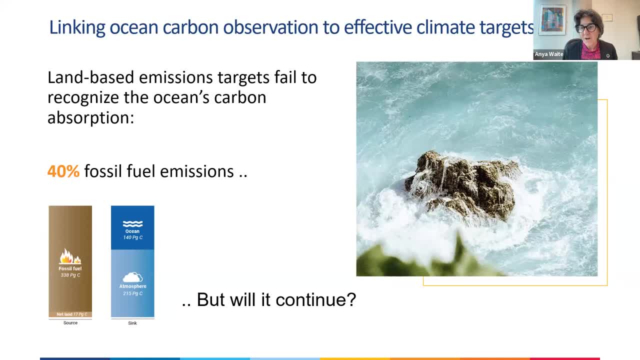 to understand it, for example, less than five percent. Right now it's between 25 and 30 percent uncertainty, and climate modelers can't even generate what we call a now cast, which is telling us exactly what's happening now based on data, because there simply are not enough ocean. 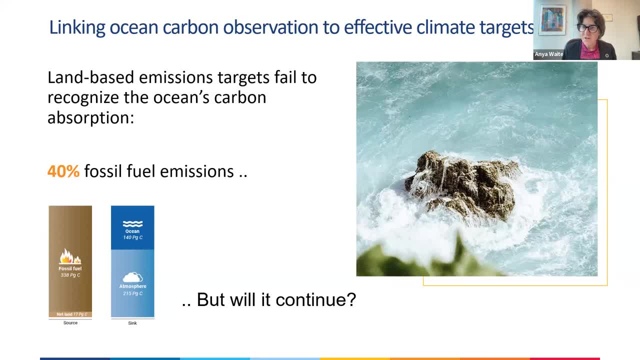 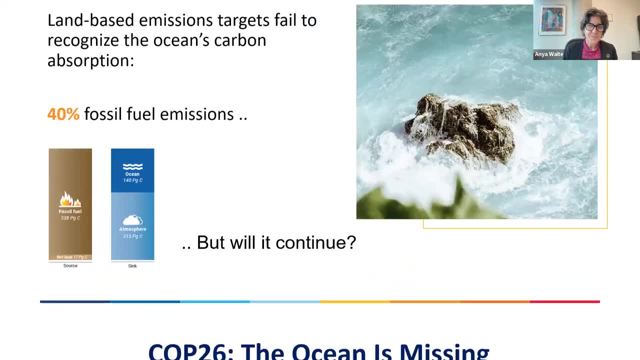 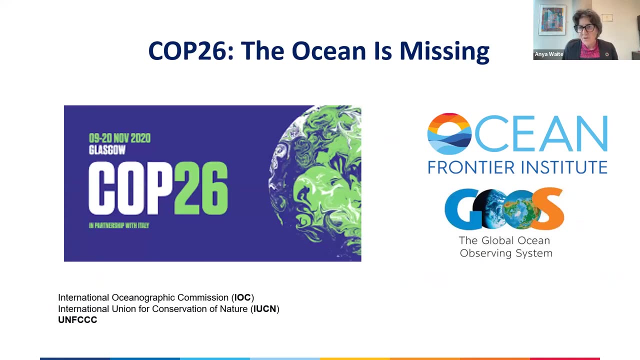 data And there are signs that extreme events in the ocean are increasing in frequency. We don't know how quickly that frequency will change. Next slide, please. So when we went to COP26 last year, the Global Ocean Observing System which I co-chair with, 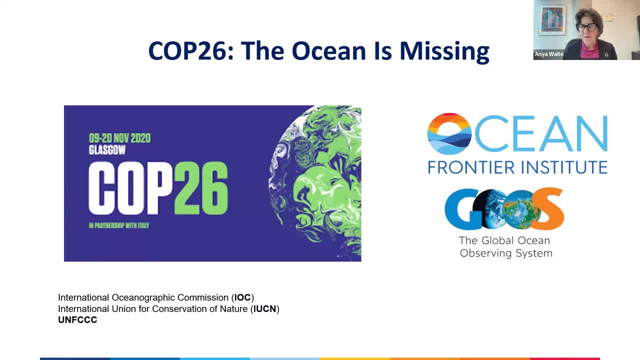 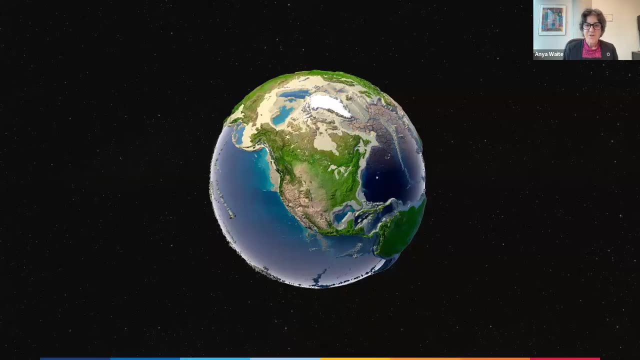 my colleague, Tosta Tanua sent the message to our global policymakers. the ocean is missing in your conversation right now And it's critically important that we put the ocean front and center in our climate discussion Next slide, please. We show the ocean without its. we show the world without its blue ocean. This is how we're actually. 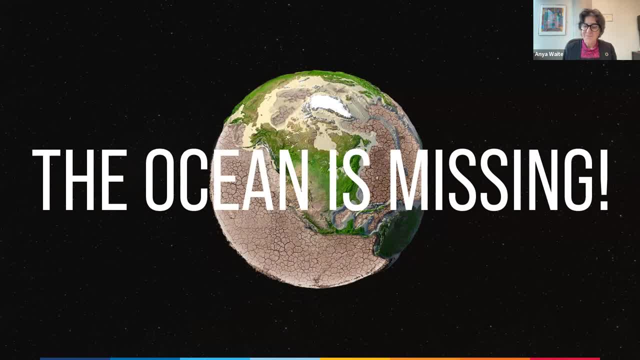 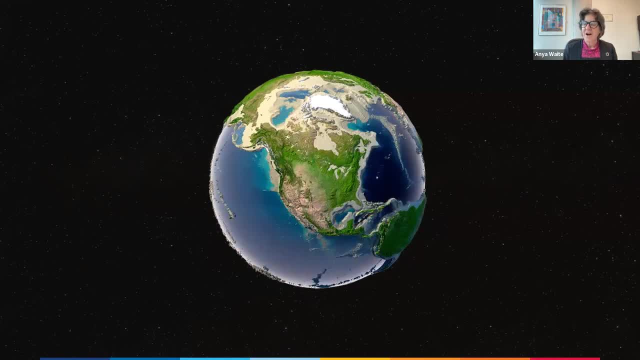 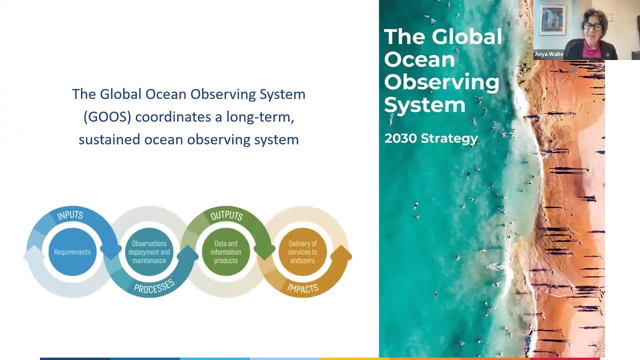 tackling climate change right now. Next slide: We need to refill the oceans with the water in order to get a sense of where we really are with our climate trajectory. Next slide, please. How do we do that? Well, the Global Ocean Observing System is a network of networks that 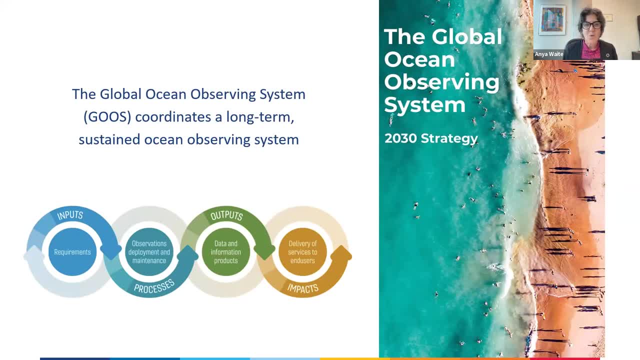 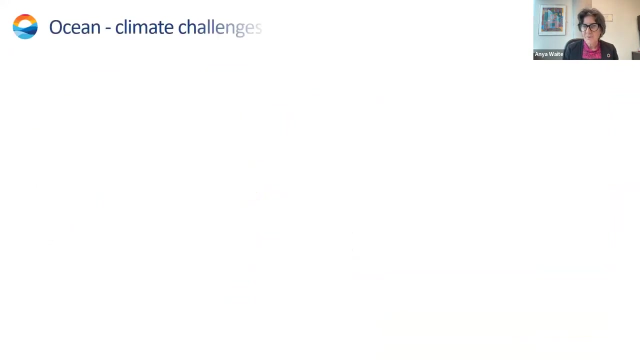 brings together observers from around the world to coordinate a long-term and sustained ocean observing system. This is a permanent organization and we deliver a report every year to the COP through Earth Information Day, And it's a very important organization because we actually reflect globally on requirements, on how we observe the ocean, on the types of outputs that are needed to. 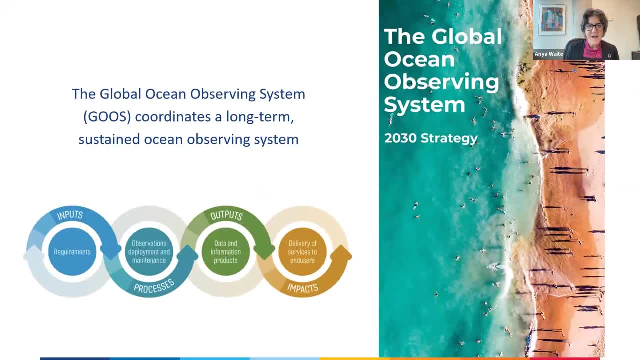 support the ocean and on the types of outputs that are needed to support the ocean. So we're a very important organization and we deliver a report every year to support policymakers. Sorry, if we could stay on that slide. And then, finally, the delivery of services to end users on their 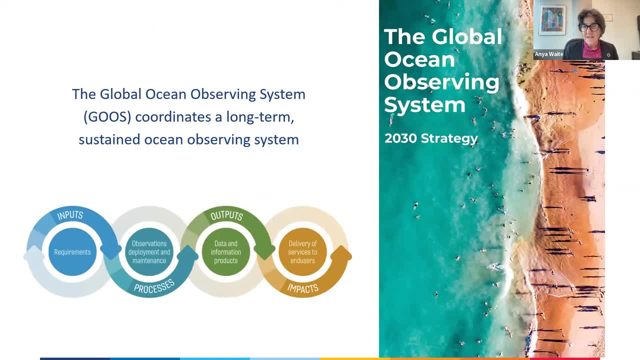 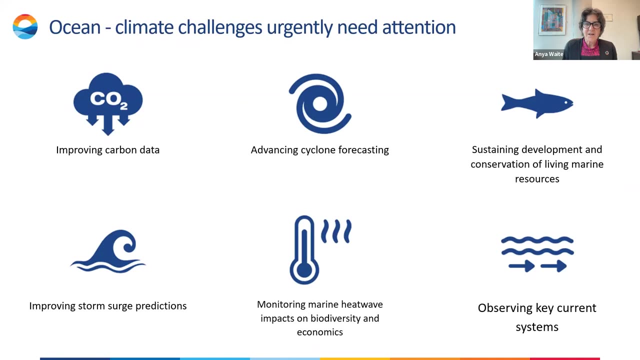 impact. Now the Global Ocean Observing System has recently instigated under the UN decade a new program called Ocean Observation Co-Design. Next slide And Ocean Observation Co-Design has tackled, for example, improving, basically focusing in on climate challenges that urgently. 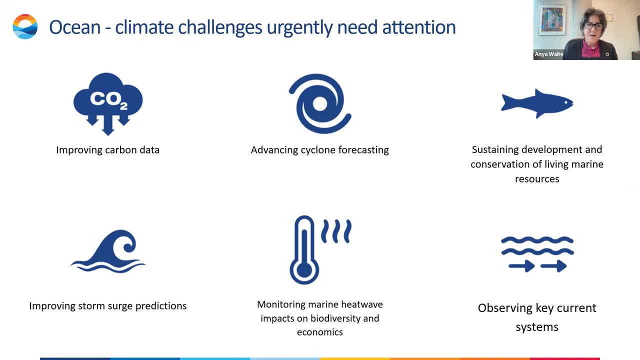 need our attention in the ocean observing space. One of the first is improving our understanding of the carbon cycle in the ocean, but there are many others, And once you create an observing system that improves carbon data, for example, you can also increase the observation of many other critical things in the ocean, like heat salt. 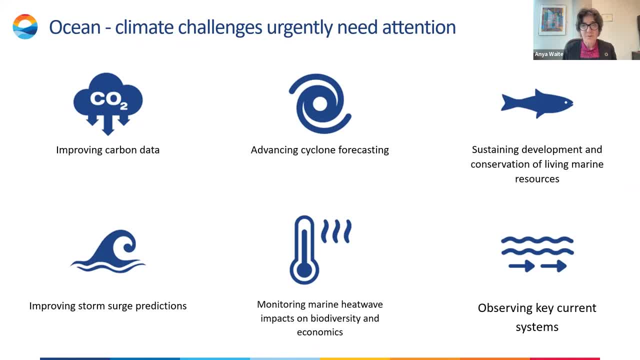 and other scalars that we need to address other problems. For example, many aren't aware that cyclone forecasting critically depends on ocean heat. The top 10 meters of ocean heat are actually what drives cyclone intensity- the amount of water that is held by a cyclone and therefore the length of 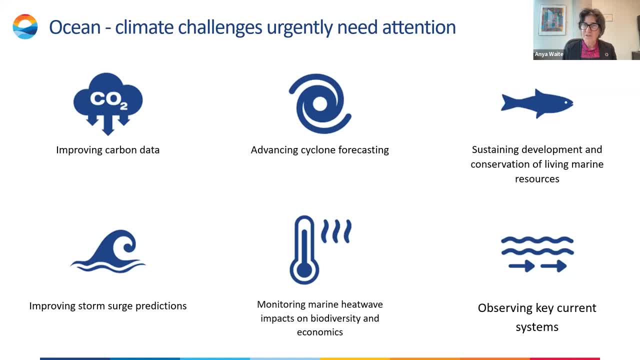 time that a cyclone sticks around is totally dependent on surface ocean heat. We also, as was beautifully discussed by the last speaker, we need to sustain conservation of living marine resources, And that's what we're doing. We need to sustain conservation of living marine resources And. 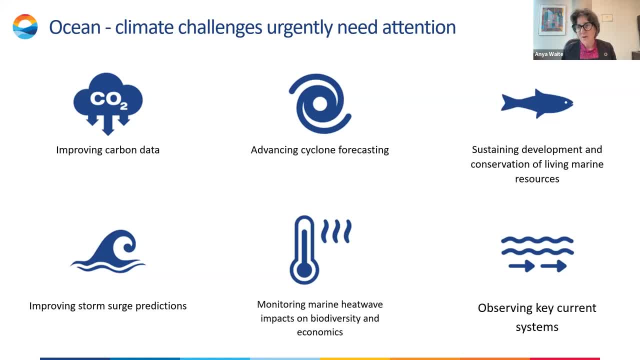 that's what we're doing. We need to sustain conservation of living marine resources, And that means putting out sensors that can measure eDNA, that can do underwater imaging and also that can bring new data to shore When we have storms. we need to have improved storm. 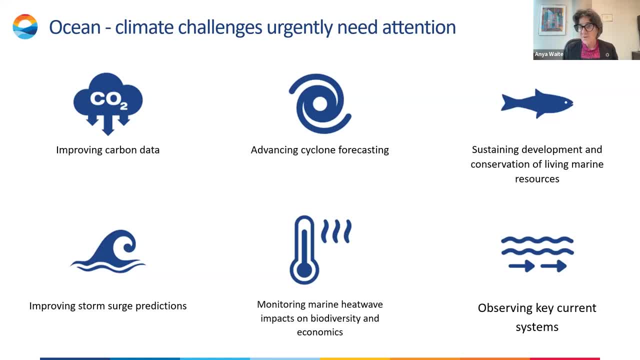 surge predictions. That's also data comes directly from the sea and marine heat waves that have increased radically in the last decade. we need to monitor and predict those, And all of these, of course, are driven by key current systems that move heat, salt and organisms around the ocean. 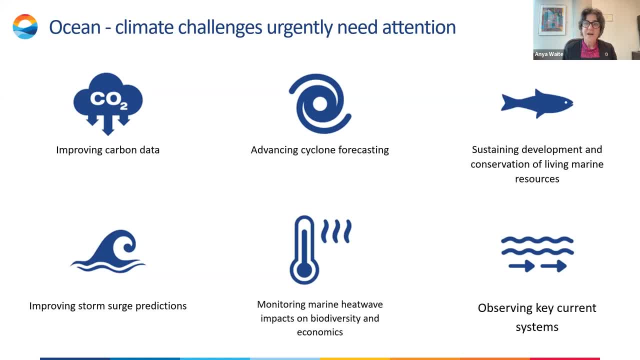 So these are our ocean climate challenges and these are the committees, the six committees of the Ocean Observation Co-Design Program under the UN Decade in the Global Ocean Observing System. So what do we need from the global community? What do we need from our policymakers? We need a massive lift Right now. the ocean is so. 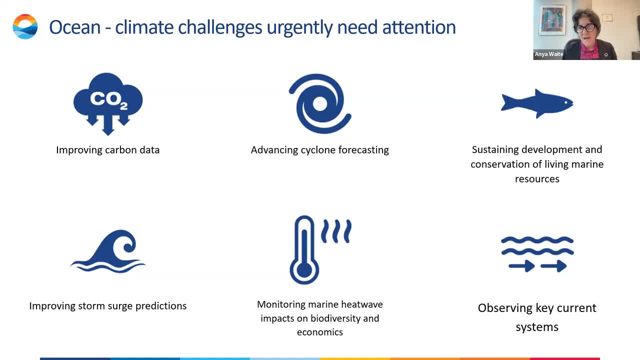 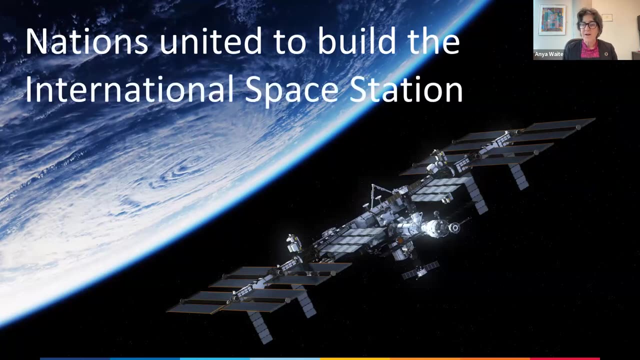 critically under observed that, as I said, we can't even generate a now cast of current conditions. We need to rethink how we observe the ocean. Next slide. The way we observe the ocean now is done individually by single countries putting observing systems, often in their local environment. But if we zoom out to the big scale, we can think about how nations 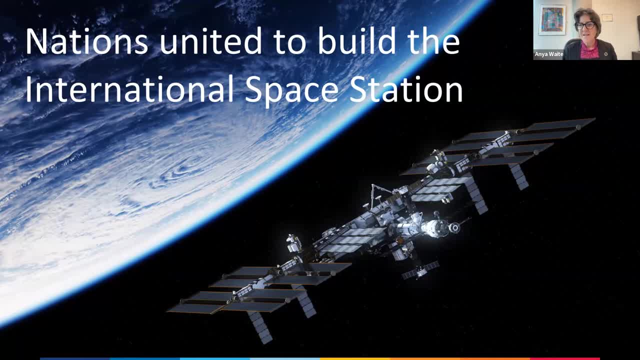 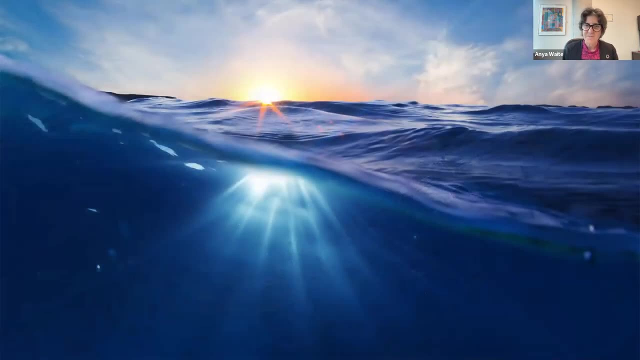 united to build the International Space Station, And this can give us an inspiration to think about. how do we observe the ocean at a step change where nations come together internationally to co-invest in the ocean infrastructure and ocean observation systems. So we must act at this same scale for ocean observation and 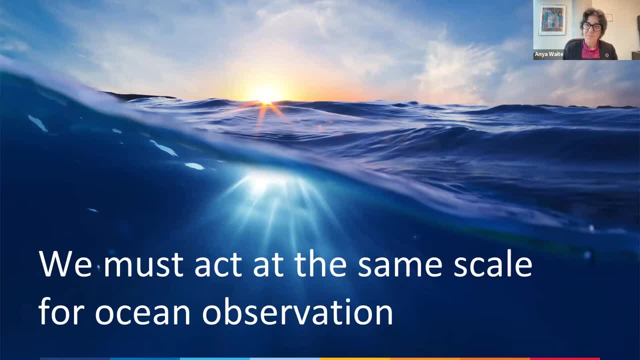 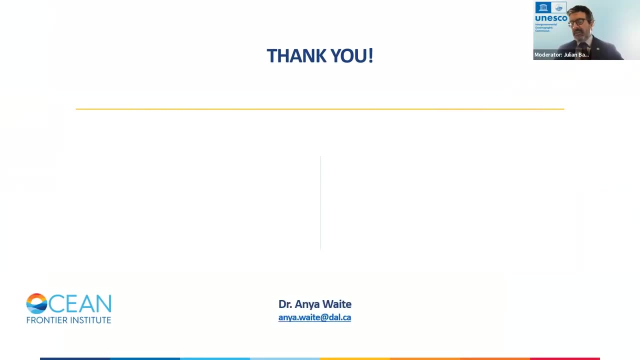 support the UN Decade of Ocean Science for sustainable development by the best possible observing system, And this is something that can be done if nations step up and work together to support ocean observation. Thank you, Thank you very much, Enya. This is also wonderful. 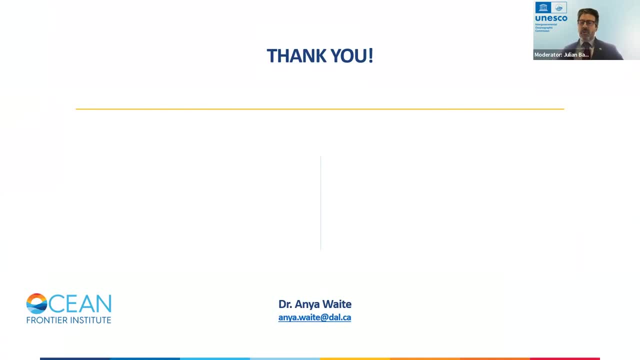 And so informative to really also understand the role of the ocean on a global scale in terms of the ocean carbon size And, as you said, and the need to really, you know, in committed infrastructure like ocean for the ocean. So that's what we need for really delivering the data and observations that can really help us with the management and the protection of coastal communities. So we're now going to go. 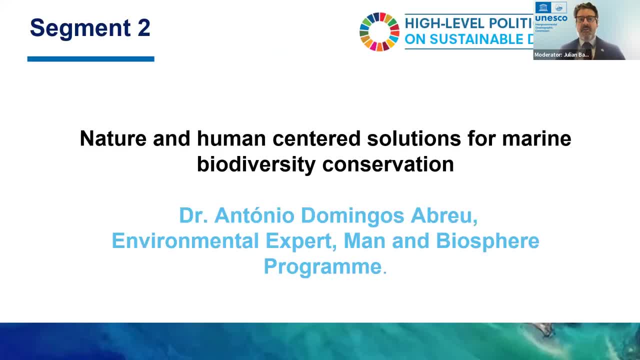 from what we're doing now, we're going to start talking about a few issues that we'd like to cover, And just from a really local scale, from the global scale to the very local scale, and really look at- And that's what actually serve. the more local scale and go back to what the world asked us and where we can in in specific areas of the world and in particular, I think we will dwell into the biosphere reserves. and UNESCO is managing a huge network And Dr Antonio Ambaro is going to tell us all about it. over to you, Antonio. 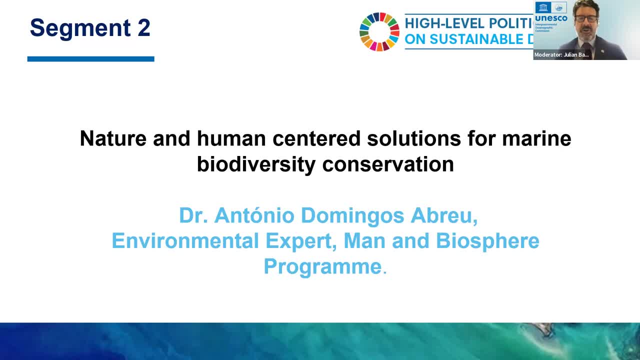 And that's what I want to do. Thank you very much and, Julien, Thank you to the organizers for allowing us to represent you and actually manage every one of the communications coming from this area. that's how you would think we all in those categories, but dreaming about biores meille. 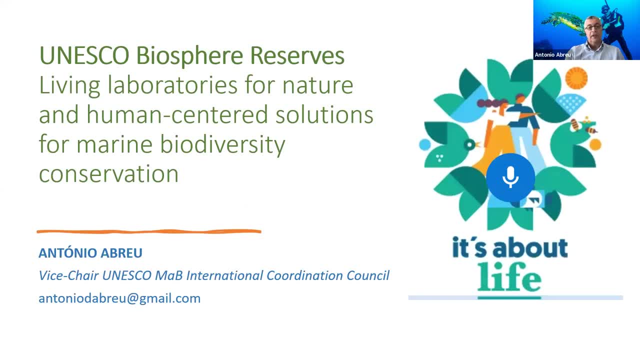 analysis capability are totally fluff. Thank you very much you to the organizers for allowing us to give some information and perspective from the UNESCO Biosphere Reserves. In fact, I will start by informing that during the last meeting of the MAB, Man and Biosphere International Coordination Council, there was a message from Monaco, endorsed. 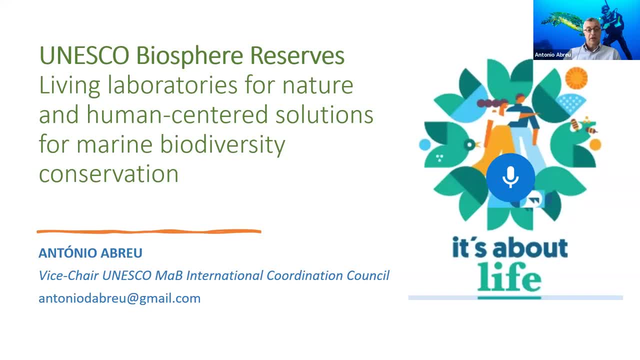 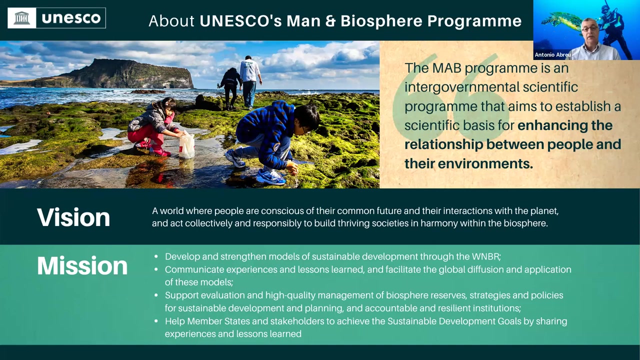 by Portugal, encouraging a broader connection between UNESCO, MAB Biosphere Reserves and the UN Decade for the Oceans. So this is part of the message that I start by delivering. Can we move into the next slide, please? And just a brief about what is the UNESCO Man and Biosphere Program? 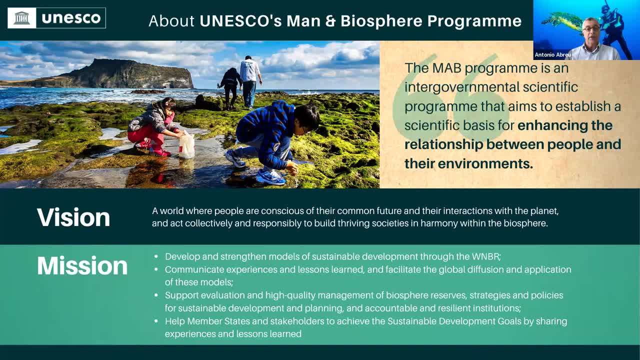 and then of the which the Biosphere Reserves are the central actors. So the MAB program is in fact a scientific program, intergovernmental program that aims to establish a scientific basis for enhancing the relations between people and the environment. This means that there is a knowledge and research. 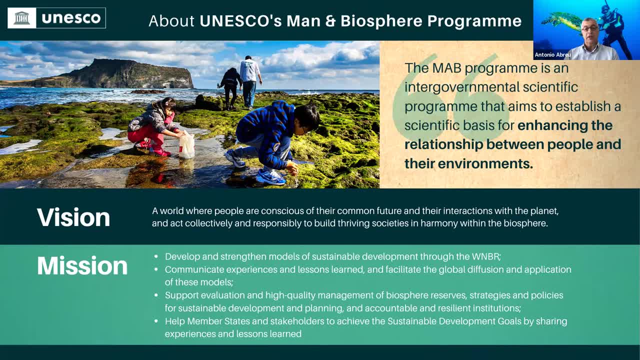 base, a basis that then will be explored and used for not only conserving or promoting biodiversity conservation, but also socio-economic development. Also, as socio-economic development, The program is very well established since 2015.. There is a strategy and action plan. 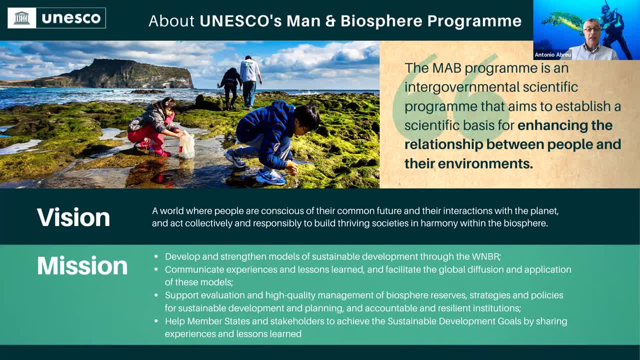 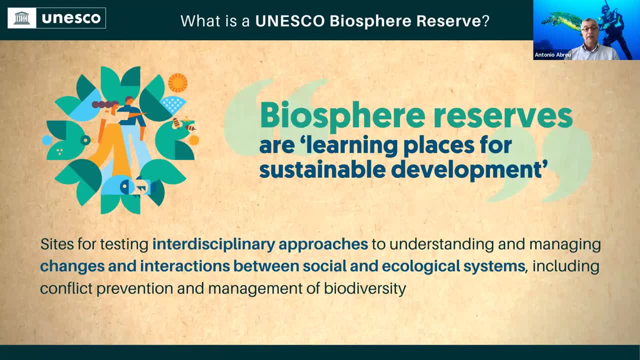 with a vision and the MAB Secretariat that is hosted by UNESCO Division of Ecological and Health Sciences as a mandate. Can we move into the next slide, please? are acting as learning places for sustainable development, One of the best definitions that we can find for these sites. 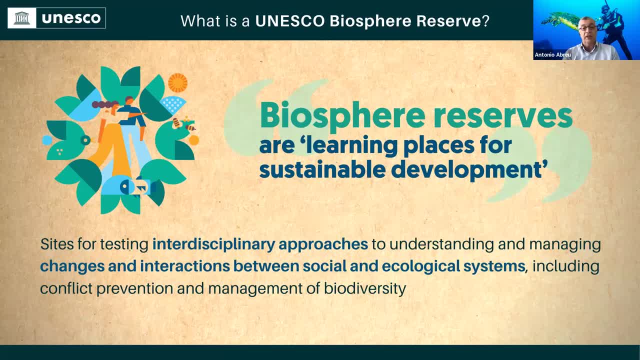 is that they really are living laboratories for testing interdisciplinary approaches, So not only looking at one level of the environmental or social economic development, but mixing all kinds of vectors and disciplines In order to better understand and manage the complex world that we live, all the changes and interactions between social and ecological systems. 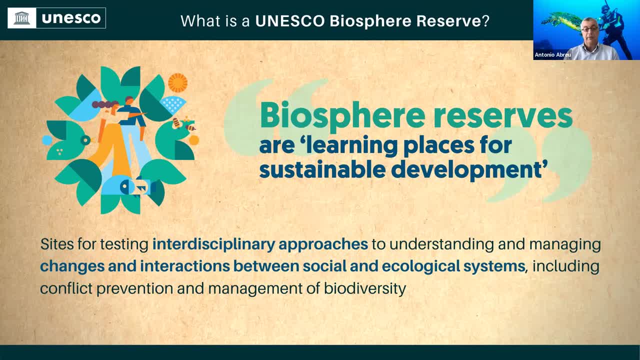 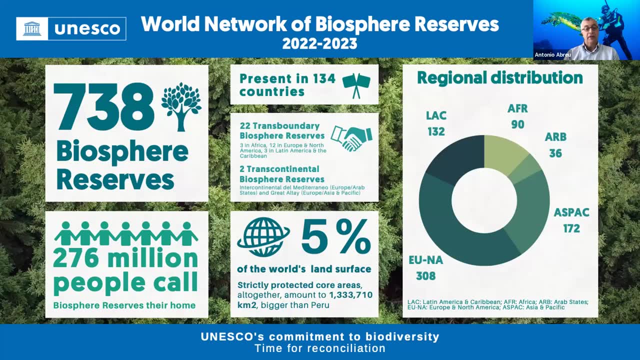 including peace and the management of biodiversity. And next slide, please. We are not talking about just protected areas or nice sites with outstanding biodiversity that are recognized for these assets, But we are talking about 276 million people that live inside the UNESCO Biosphere Reserves. 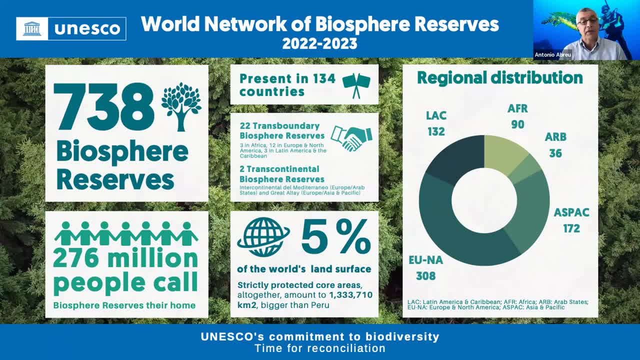 that are spread all over the world in 738 designated sites, including some transboundary biosphere reserves, which means cooperation, both bilaterally or multilaterally, including continental cooperation, and they are distributed all over the world. So this is the stage in our point of view. 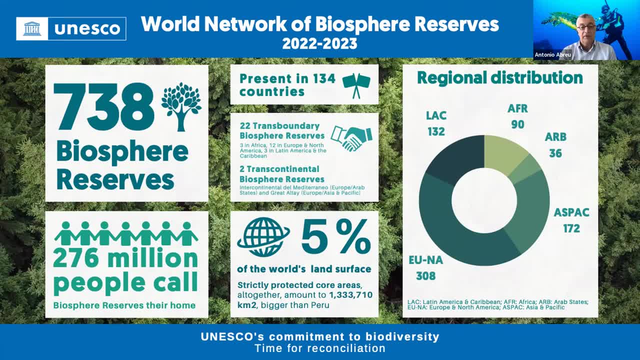 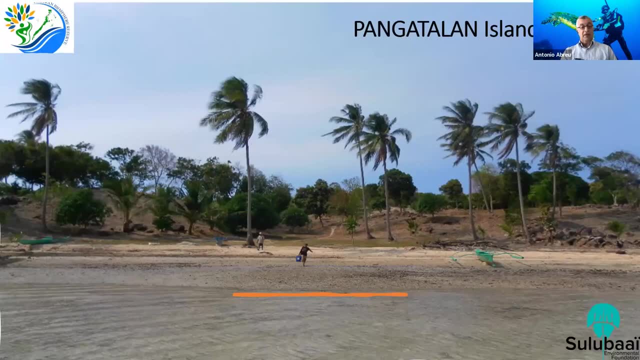 that could fit and help and support most of the discussions that we held here today. Next slide, please. I will go now into two or three examples. And because biosphere reserves are sites where daily the communities, the researchers, the managers, the policy makers are working. 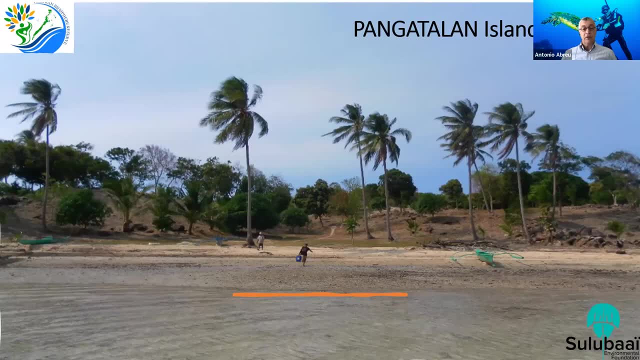 So this is. I will tell a little bit of two or three situations, And it's good also to bring good stories and because we need hope and we need to demonstrate that it is possible to do things, And this is the case of a biosphere reserve in Palawan Island in the Philippines. 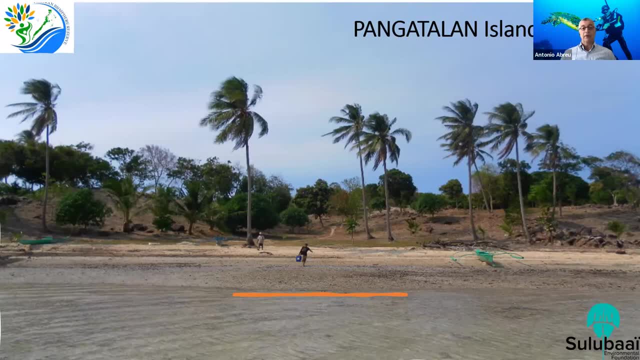 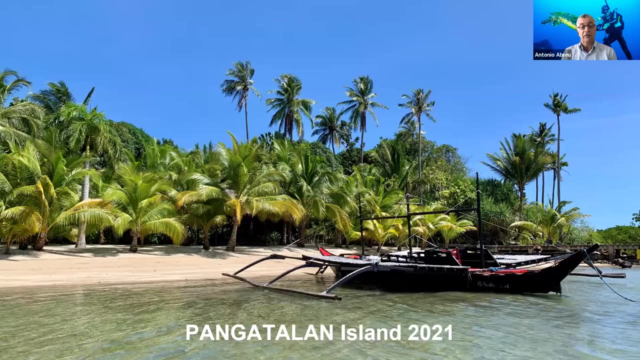 where, in a particular island, a close to Palawan, Pangatalan, this is the aspect of the island in 2011.. And next slide, Next slide, please. And currently, this is the same island. Of course, there is here a lot of work on restoration, ecological restoration. 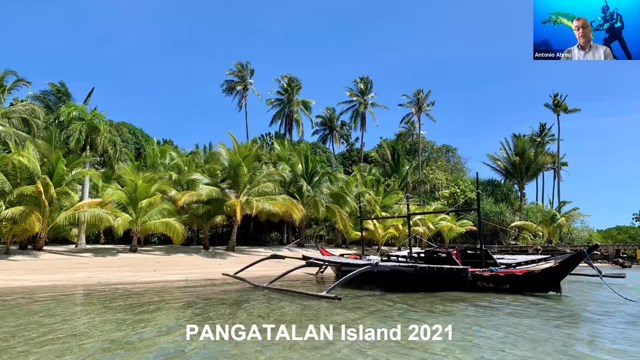 and recovery of habitats, terrestrial and coastal. But this island is mostly like a research vessel that is looking to the sea, So I am not showing the island as a success case for the terrestrial situation. Next slide, please, Because it will be a minor example. 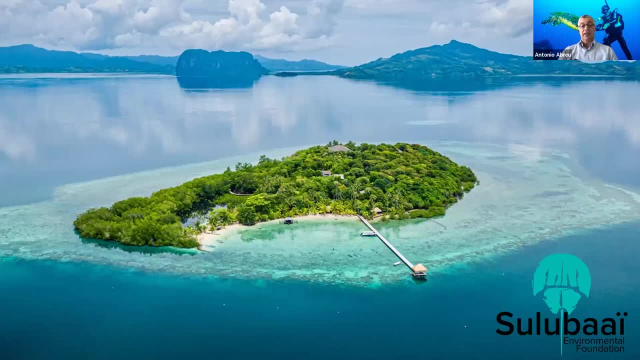 So this is a small island that is managed by, so by foundation, And as an example of recovery it's good, but not enough because it's very small. So from this island- and from this point it's a positive perspective- to by foundation. 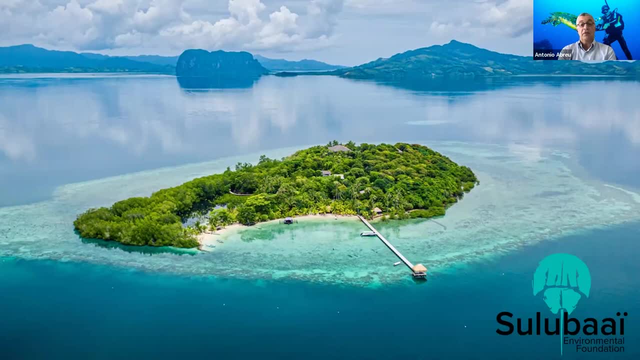 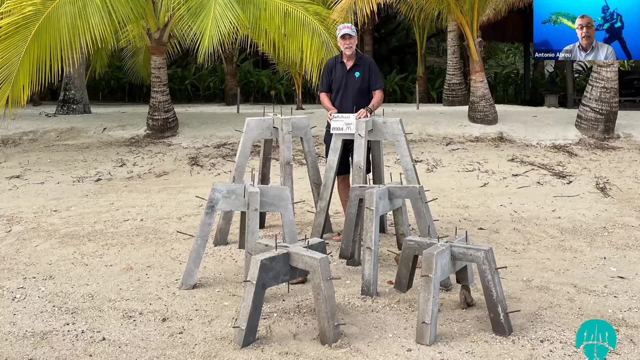 Next slide please Establish the strategy for the ocean, And the idea is to recover the sea as and restore the coral reef and the marine ecosystems, as they did for land. So some research in land and in shore led to the development of processes. 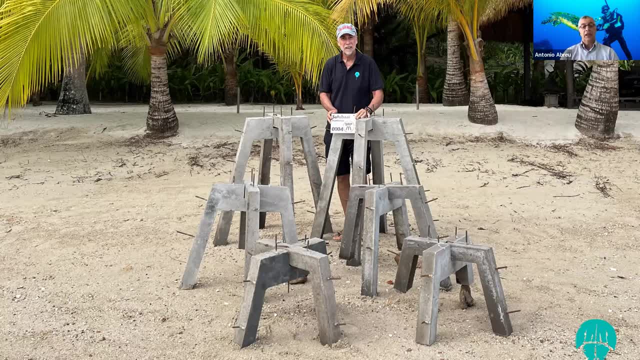 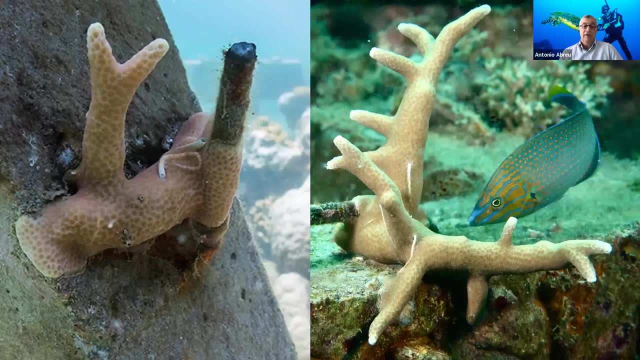 And several initiatives for restoring coral reef. Next slide, please. And the monitoring after five years is showing a great development and capacity of the coastal and coral reef ecosystems to restore and recover at a quick and very fast speed. Next slide, please. So we are talking about a lot of work. 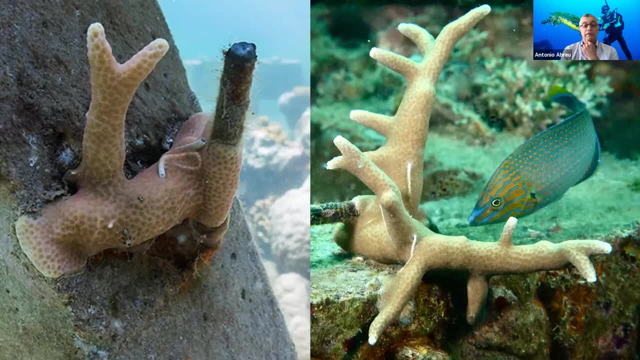 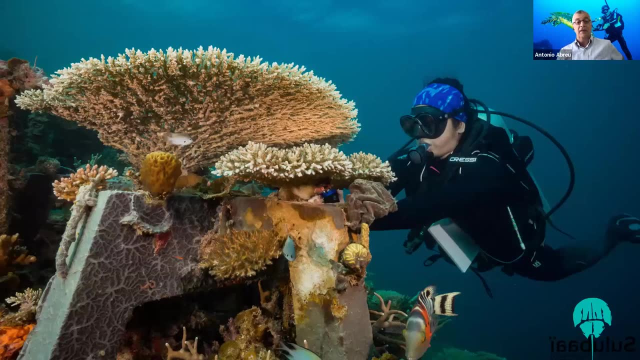 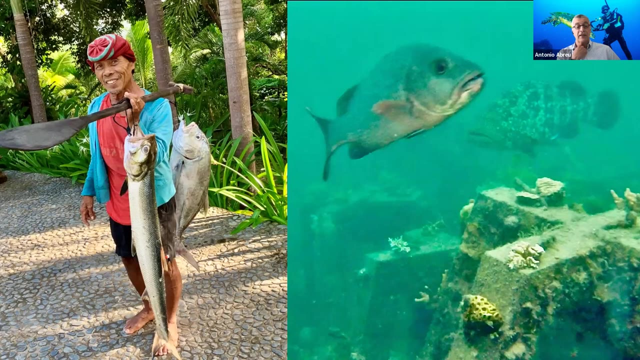 Live situations that we can monitor and follow visibly. So these are the structures after a few years. Next slide, please, That shows that biomass, maritime biomass, is increasing and that opportunities for artisanal fisheries can be recovered. Next slide, please. So the idea here around the Pangatalan Island. 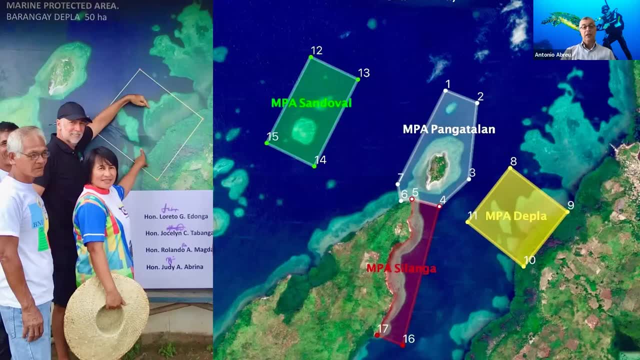 that is, the central marine protected area that you see, this was a demonstrative success case that was immediately transferred into the neighborhoods. And so by engaging communities, by promoting what is called the Sea Academies, promoting ocean literacy and alternative livelihoods based on science approach, 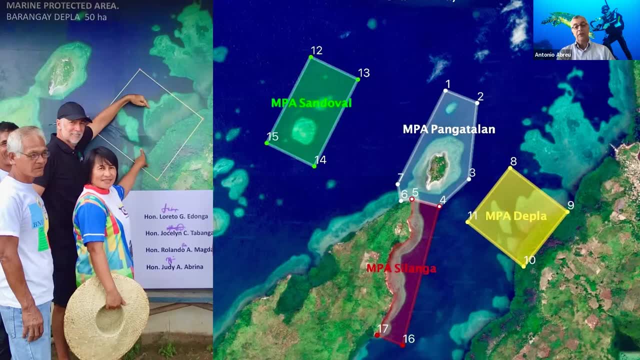 like capturing post larvae that are used for aquaculture- inshore aquaculture- that feel two purposes: One, feeding the communities and providing income as well, and reducing the pressure in the system, but at the same time allowing to grow key species for recovering the marine habitat. 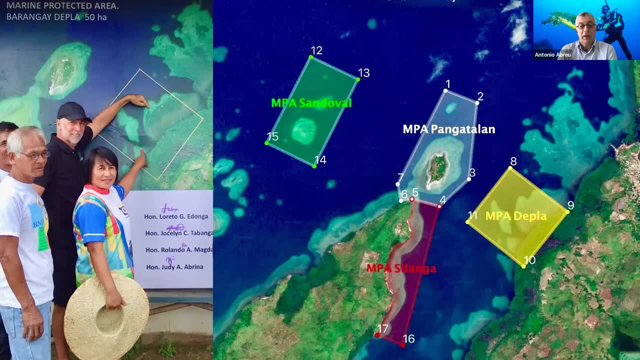 So this is one of the examples to me, one nice story from a biosphere reserve that can be easily transposed and used to show all dimensions of our discussion today. And congratulations to Sulubai Foundation and especially to the leader, Fred Tardieu. 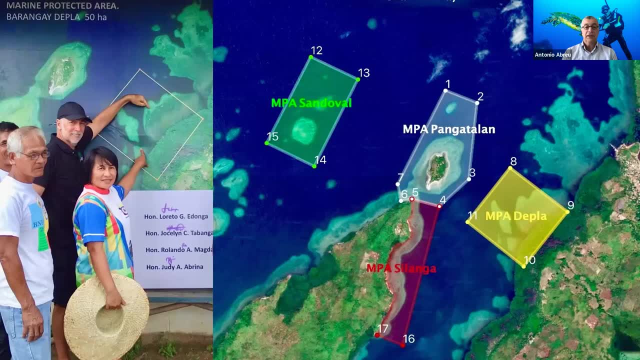 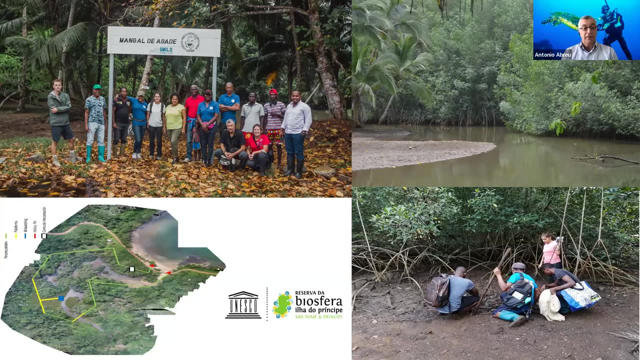 that is in the middle of the photo. Next slide, please. Another example from a remote island is in Principe Island, the UNESCO Biosphere Reserve, where a few stakeholders and community fish, small community that lives in the bay shown below in the picture below on the left. 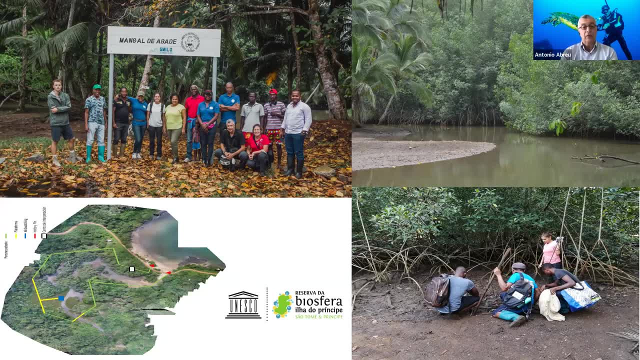 is recovering one of the few mangrove remaining sites there in the island. So the idea is to bring information and to promote restoration at the same time, by providing capacitation to local communities in order to use the mangrove for not only ecotourism-based information. 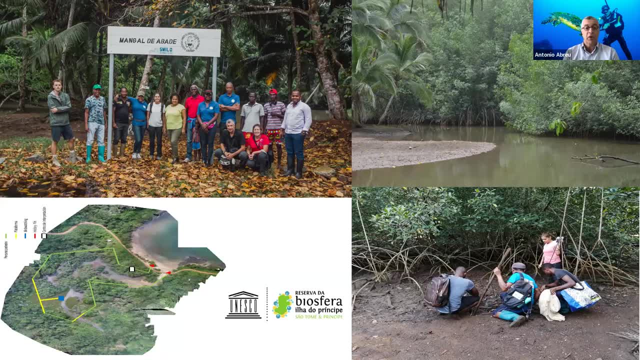 but also for monitoring biodiversity. So a baseline was established, including a lot of citizen science, and techniques for restoring the mangroves were implemented, And this is targeting the restoration of the coastal ecosystems as well as fighting and preventing erosion of the coastal areas. 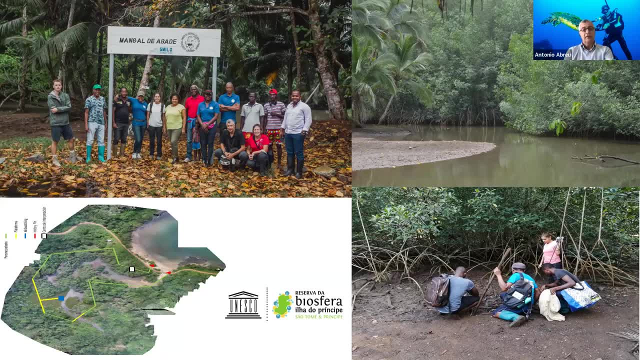 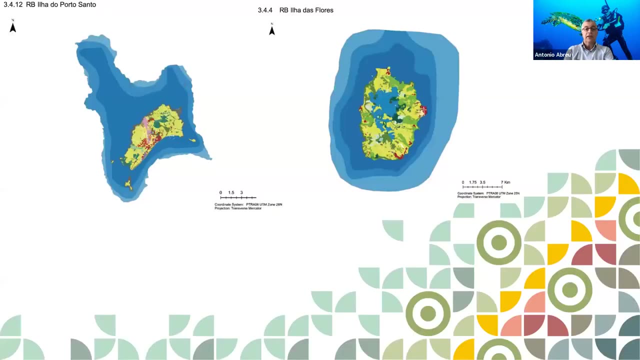 Again a small project, a small initiative that ensured the participation of all local, national and international stakeholders. And the next example and the last, please Next- slide Is about an ongoing initiative in Portugal. Portugal has 12 UNESCO Biosphere Reserves. 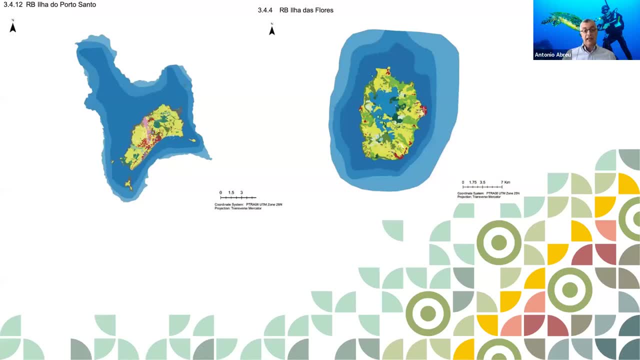 and they are being being mapped on the ecosystems and ecosystem services, And that exists in each of the UNESCO Biosphere Reserves. In this case, we have two islands here On your left side: Porto Santo Island in Madeira Archipelago. 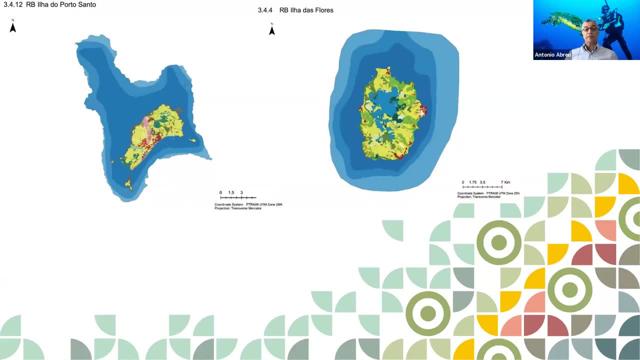 and the other island is Graciosa Island- sorry, Flores Island in the Azores Archipelago. So all the existing marine and coastal ecosystems were mapped and now are being assessed and evaluated on the ecosystem services by identifying key ecosystem services and the identification of key ecosystem services. 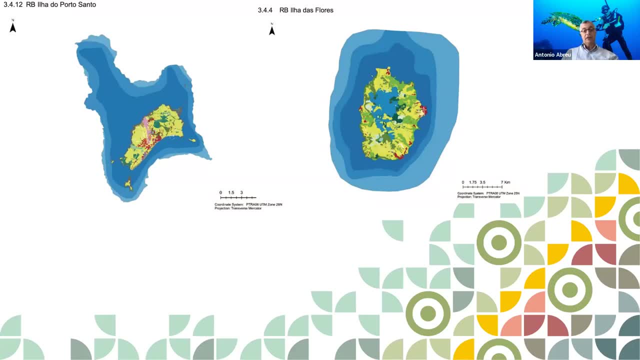 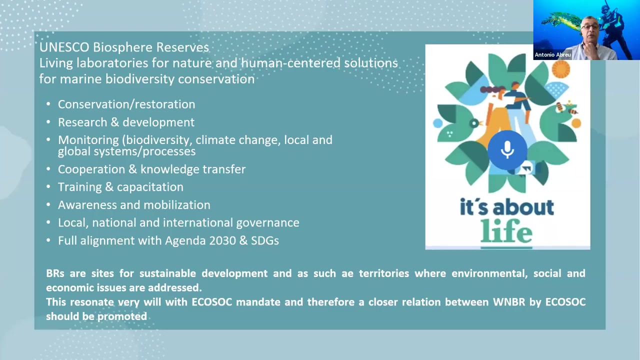 It's not only a technical or scientific issue. it's based on a participatory approach by including the local population on the analysis and the decision of which are the key ecosystem services. So in resume next slide please- I will say that UNESCO Biosphere Reserves act. 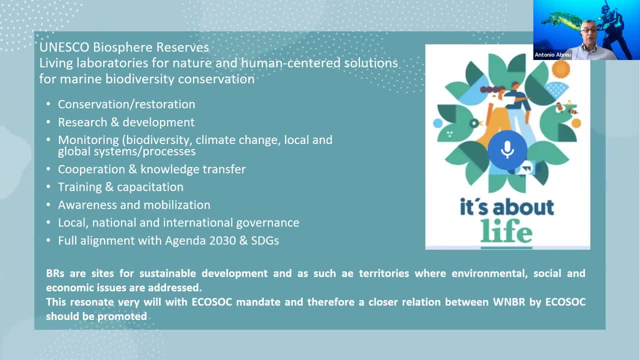 as living laboratories for nature and human-centered solutions by definition, and they can be used for marine biodiversity conservation and sustainable development. They provide initiatives and they have a mandate on conservation and restoration They need, then they do promote research and development. They are suitable sites for monitoring. 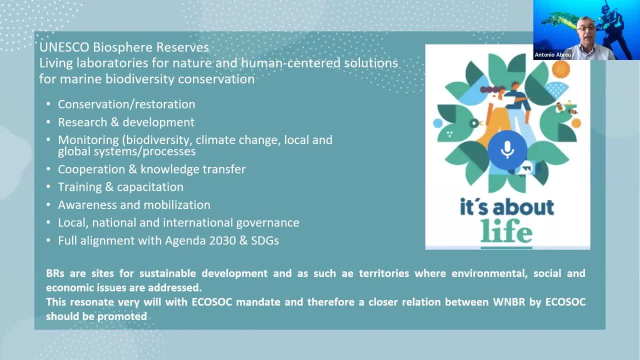 whether biodiversity or climate change or any other sector, including socioeconomic dynamics. They tend to work together and cooperate through networks, regional networks, thematic networks, so easy to promote. They also provide training and training to promote knowledge transfer. They ensure some training and capacitation. 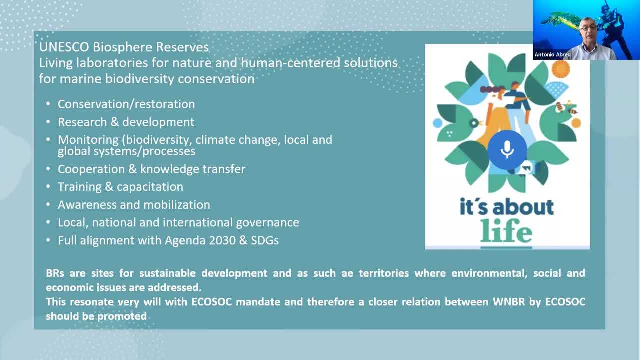 in different levels, as well as they promote a lot of awareness and mobilization, especially with schools. They ensure local, national and international governance which is suitable for ensuring a long or midterm initiatives, And they are fully in line with the agenda 2030. 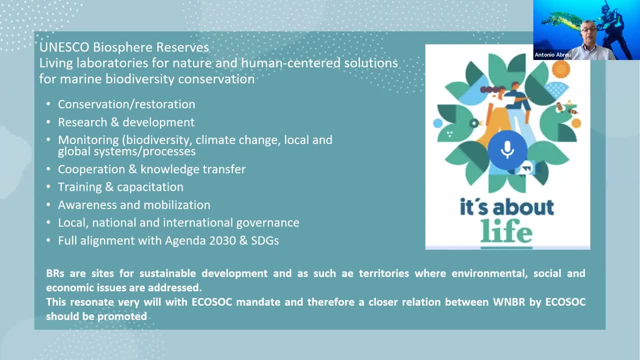 and the sustainable development goals, because the strategy that was approved in 2016, had that as a primary objective. In fact, what is missing here, it's communication and more availability of using the biosphere reserves as sites for sustainable development and benefiting from all the dynamics that exist. 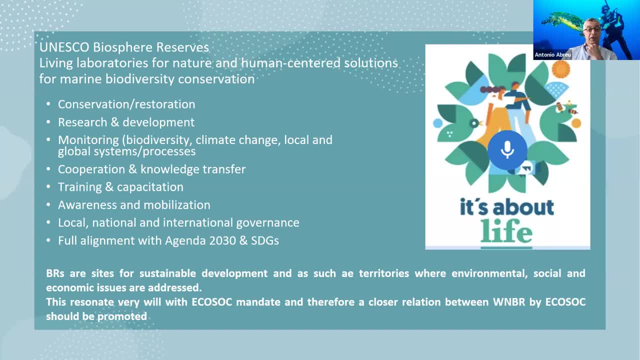 And I will mention. I am mentioning here ECOSOC, because the ECOSOC mandate is exactly in line with the biosphere reserves, but of course all other programs and agencies are strongly invited to explore and better link with the UNESCO man-handed biosphere reserves. 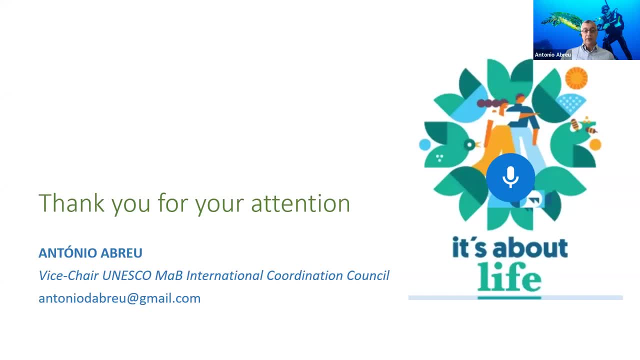 Thank you very much again for this opportunity And I hope that we can continue dialoguing and exchanging, Thank you. Thank you very much, Antonio, And thank you also for bringing in the connection between SDG 14 and SDG 15,. 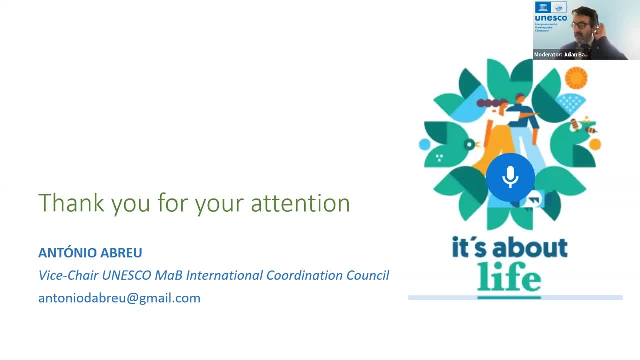 because also the whole work of marine biosphere is contributing to both. you know, for this kind of human centered approach, research driven management of ecosystem. And nice to hear some nice you know, some success stories and really how we can really concretely transfer. 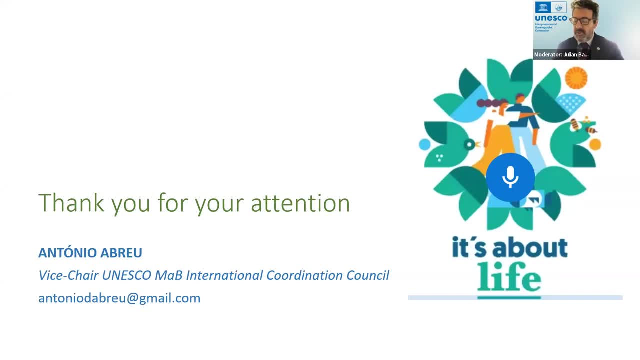 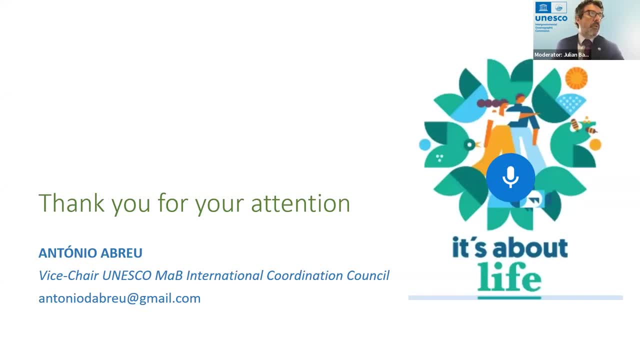 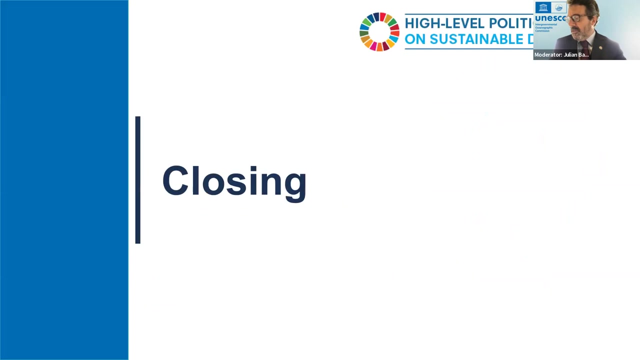 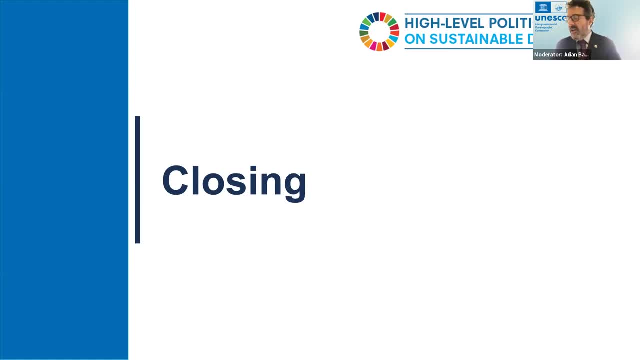 help with the implementation of sdg14. clearly, colleagues who are attending the high level policy forum can draw from this information and highlight some of the priorities we've heard about in terms of where we need to invest in terms of generating this kind of new type of ocean. 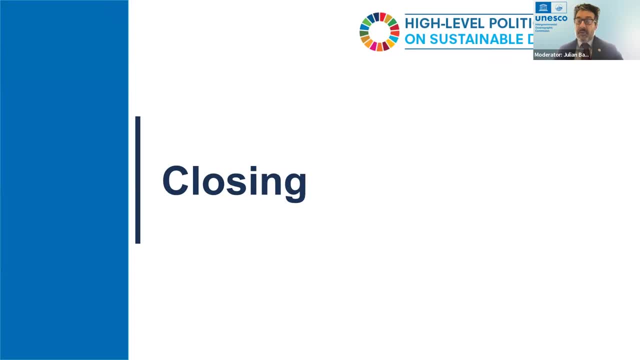 research and, of course, the ocean decade for ocean science for sustainable development is quite a unique framework to uh to collaborate and generate this transformative approach to science. we need better observations, uh, and we have innovation in those areas in all fronts, and i think that's um that that's good. but we need to integrate this uh to really get this global picture and holistic. 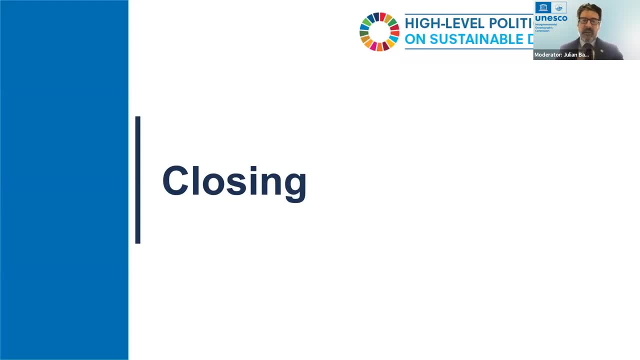 vision of how the the ocean is evolving in in real time and but also in terms of future. and then we need uh to apply this knowledge to support management. that that's really the the ambition of uh, of all we are doing here. uh is to have a you know, the right capacities and the right